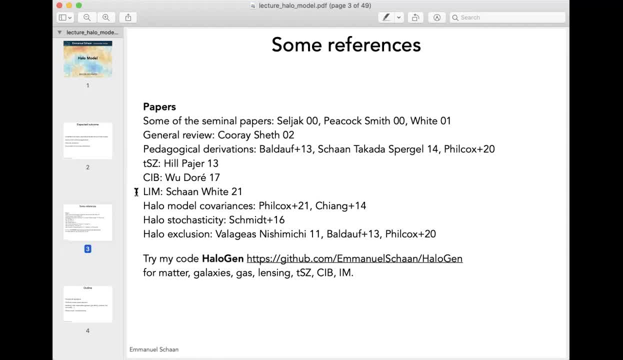 The cosmic infrared background and line intensity mapping, And again I'll say what those things are. Some other topics that I'll mention but won't go into in too much detail. There are sort of advanced topics, for the HILO model are here and I'm just listing some references in case anyone's interested. 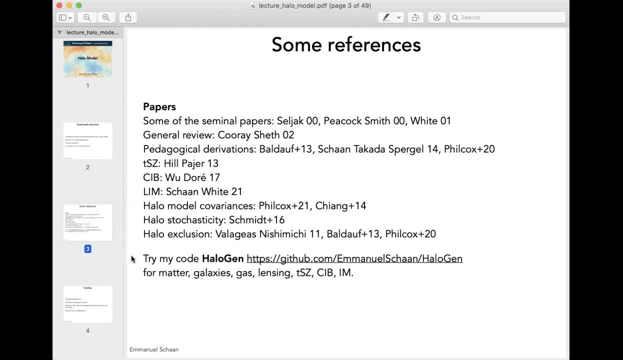 And something that might be useful is that pretty much everything I'm going to show today is implemented in this code, HILOGEN. This is a code that I've written and worked with in a number of papers, And so it's in this repository. if you want to go, take a look And that's. 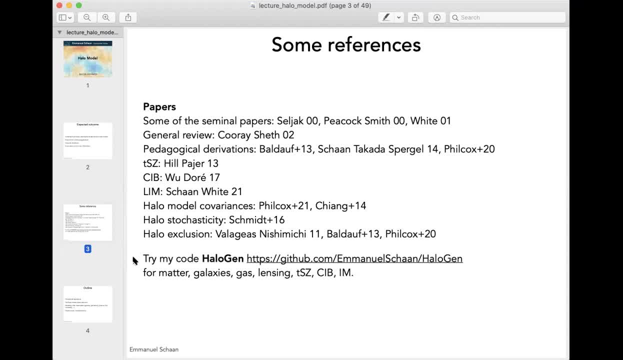 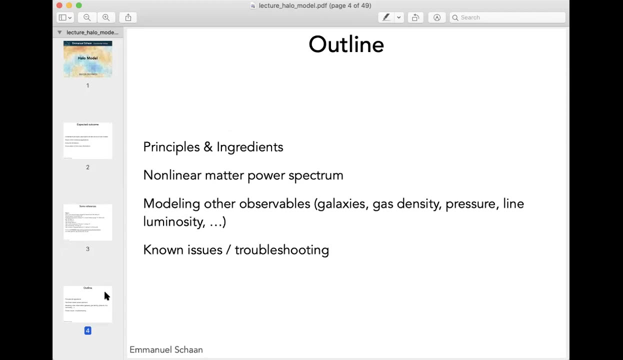 a very useful tool And it might be helpful if you ever need a HILO model for any of your research projects. feel free to use that one. Or if you're just interested in how to code up or some details of any of the ingredients, you'll find them in this code. So for the lecture today, I'll start. 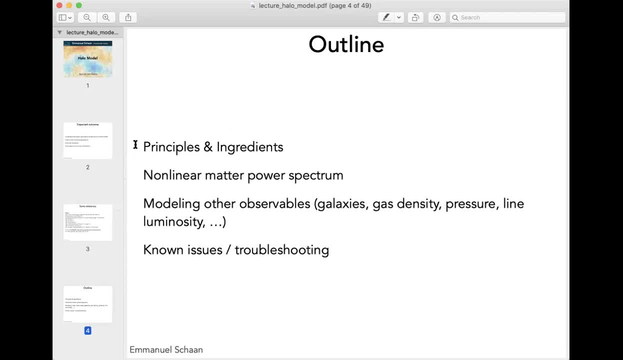 with explaining what this HILO model is, what are its goals, what are the principles, its assumptions and what are the ingredients that go into it. So that will be a big part. After that, I'll walk you through one derivation, which is how the HILO model can be used to derive. 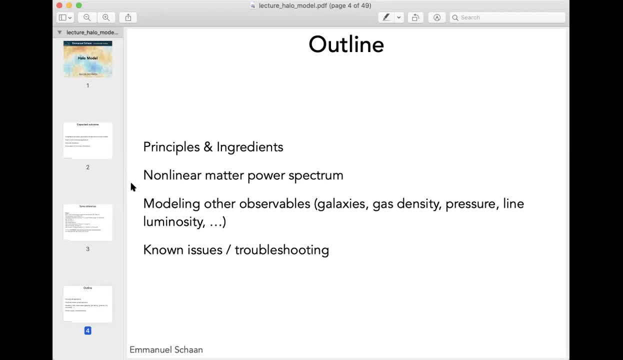 the nonlinear matter-of-power spectrum. And then I'll briefly list a number of other applications of the HILO models And these are things where I've actually been using the HILO model quite a bit. And finally I'll list some of the common issues with HILO models, some of the limitations. 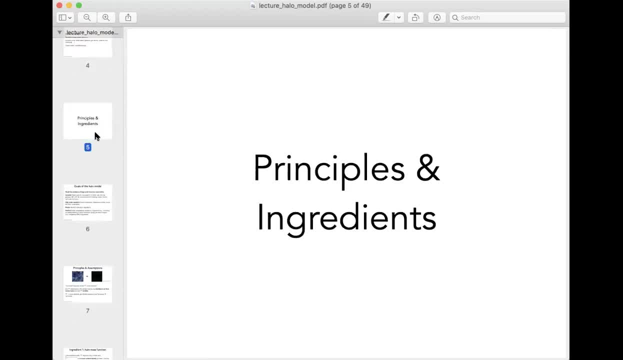 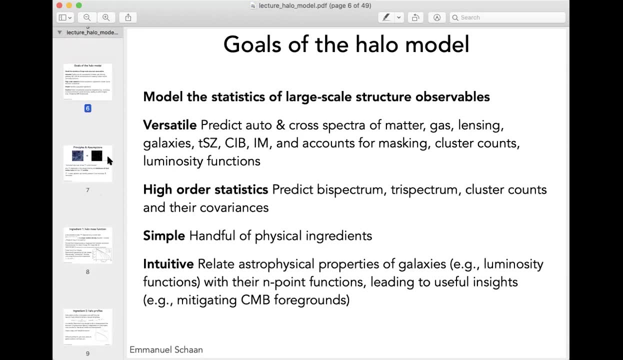 that I just talked about. So let's get started. What's the HILO model? What are we trying to do here? So there's a number of goals, Things we're trying to achieve with this HILO model, And the first one is basically in general. 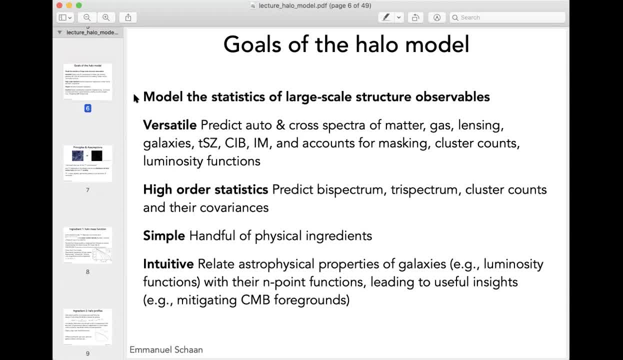 modeling the statistics of many large-scale structure observables, And so those observables might be things like galaxy clustering, matter clustering gas density pressure in the universe, things like lensing of galaxies or the cosmic microwave background thermal Sunyev-Zeldovich. 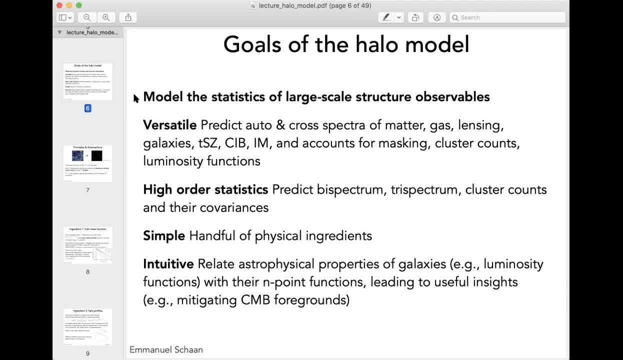 effect, which I mentioned- intensity mapping, et cetera- And that's actually one of the values of the HILO model- is that it's extremely versatile. So with this model, you can predict auto and cross-power spectra for many, many different observables, some of which I just listed. 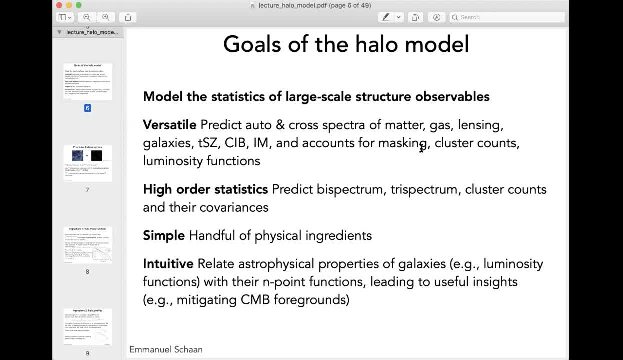 And this model lets you account for a number of realistic effects such as masking- But we'll see what that means later- And it lets you relate these quantities to other observables like cluster counts. So when you try to count how many galaxy clusters you find in a given survey, 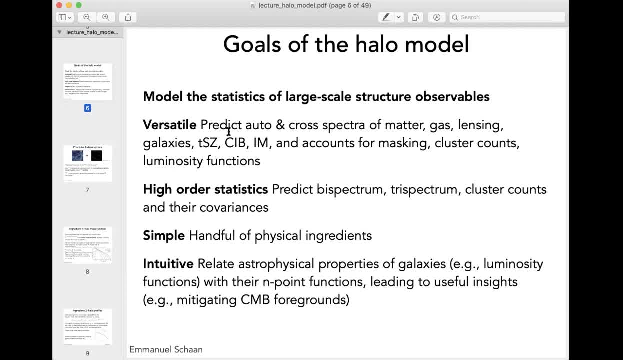 or things like galaxy luminosity function. So not only does it let you predict auto and cross-power spectra of these observables, it lets you relate them to those cluster counts and luminosity functions. Another value of the HILO model is that not only do you predict power spectra, but you can actually 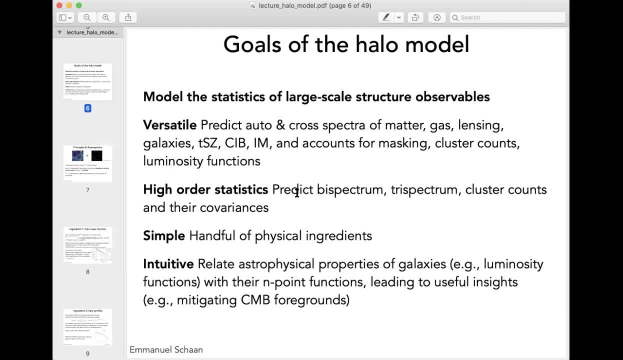 predict all sorts of higher-order statistics. So things like bispectrum, trispectrum, endpoint function with higher n, And this is useful in particular if you care about covariances between, for example, power spectra. Those covariances are useful if you're trying to combine different power spectra. 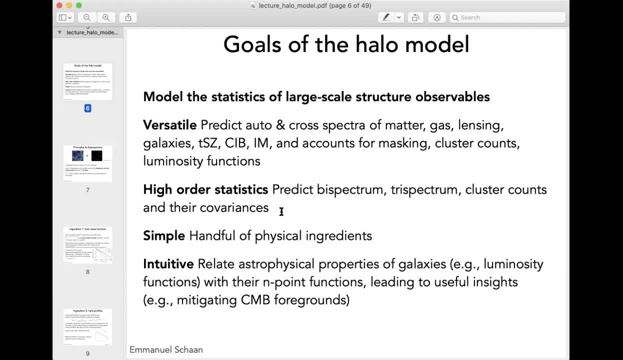 in a joint cosmological analysis. You need to know about the covariances. And finally, one of the key values of the HILO model is that it's very simple and intuitive, in the sense that there are only a few physical ingredients that go into. 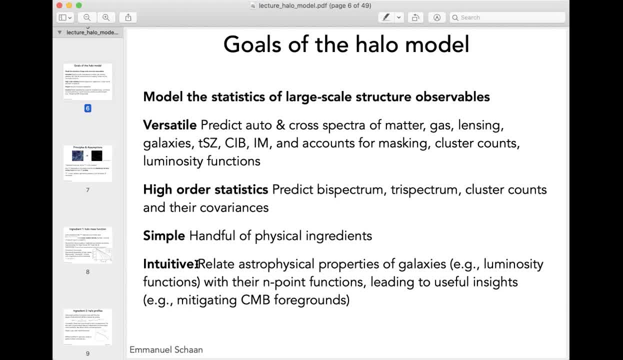 that model And it's intuitive because it lets you relate a lot of the astrophysical properties of galaxies to their statistics, like endpoint correlations. So these are the goals of the halo model and this is why I think, as a cosmologist, it's very useful to know about it. 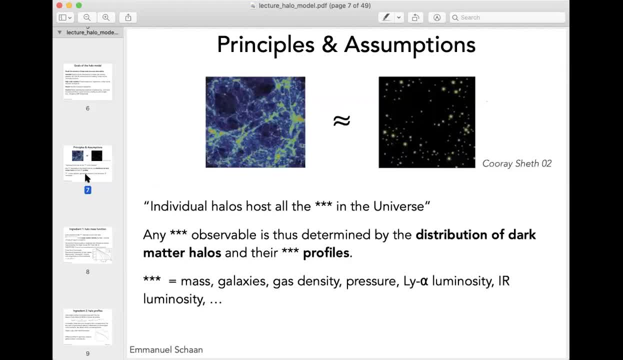 Going through the assumptions. in principle they're fairly simple, And the idea is that if you look at an n-body simulation of dark matter in the universe, you might find that what you see looks kind of similar to a set of dots where all the mass would be concentrated. 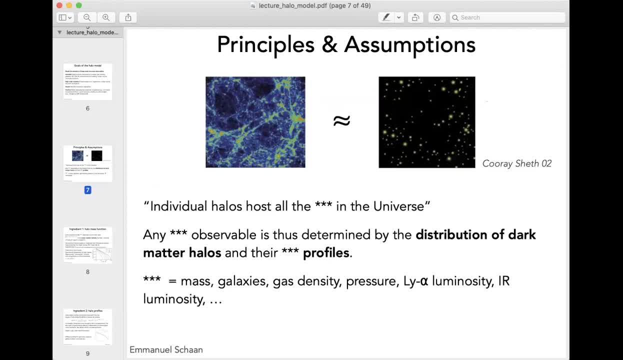 and these are called dark matter halos, And a halo model is going to be useful for you every time that individual halos host all of the quantity you care about in the universe. And again, that quantity observable can be mass, galaxies, gas density, pressure, etc. 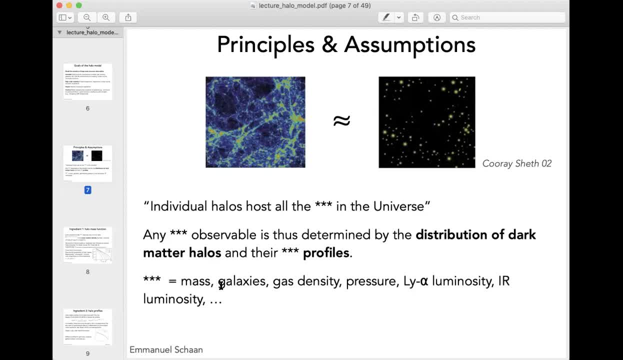 So, for example, if you care about the clustering of galaxies, the halo model is going to assume that individual halos host all of the galaxies in the universe And, as a result, any observable or statistics of the quantity you care about- maybe galaxies- 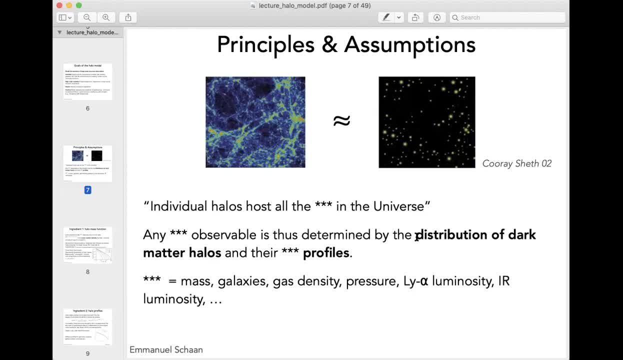 is determined mostly by two things: One, the distribution of dark matter halos, And here that means how many halos there are where they are, And two, what are their profiles in terms of the observable you care about. For example, in a given dark matter halo, how are the galaxies distributed? 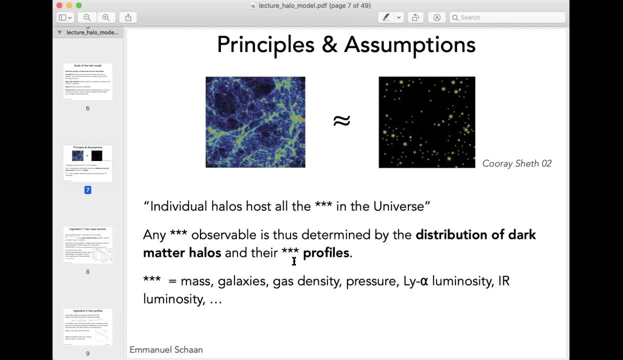 How spread out are they? So that's the key assumption of the halo model is that, hopefully, the quantity you care about is made of objects that only live inside of halos, And therefore, to predict their statistics, all you need to know is where are the halos and what are their profiles. 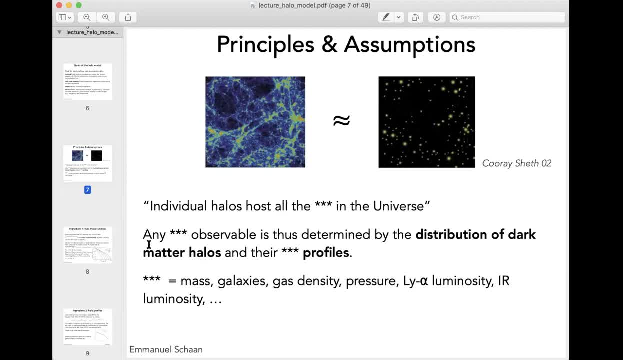 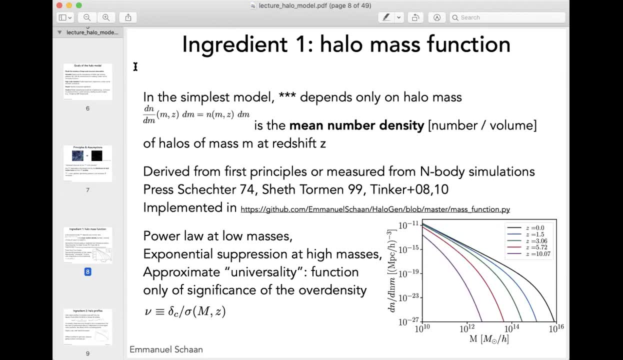 So let's now go into those ingredients about where are the halos, what are their profiles, and start ingredient number one, the halo mass distribution function, And this basically answers the question of how many halos are there of a given mass And in the simplest halo models, 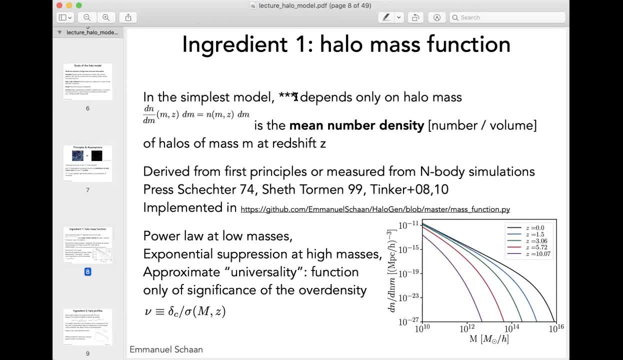 your observable is related to the halo only through mass. That's the simplest model. In practice, things like the number of galaxies may depend on other things than halo mass, But that's the first step, the first approximation, And to do this we then describe the number. 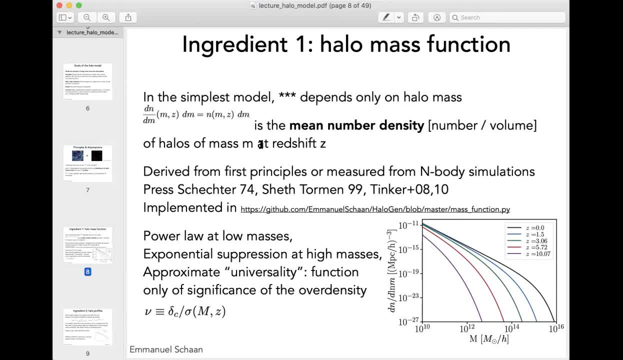 the mean number, density of halos of a given mass at a given redshift by this quantity called the halo mass function dn, dm, which I'll write- and it's often written n of m, So n of m. dm is the mean number, density of halos of mass m and redshifts. 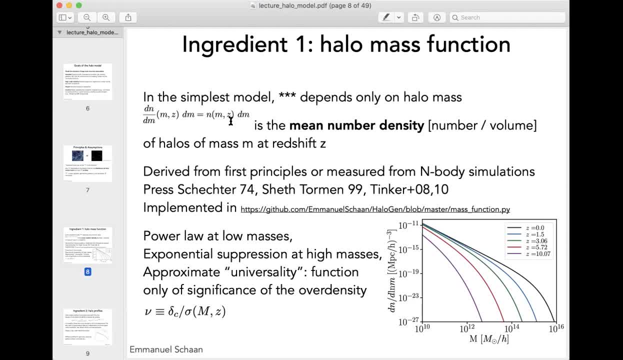 So that's a key ingredient in the halo model, the halo mass function, And there are various ways to predict it or to estimate it. There's a very interesting first principle calculation for what the halo mass function should be, And an example includes the press checklist. 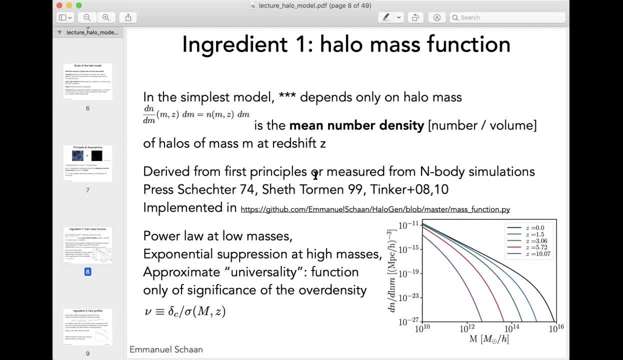 So the mass function is a vector mass function, and then other fitting functions have been derived by looking at n-body simulations, And so these might be the Scheff and Tormann or the Tinker mass function, And so these names are names that you'll hear all the time when people talk about halo model. 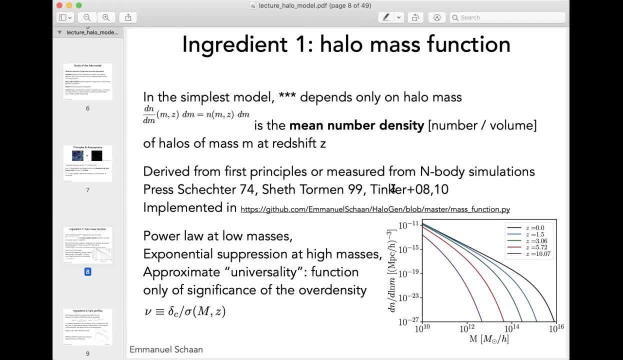 People might be using the Press-Schechter mass function, the Scheff-Tormann mass function or the Tinker mass function And if you ever need any of them again, they're implemented in this code, in this code halogen that I talked about. 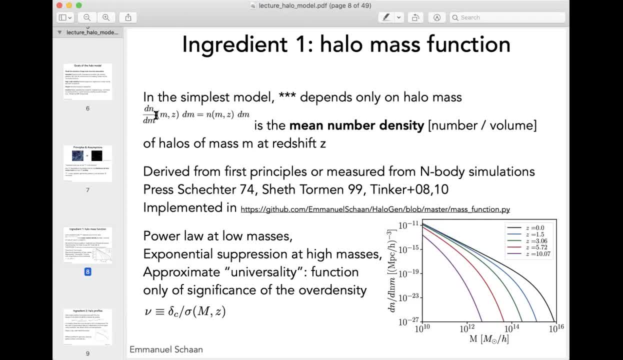 So now, if you ask: how does this work? what does this mass function look like in practice? I've plotted it here as a function of mass, And so each line is a different redshift. So if you start at redshift 0, that's the black line. 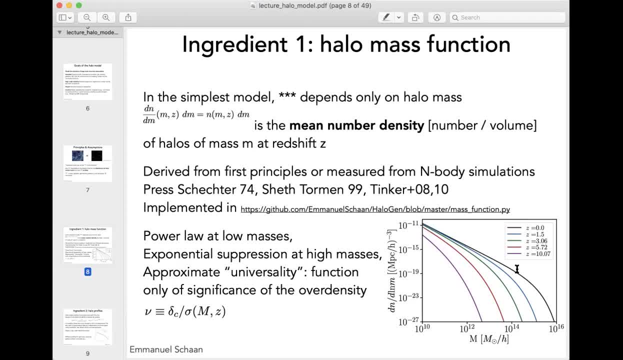 the features you see in this halo mass function are a power low at low mass and then an exponential suppression at high masses, And this is basically what you'll find in any halo mass function: fitting function, And then, as you go along, as you increase in redshift. 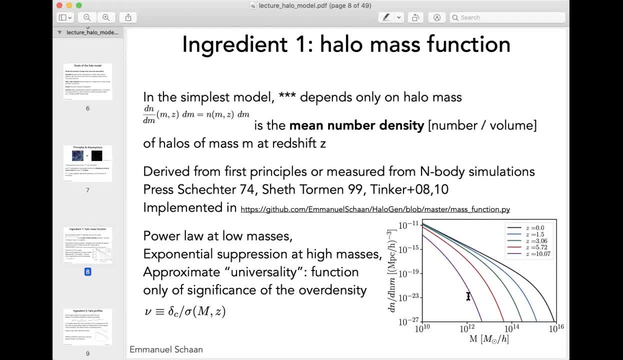 you see that the curve goes down because as you go to higher redshift you go back in time. fewer halos have had time to form and, in particular, fewer massive halos. So that's the typical shape of a halo mass function. 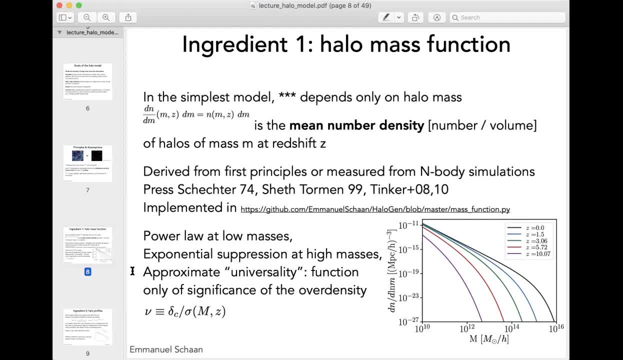 And you might hear of something called universality, which is the fact that the halo mass function can often approximately be written as a function not directly of mass and redshift, but of the significance of the over density. So at a given redshift and for a given halo mass, 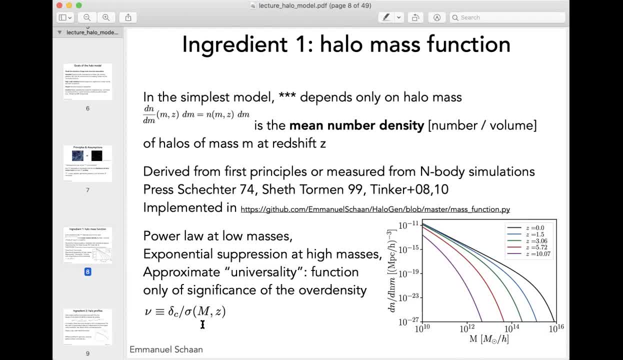 you can ask what's the variance of the matter density field on the scale defined by the mass and ask how that compares to a fixed threshold from spherical collapse. So that's a little bit of a detail, but I just wanted you to have heard of this word of universality. 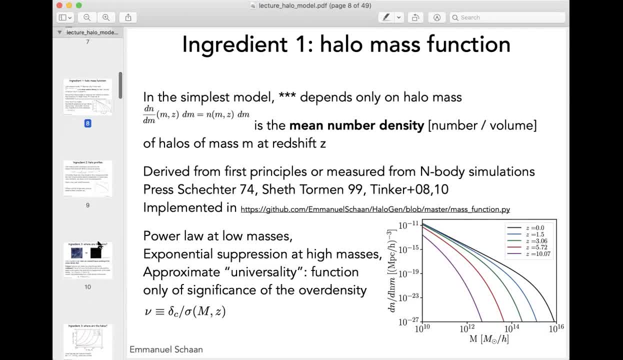 of the halo mass function. Okay, So that was ingredient number one. I'm going to move to ingredient number two And, again, at any time, feel free to interrupt if there's anything that's unclear, Since we're in a small group. 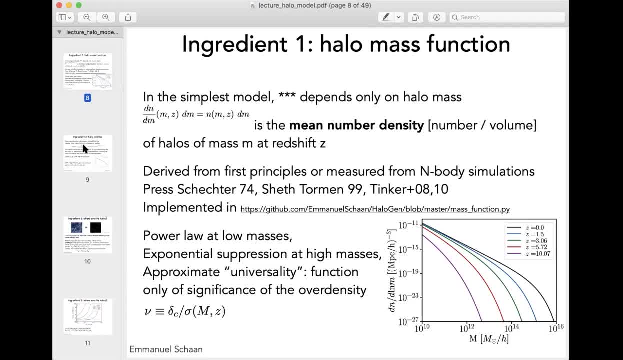 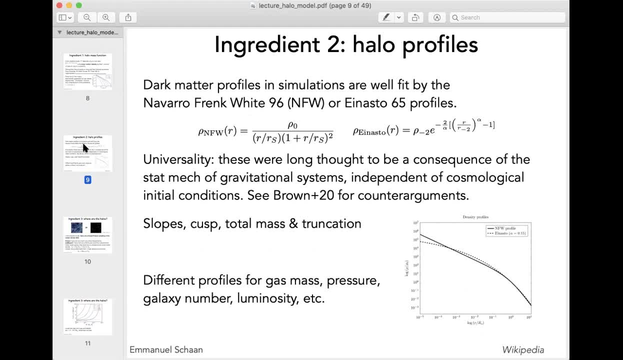 this is perfect for doing this. So, moving on to ingredient number two: halo profiles. So we know how many halos of each mass there are. That's the halo mass function. Now I would like to know how is the mass distributed within a halo? 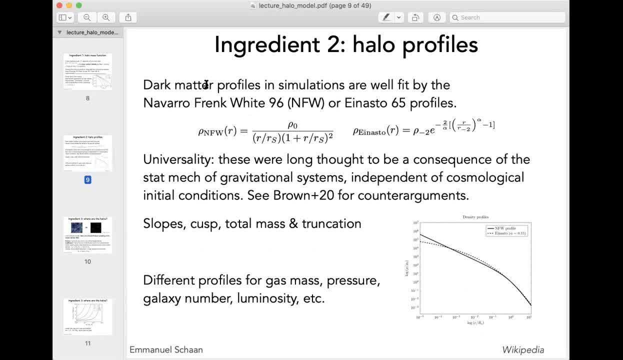 And these are the halo profiles It turns out, if you look at dark matter simulations, so n-body simulations, what you find is that the density profile of halos are well fit by some of these fitting functions: the NFW or Navarro-Frank-Wein fitting function. 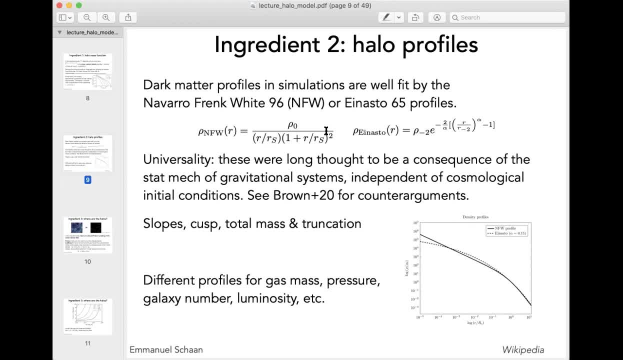 and the I-Nasto profile. So I've written their expressions here And the one that I think is most commonly used is this NFW profile. So it's characterized by one free amplitude and one scale for the radius And you can see that the scale dependence. 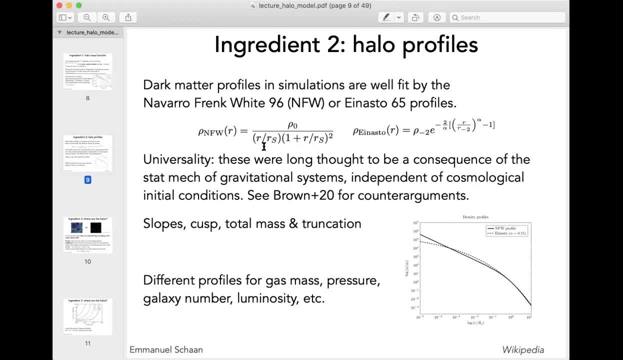 as a function of radius. R is basically a broken parallel. So when the radius is small and this quantity is basically one, you see that the profile goes down as one over R. But instead, when you're at large radii and R over the scale, radius is much larger than one. 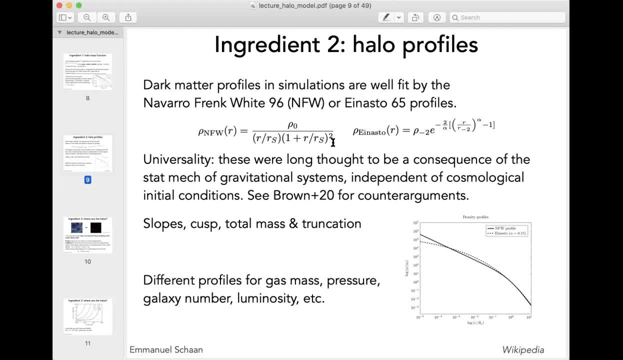 you find that the scale dependence of the profile is more like R cubed, So NFW profile, broken parallel, one over R and one over R cubed. And this is what is shown on this plot: one over R and then one over R cubed. 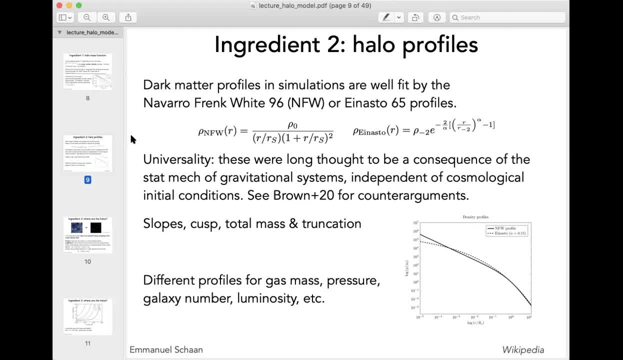 Something that's somewhat intriguing about these profiles is that it's again an issue of universality, but here a slightly different meaning. This is sort of an unsolved problem, but there's this idea that those NFW profiles would naturally arise from the stat mech of gravitational systems. 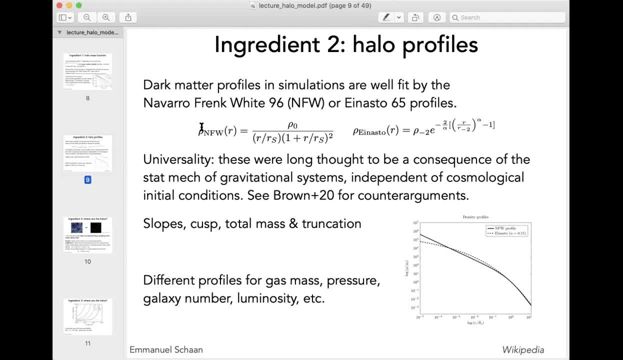 Meaning that all halos would sort of look like this, regardless of the initial conditions of the universe, just because of how gravity clumps things together. And this is sort of a longstanding open question, And I thought I would just mention it so that you've heard of it. 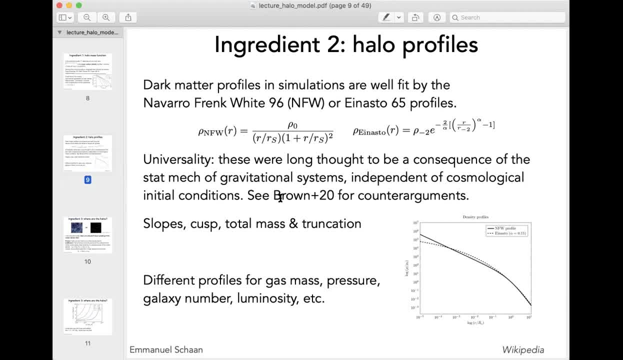 And if you're interested in counter arguments to this, you can look at this paper. So I described the two slopes of that broken parallel for NFW: one over R, one over R, cubed. One thing that you might think, one thing that you might hear about. 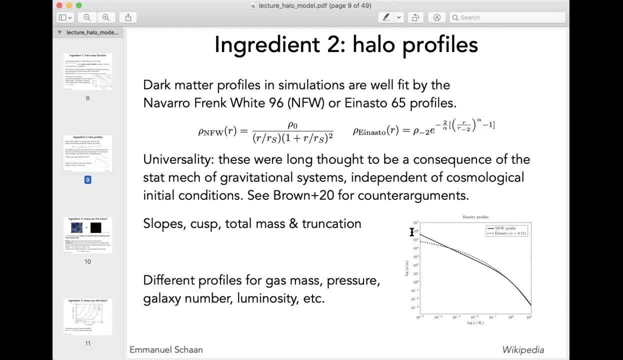 is this concept of cusp, The fact that the matter density at zero radius is infinite. So there's this peak in density, And another thing I should draw your attention to is the fact that since at large radii this profile goes down as one over R cubed. 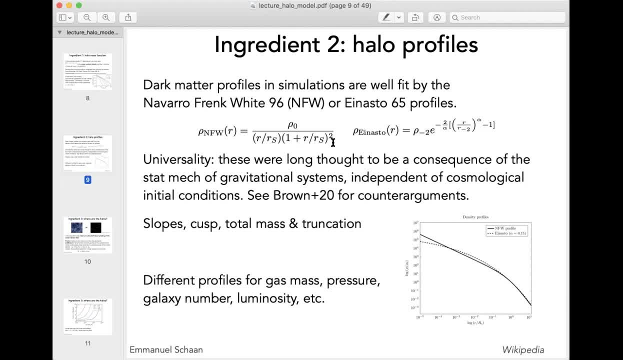 If you integrate over radius to get the total mass within that profile, you find something infinite. So that's somewhat unfortunate that this fitting function gives you an infinite profile And it's related to the fact that this profile has been measured in simulation just out to some radius. 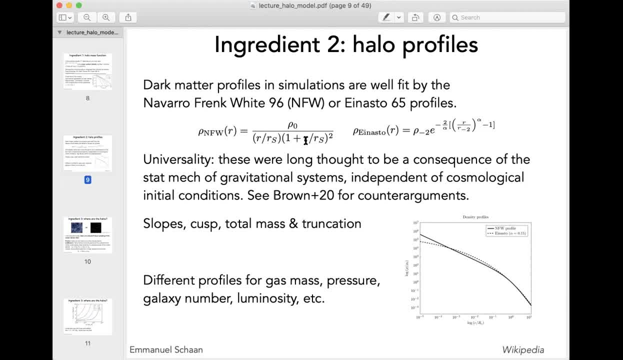 And so this profile is typically truncated when using the HILO model, meaning past a certain radius, people just set it to zero, So that's good to keep in mind, And here I talked only about dark matter density profiles. but really in your HILO models, 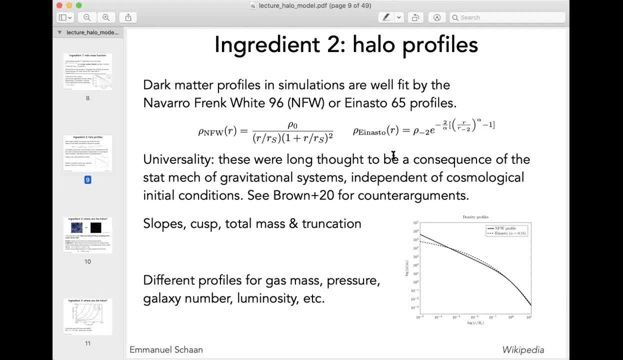 you'll need the HILO profile for whatever quantity you're interested in. So if you're interested in predicting instead the clustering of galaxies, what you'll need is the galaxy profile. If you care about the gas mass, you'll need the gas mass profile of the HILOs, and so on. 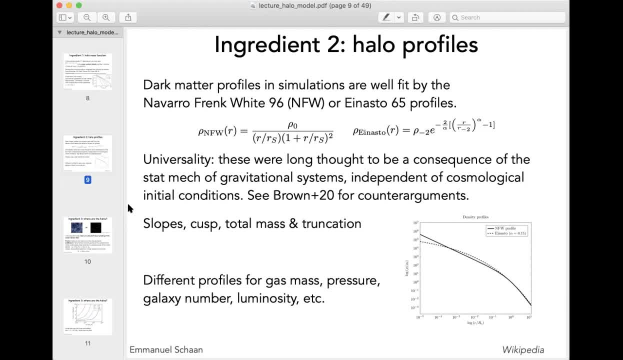 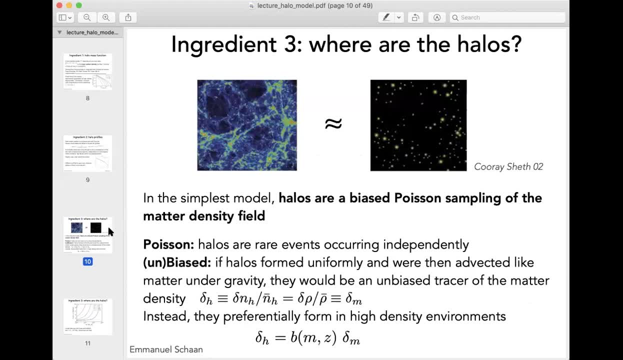 Okay, so now we know how many HILOs of each mass there are. We know what their profiles look like. The last thing we need to know is where are these HILOs located? How clustered are they? And, of course, if you look at those two pictures, 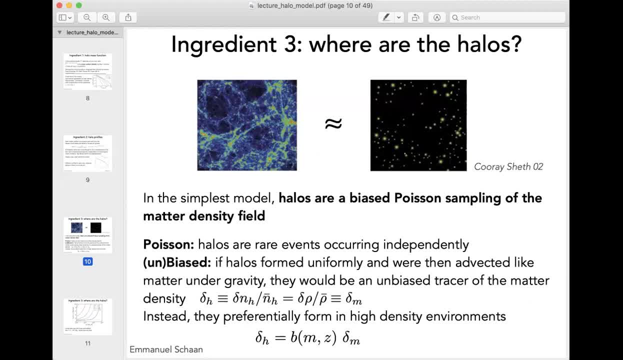 what you see is that those dots, these individual HILOs on the right-hand side, sort of trace the over densities you see in the n-body simulation, And so in the very simplest HILO model we typically assume that HILOs are biased Poisson sampling. 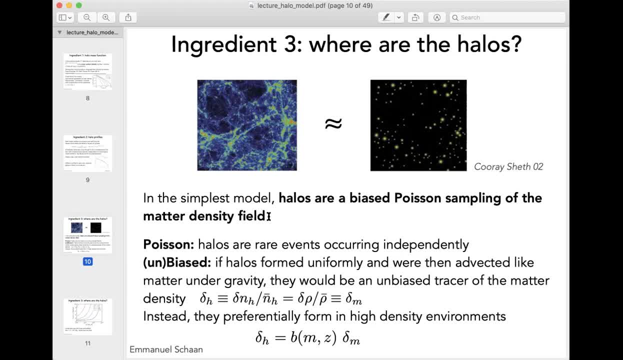 of the matter density field. So let me break this down. They are a biased tracer of the matter density field, and I'll say what that means in a moment. And they are a Poisson sampling, And I'll explain what that means. 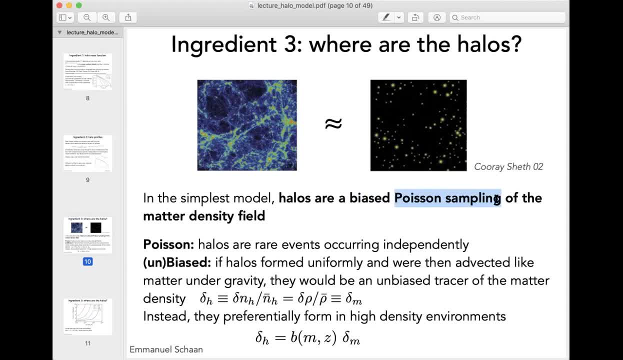 But so basically, this assumption of Poisson sampling means that where you have more density, matter density you'll have more HILOs, And exactly how many HILOs you'll have is a Poisson random variable And that Poisson distribution is appropriate. 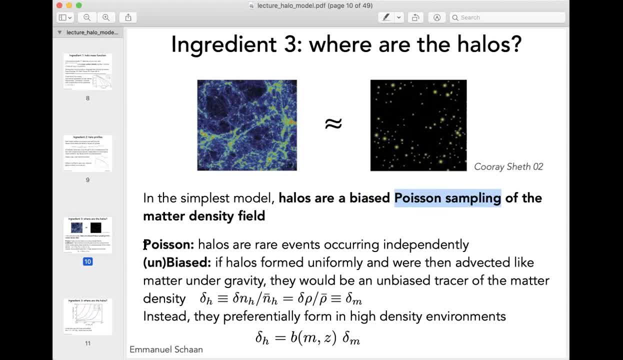 every time you have independent rare events. So when we assume a Poisson sampling we assume that HILOs are rare events that occur independently. meaning if I happen to have a fluctuation of one or more HILOs here, that does not influence whether or not. 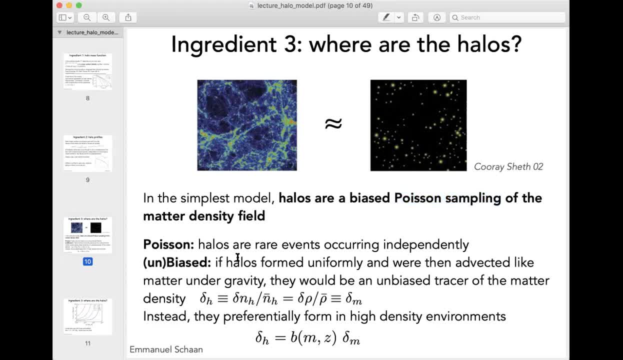 I will have more there. So that's the Poisson part, And then the biased part means the following: If HILOs had formed uniformly in the initial conditions in the universe and then were just advected under gravity, just like the matter is, 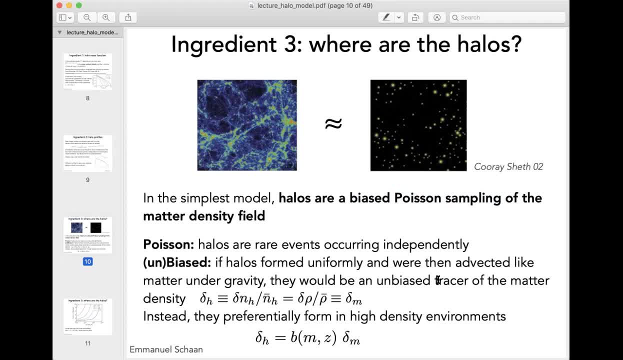 what you would find is that HILOs would be an unbiased tracer of the matter density, And what that means is that the HILO number over density, which is the ratio of the variation in the number of HILO over the mean, would be equal to the matter over density. 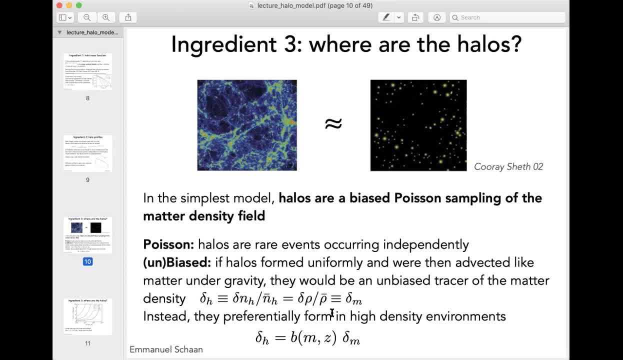 So delta HILO- the HILO number over density equals delta matter, the matter over density. That's the definition of what we call an unbiased tracer. The over density in HILO is exactly equal to the over density in matter. But in reality this is not the case. 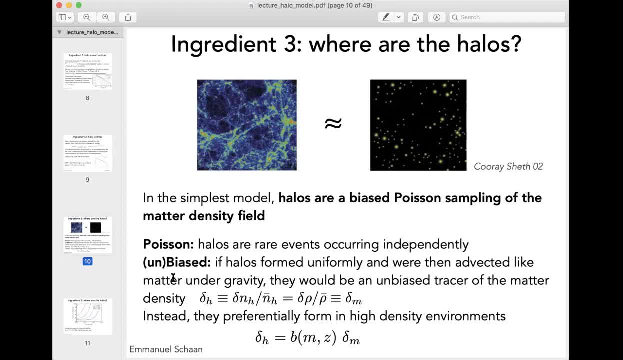 The HILOs don't just form uniformly, randomly, in the initial conditions. They form only in the high density environments in the initial conditions And, as a result, the HILOs are actually more clustered than the matter, And this can be encoded to lowest order. 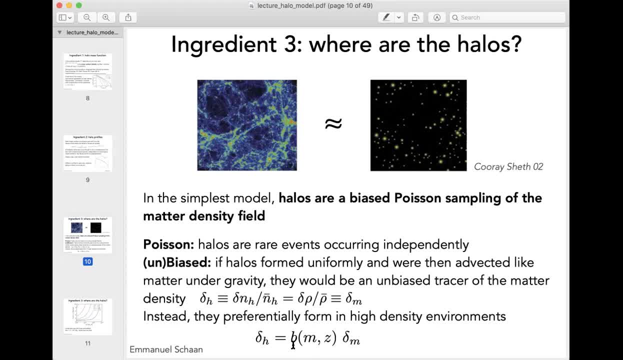 by this bias coefficient. So this bias, which depends on the mass and the redshift of the HILO and relates the matter over density to the HILO number over density determines how clustered the HILOs are compared to the matter. If the bias is equal to 0, it means delta HILO is 0. 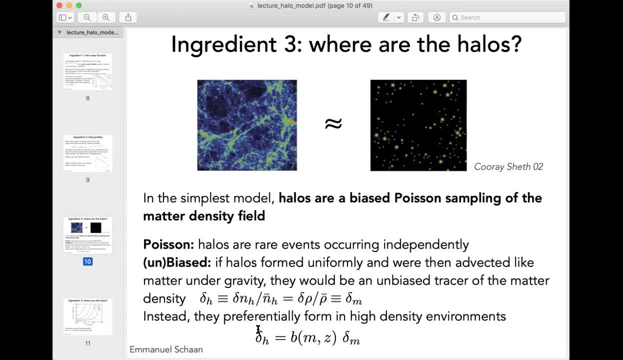 There is no fluctuation in the HILO density. The HILOs are perfectly uniformly distributed, So this never happens. If the bias was 1, it means the fluctuation in the HILO number density are the same as the fluctuation in matter over density. 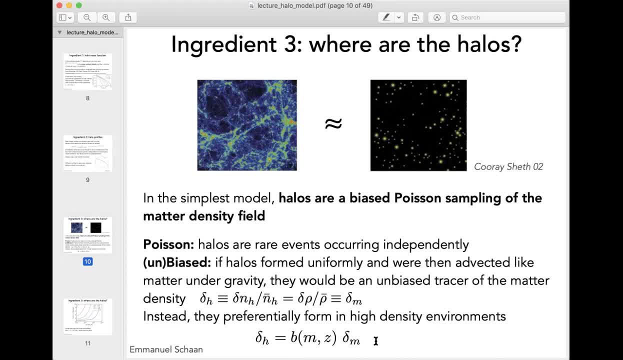 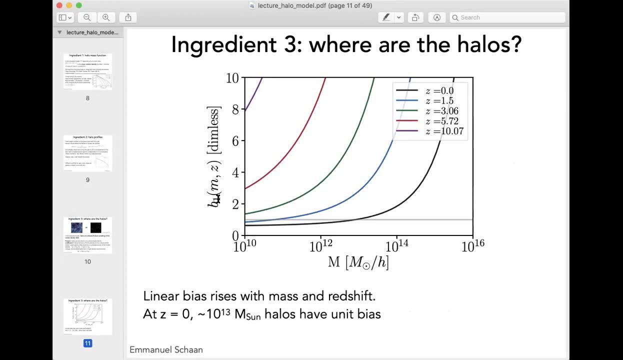 And that's why we would call an unbiased tracer of the mass. And in reality, depending on the mass, this bias can take a number of different values, And this is what I'm going to show you right now. So here, b1, or same as before, this linear bias. 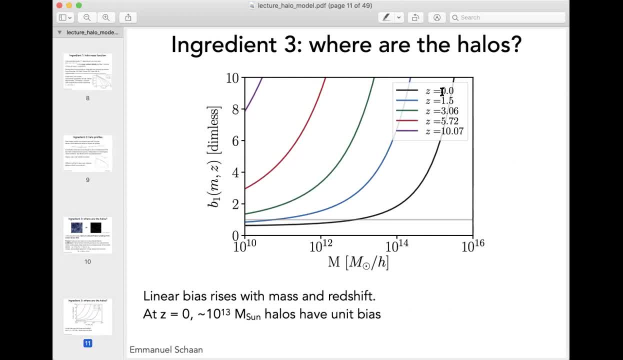 I have plotted as a function of mass for different redshifts. And so again, if you look at the black line at redshift 0, what you find is that the bias is equal to 1.. And so some of the HILOs are unbiased tracer. 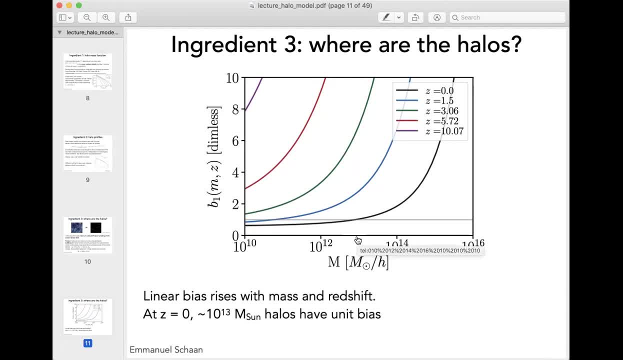 of the mass for HILOs of about 10 to the 13 solar mass. Then if you look at more massive HILOs, the bias is larger than 1, meaning those HILOs are more clustered than the mass because they formed in overdense region. 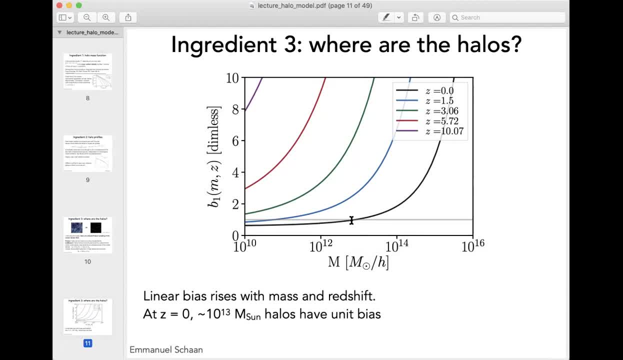 And if you look at lower mass HILOs, their bias is less than 1, meaning they are less clustered than the matter density field. So that's this question of linear bias, And again feel free to interrupt or ask any question you have on this. 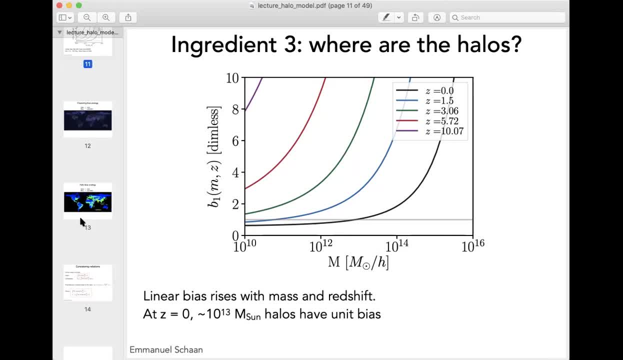 So I guess how good of an approximation is that the bias should only depend on the mass of the HILO And then also NFW, two free parameters there. The simplest model, I guess, does also just depend on the mass, or in reality, 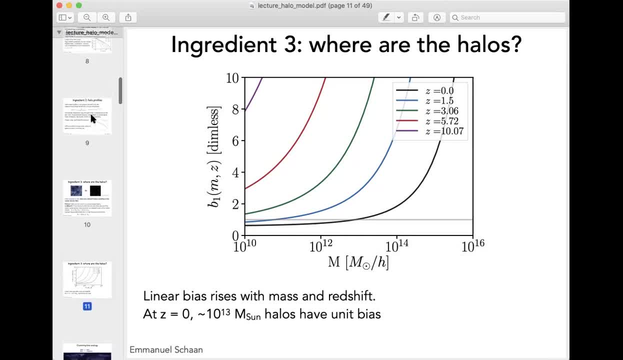 how good of an approximation is that Right? So that's a good question. So maybe I'll start with the question about the bias and the assumption that it depends only on mass, And I should say here we're making a bit more than this assumption. 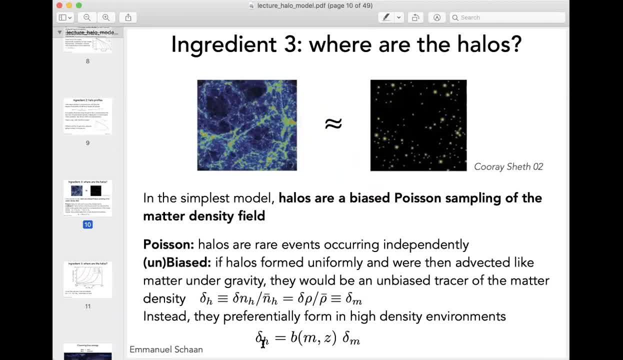 We are here assuming linear bias, meaning that the HILO density is linear in the matter density, As you know, you can go to high order in the matter density. So that's one limitation of this model. Another one, like you say, is: we assume 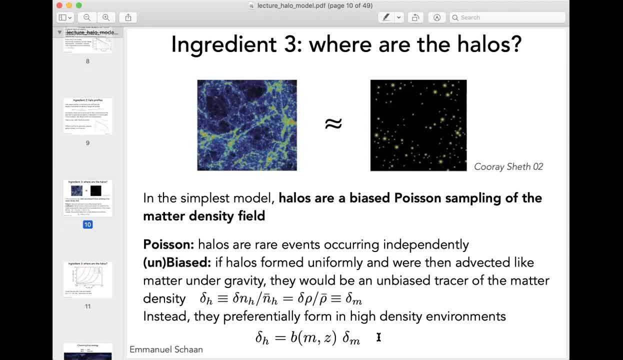 this depends only on mass And we are currently looking at extensions of this in actual data And these things going beyond the mass dependence is often called assembly bias, And the reason it's called this way it's because the idea would be that 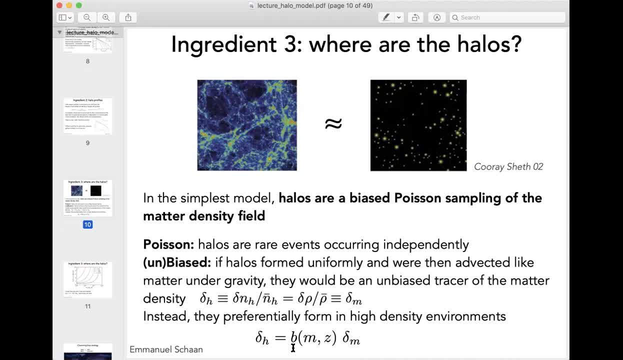 the bias of a HILO doesn't depend only on the mass but on some details of how it formed, And in practice you can get handles on this with things like HILO concentration. So if you look at a HILO and you look at its profile, 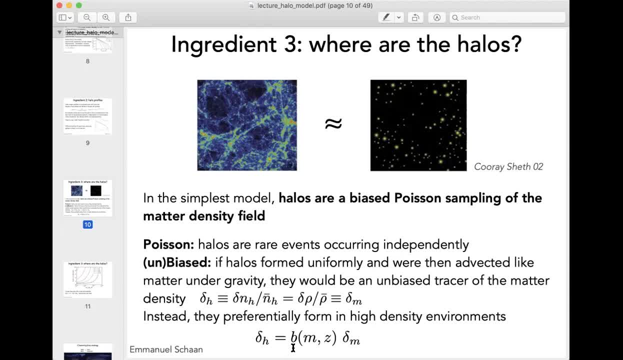 for HILOs of a given mass, you may have variance in the profile And this can be a clue as to how the HILO formed, And so that relates a bit this dependence of the bias on more than mass and this question. 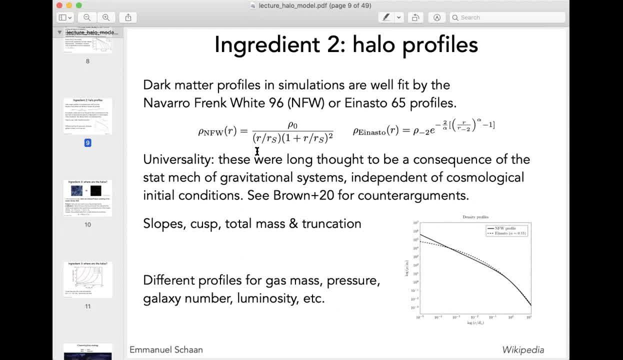 of this profile. So in the NSW profile we typically assume that these quantities- rho, naught and the scale radius- are functions of mass. But again, in practice they may depend on other quantities And going beyond just the mass dependence is sort of an open problem right now. 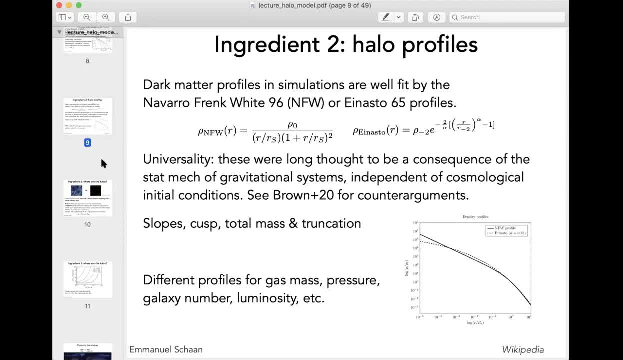 But one thing: we may have the sensitivity to detecting current data, So that's a good thing to keep thinking about. Is there a straightforward elliptical generalization of NSW? That looks very cool. Elliptical you mean taking into account the triaxiality. 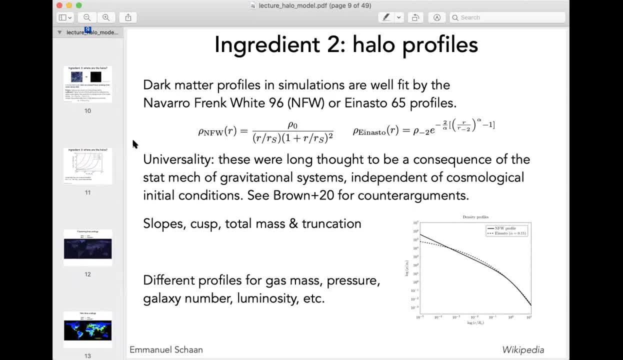 Right. I mean, the simplest thing you can do is always rescaling along each axis. For the things that we're going to talk about today, this spherical approximation is good enough, But then, of course, you can go beyond, All right. 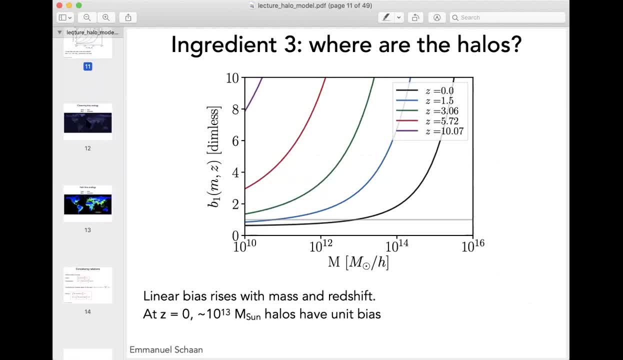 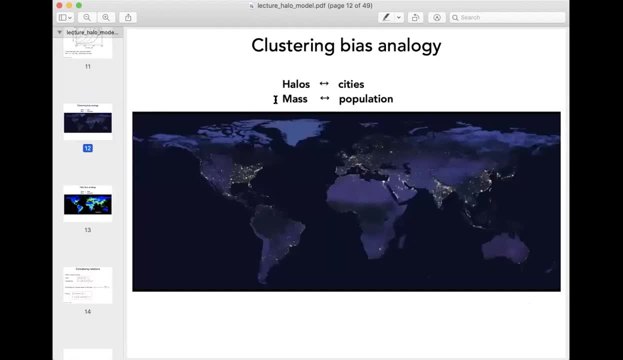 And then just to finish with one quick analogy with this question of what bias means, something I like to think about is this analogy where the mass in the universe is like the population on Earth And the individual halos are like cities, And that's just an image that can be helpful for thinking. 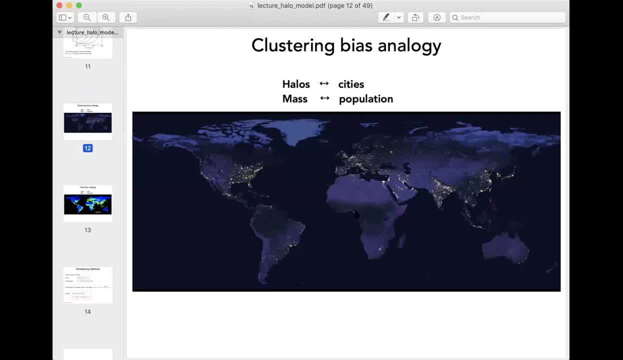 about these things. So if you look at what the Earth looks like at night, you might see those individual bright dots And these really tell you about cities, But in construction they're not. So in this small g you typically don't care about individual galaxies or halos. 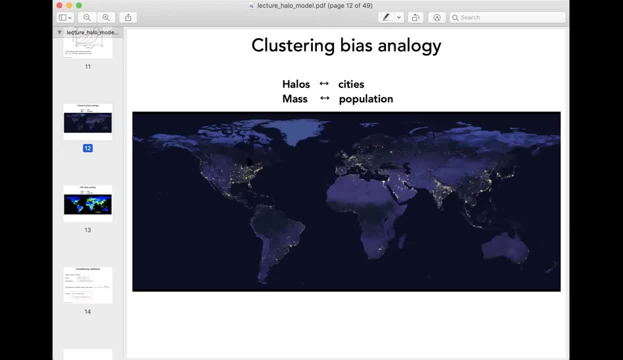 You want to know about the mass distribution. Here the analogy would be: you may be an alien who would like to know where humans are on Earth, And so what you may care about is population and ask: how can I learn about where people are? 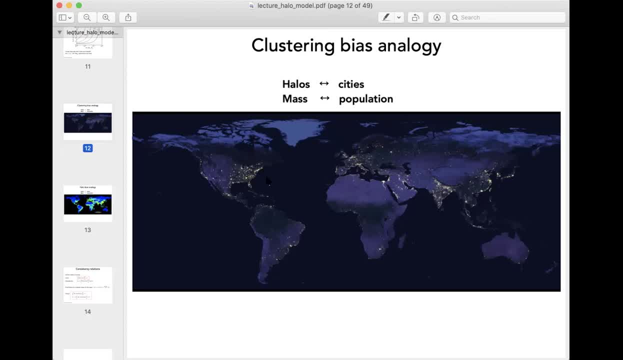 And so your first guess might be to say: well, where there are more cities, surely there are more people. And if you look at actually where the people are and you flip between these two, you'll find that it's a pretty good approximation where you have. 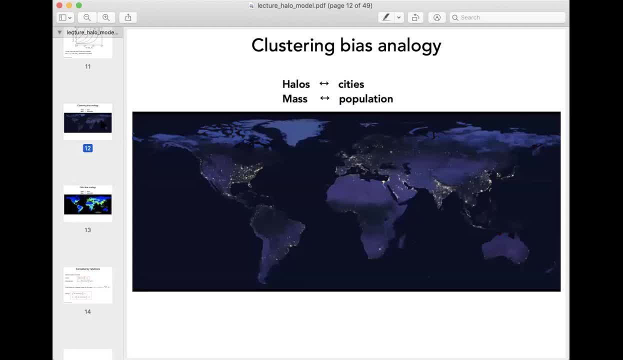 more cities or more halos, You have more mass or more people. And then you can also see limitations of this approximation, the fact that in some places you may have not many cities but a lot of population, And that's saying that cities are. 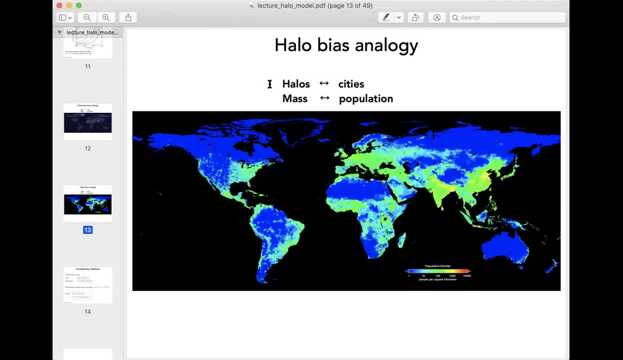 a biased tracer of the population, just like halos are a biased tracer of the mass. OK, so that's all I wanted to say about halo bias. So just to reiterate: we talked about how many halos there are as a function of mass and redshift. 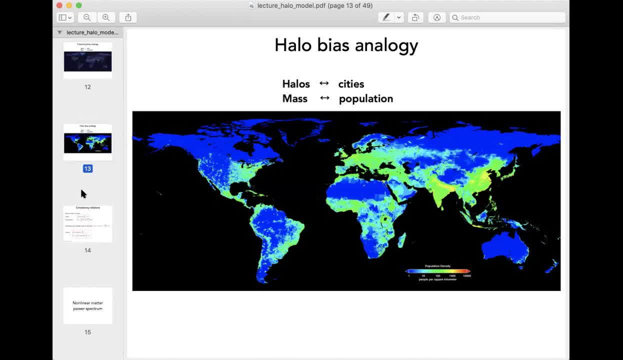 We talked about their profiles, how big those halos are, And now we just talked about where they are, how the visual halos trace the matter over density, And before combining all these ingredients to predict some statistics, I just wanted to mention those consistency relations. 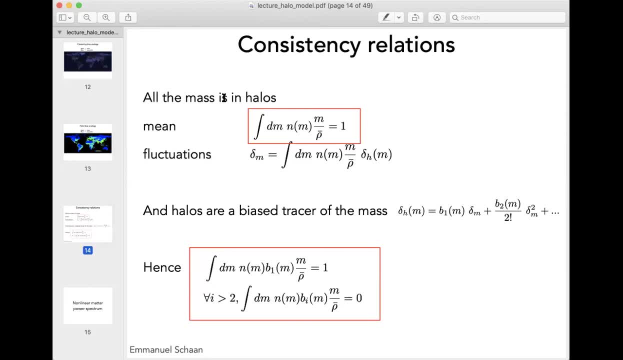 between these ingredients. And again, as I mentioned earlier, the key assumption of the halo model is that all the mass is inside of halos And in terms of mean density of the universe you can translate into this constraint. So if you forget about rho bar here, 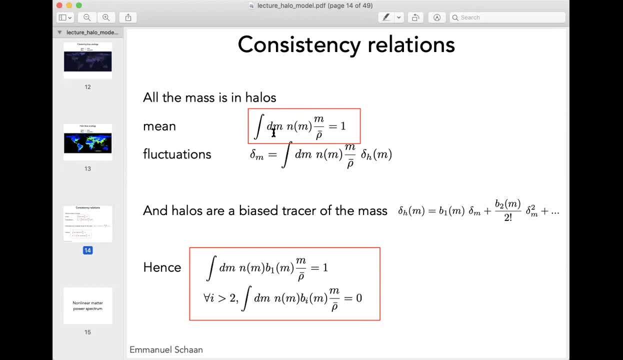 this integral tells me: dm n of m is how many halos I have of mass m per unit volume times their mass. So I have number density of halos times their mass. That's the mass density, And that quantity should be equal to rho bar. 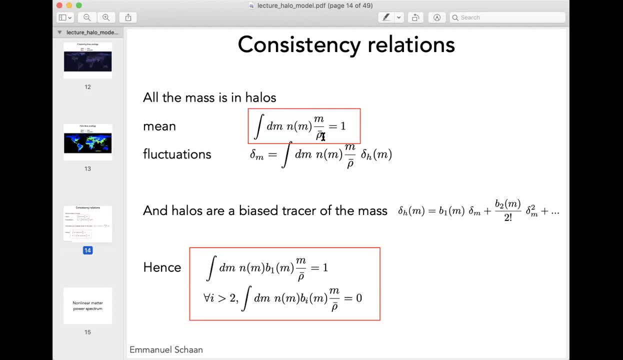 the mean matter, density in the universe. So if you divide by rho bar, you get this integral that should be equal to u bar And that's the first consistency relation on your halo model is that, if you want that all the mass is inside of halos. 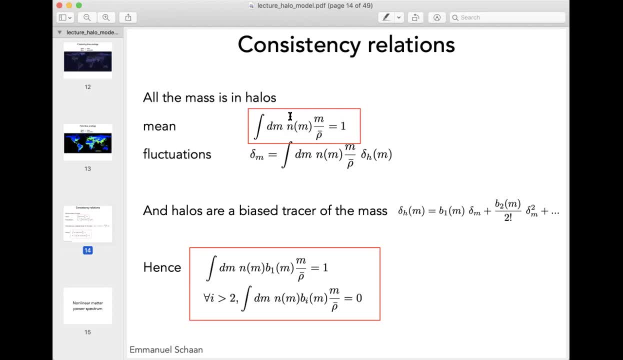 you need your halo mass function to be normalized in this way. The next consistency relations come from the fact that, again, we've assumed all the mass is inside halos And so, in particular, the mass over density field can be determined if you know the halo over density. 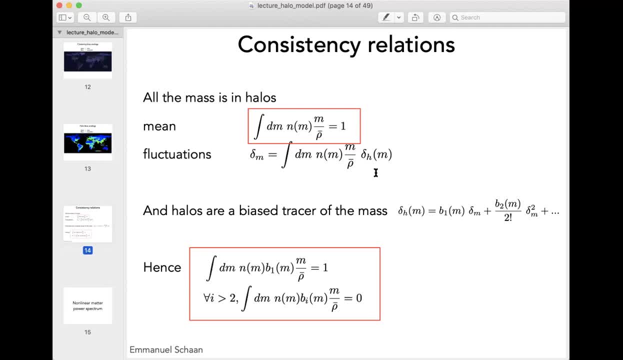 Simply by saying: if you weight all of your halos of mass m by their mass and by how many there are, you should recover the total matter density field. But here you have related the matter density field to the halo number density field. But as we said, this quantity is also related. 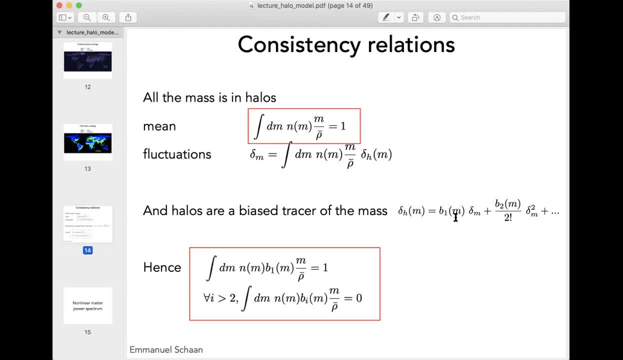 to the matter density field through the bias, And so we talked about this linear bias model And if you want, you can also go to higher order. But if you keep only this linear bias model and you plug this into here, you find that delta matter. 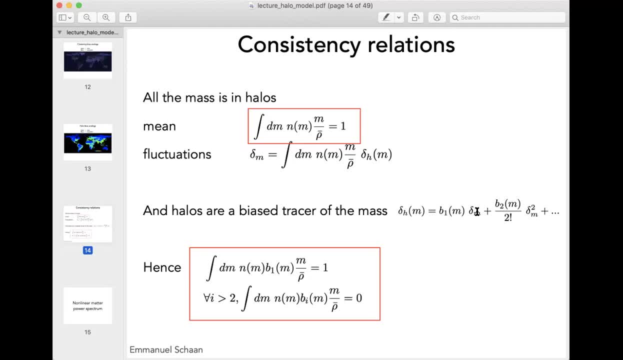 is equal to some integral of b1 times delta matter, And so that whole integral has to be equal to 1.. And this is this integral. So, again in your halo model, if you want all the mass to be inside of halos, what you need, 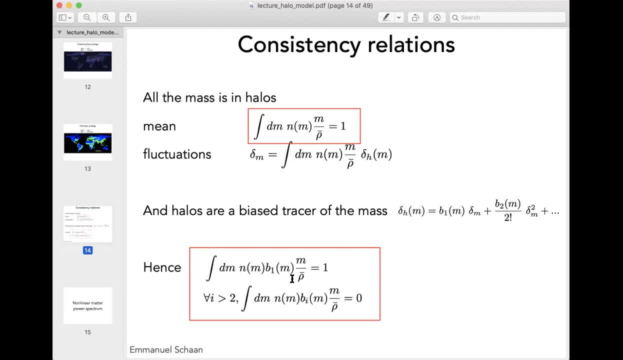 is that whatever halo mass function and bias model you're using, they have to satisfy this consistency. And if I go to higher order in biasing, for example, second order, where the halo matter density field depends on the square of the matter density field. 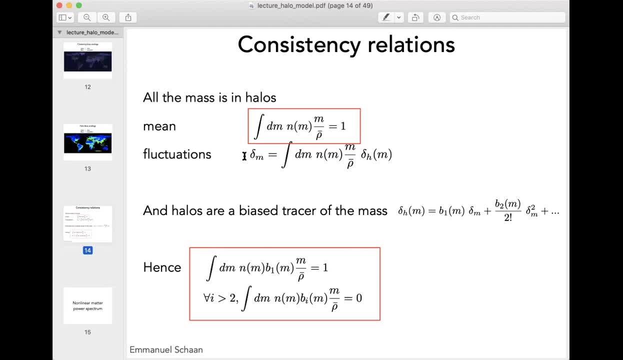 again, because of this constraint- and you have no second order term on this side- you need the integral. you get to be equal to 0. And this is this next consistency relation. So this is just something I wanted you to have heard about, this issue of consistency relation. 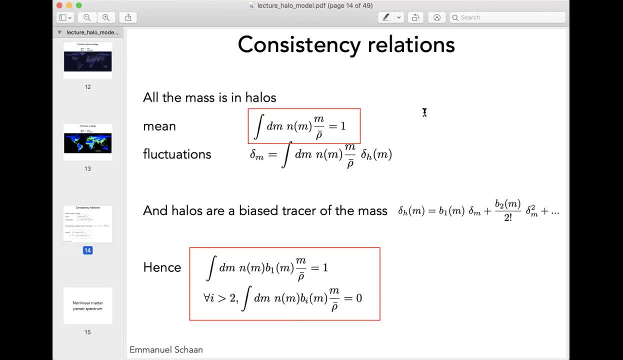 And we'll say a little bit more about this towards the end, when we talk about limitations of the halo model. But for now that's it for the ingredients of the halo model. So we have the halo mass function, We have the halo profile. 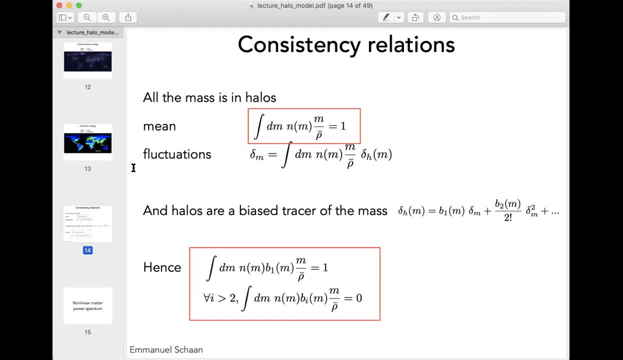 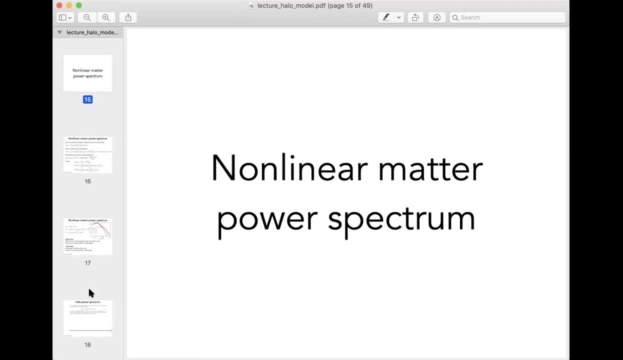 And we have halo bias. So how do we combine these things to predict some observables? And the observable we'll start with is the nonlinear matter power spectrum. So, if you bear with me, there will be a few slides of derivation that I'll walk you through. 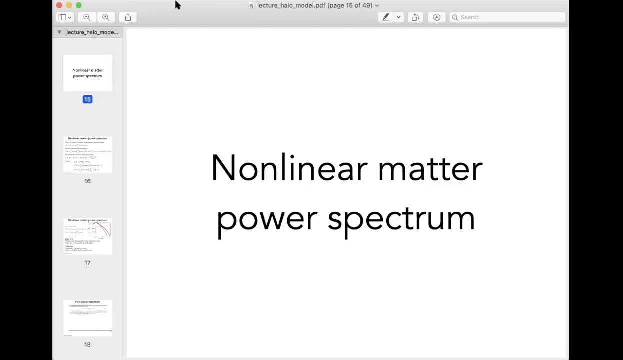 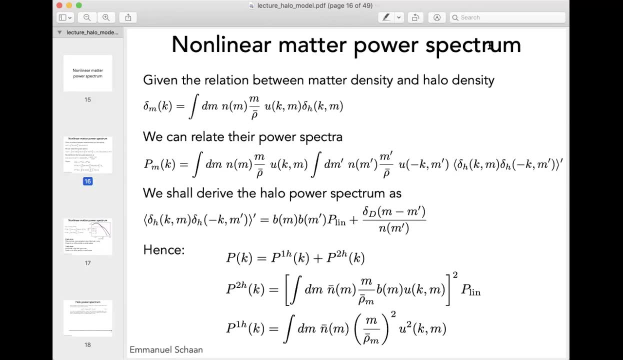 And after that it'll be much less dense And we'll just look at applications of the halo model. OK, So say, I would like to derive the nonlinear matter power spectrum in this halo model. How do I do this? And so, as we've seen, there's a relationship. 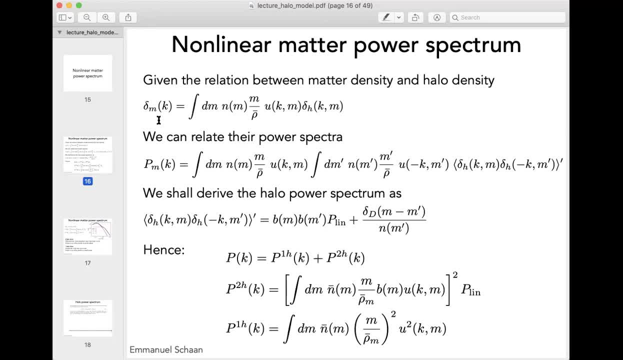 between the matter density field and the halo density. The fact that to get the matter density field all I need to do is take my halo over density field for each halo mass and weigh them by how many halos of that mass I have and how massive those halos are. 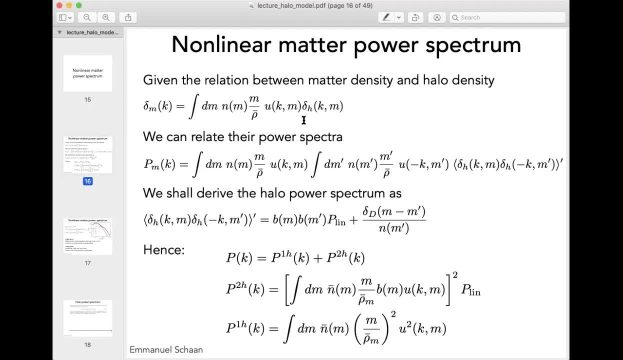 What you see here is this additional term u of k and m, And that is the Fourier transform of the halo profile that we talked about. So that's an NFW function, but in Fourier space. The reason I'm switching to Fourier space as opposed. 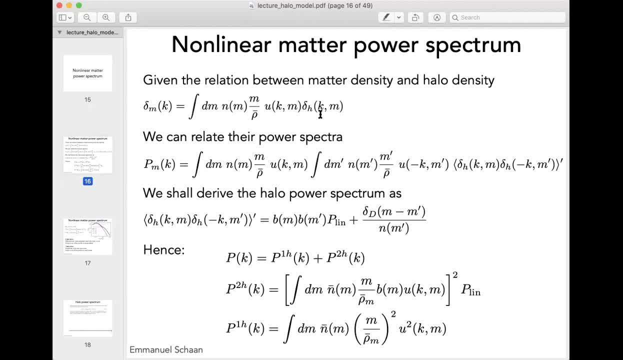 to real space is. you can see, here I have the product of two functions of k, And in real space this would be a convolution, And so writing it in Fourier space is convenient to avoid those convolutions. OK, So we have an expression for the matter: density field. 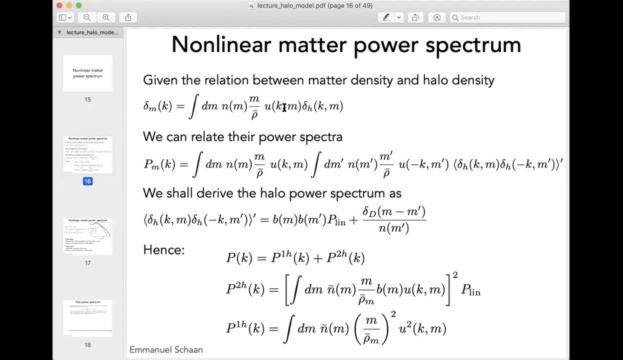 as a function of all our ingredients: halo mass function, halo profile and halo over density, which we know how to express in terms of bias. OK, So, given this matter over density field, what is its power spectrum? To get the power spectrum, what I'll do? 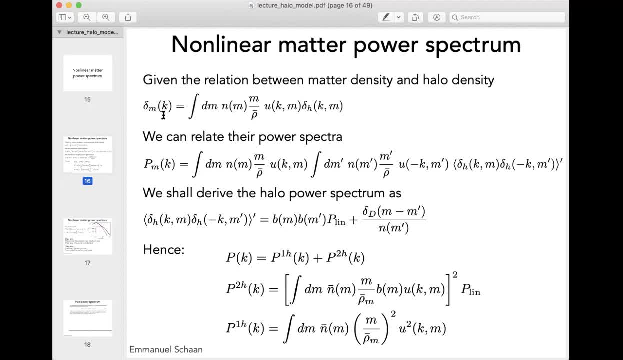 is, multiply this quantity by itself, but minus k, And so I had one integral. When I do that multiplication I'll get two integrals, So dm n m over rho bar u, dm n m over rho bar u, And for the second delta I get again the same integral. 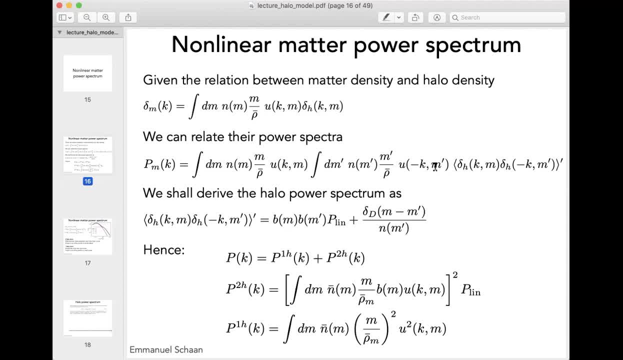 but with m prime instead of m. And when I take the expectation value, I get this expectation value of the product of the halo over densities at mass m and m prime. And the key insight of the halo model is that this quantity, which is the power spectrum, 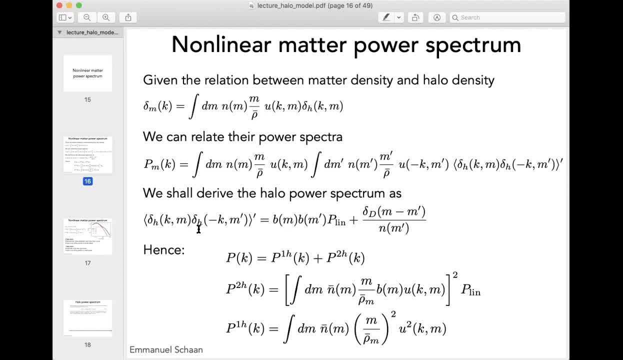 of the halo number density can be expressed as follows: Linear bias at mass m. linear bias at mass m. prime times the linear matter power spectrum, plus an extra term which is a shot noise term, And it's the shot noise of halos. 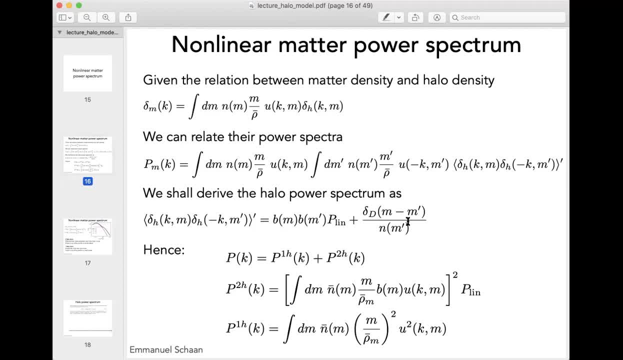 And it scales as 1 over the mean number, density of halos. So if I now plug this sum of two terms in this double integral, what I get is that the power spectrum is the sum of two terms. And if I start with those b terms, 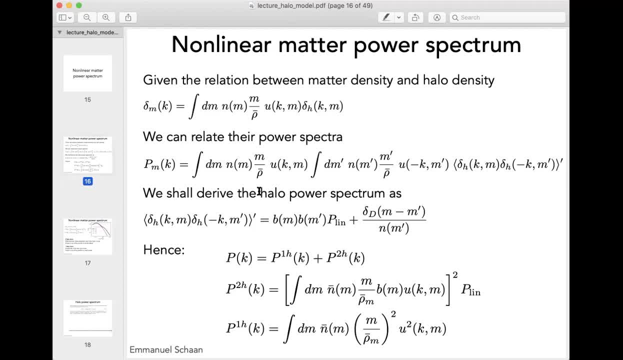 what you see is that p-lin here goes out of the integral And b of m, b of m prime, makes this whole thing separable. What I end up with is this so-called two-halo term. So again, p-lin outside of the integral. 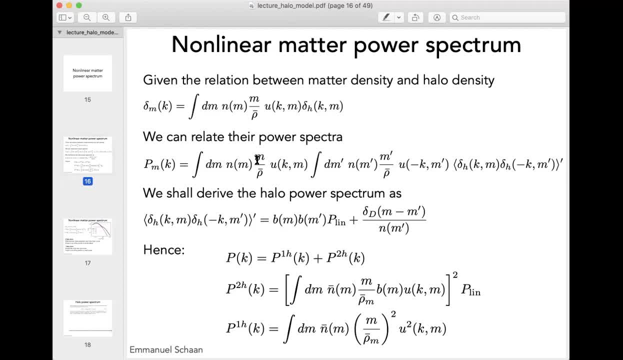 the integral of mass which you can see here and m over rho u and m over rho u And the bias right here. So this is the so-called two-halo term And finally, if you plug in this second term in here: 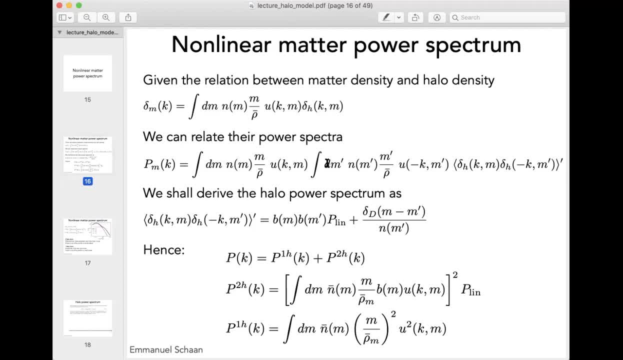 this delta drag in mass kills the second integral in mass, And this 1 over n kills one of the two n's of m. So you end up with only one integral, only one halo mass function as opposed to 2. And you get the m over rho bar. 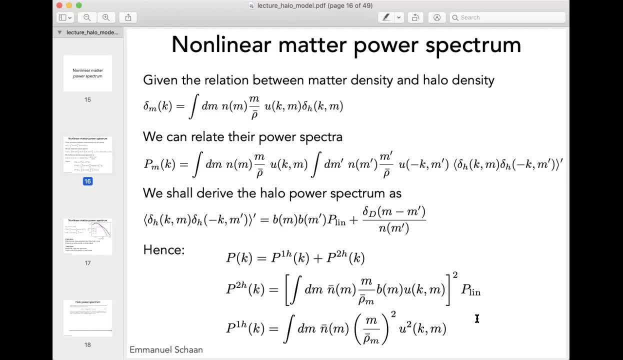 And you get the m over rho bar squared and the u squared And this is called the one-halo term. So now, why are these terms called two-halo and one-halo term? I'll explain a bit more about this, But you can think of them schematically. 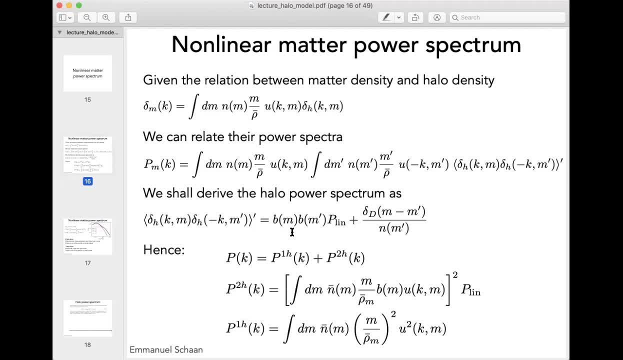 as being the clustering for halos of the same mass or particles coming from the same halo, for the two-halo term and oh, sorry, for the one-halo term- Being particles coming from two different halos of two different masses. So let me just rewrite this expression again in this slide. 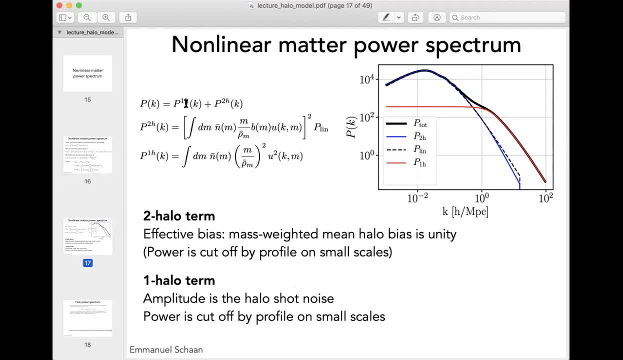 So the power spectrum of matter is the sum of a one-halo and a two-halo term, And let's look at what these terms look like in practice. when you evaluate- And this is a calculation again- you can do with the code on the repository I listed. 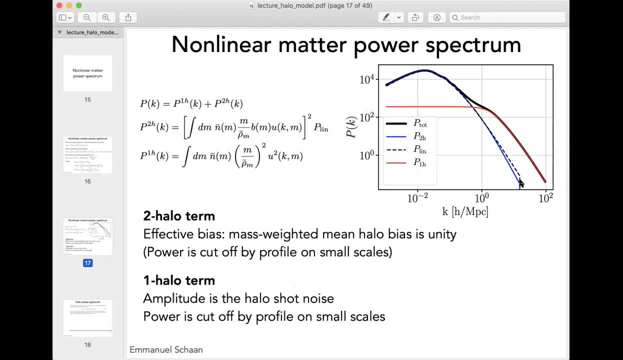 So here's the matter: power spectrum as a function of scale And dashed line is the linear matter power spectrum. You can get it from CAM, for example, And again, we'd like to predict the nonlinear power spectrum. The halo model gives it to us as a sum of this two-halo term. 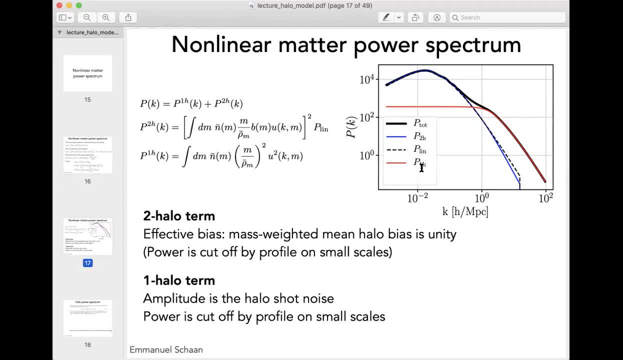 and this one-halo term. The two-halo term you can see in blue- looks very similar to the linear power spectrum on most scales And the one-halo term is a really new term. It looks constant on large scales and then goes down. 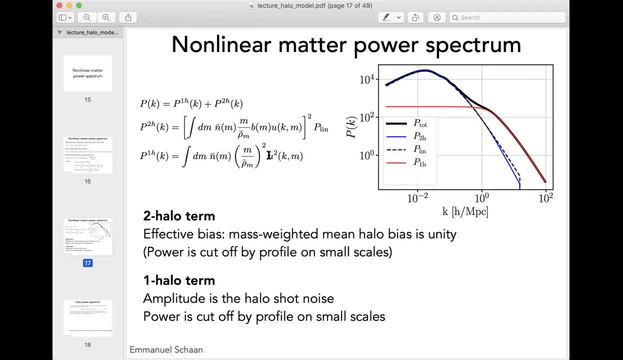 And the scales at which it goes down are determined by this profile u of k. So this curve you're seeing here is really just the Fourier transform of the halo profile, properly weighted by mass. So that's the one-halo term. It tells you about the halo profiles. 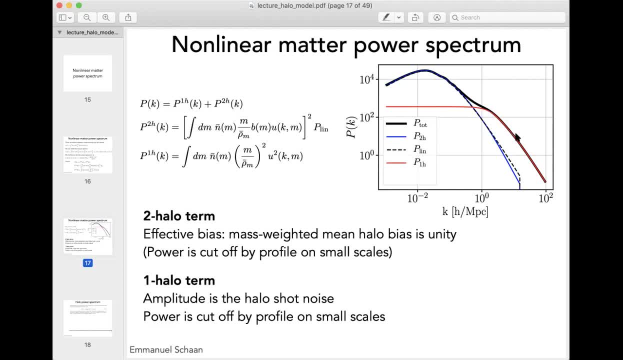 And it adds a large contribution to the matter. power spectrum on small scales- The two-halo term as we described, matches very well the linear power spectrum on large scales, And this should not be a surprise. It has to do with the fact that, if you forget, 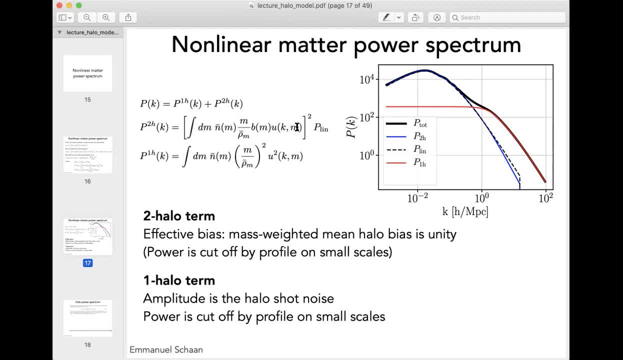 about this u profile, which is constant and one on large scales. this integral here is exactly the consistency relation we talked about for bias, And so on large scale, where the profile is irrelevant and it's just one, this integral goes to unity. 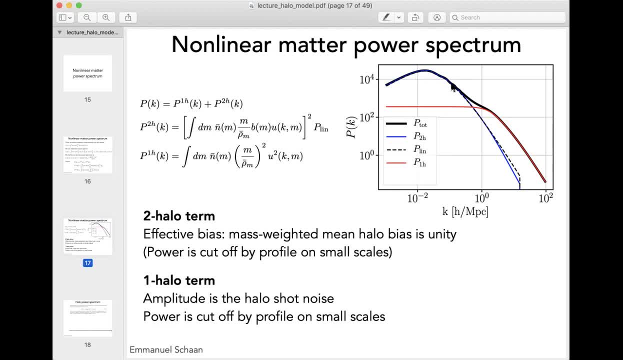 And this is why on large scales the two-halo term matches the linear power spectrum. On small scales this profile starts to go down, Just like you see in the one-halo term. So this turnover here in the one-halo term, 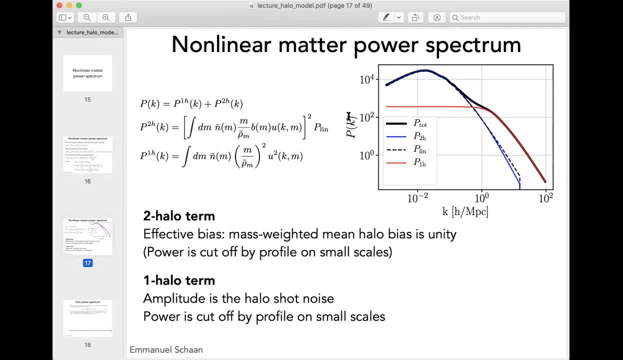 is the scale dependence of the profile, And the same thing happens in this integral for the two-halo term, causing the two-halo term to drop below the linear power spectrum on small scales. OK, so this is one of the key results of the halo model. 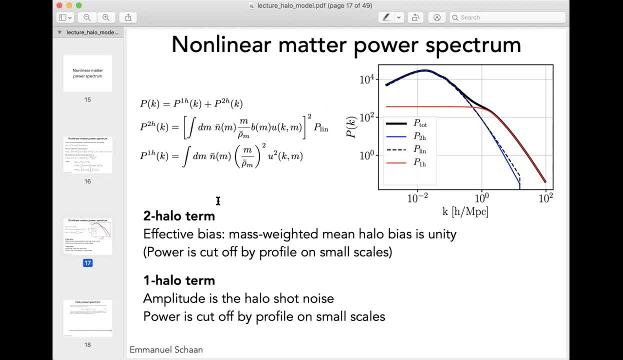 predicting the nonlinear matter power spectrum. We talked about this two-halo term where you can think of this overall integral as an effective bias. Effective because it's an average of the halo bias, average over mass, weighted by how many halos there are. 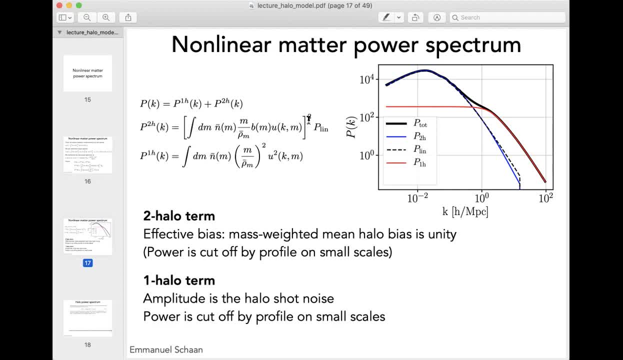 how massive they are. So the two-halo term is the linear power spectrum times, an effective bias, And again this bias goes to unity on large scales, And the one-halo term, on the other hand, which comes from this shot, noise of halos. 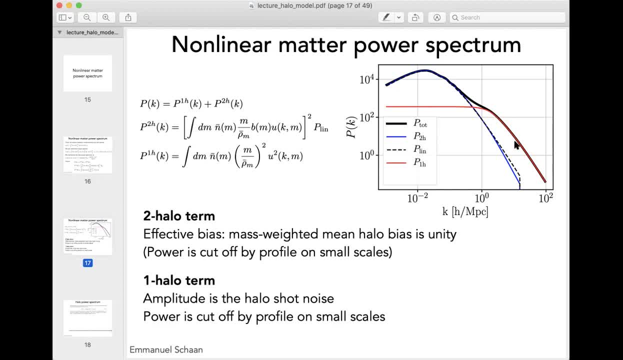 and I'll say more about this- has this cutoff on small scales And basically tells you about the halo profile. So this is already kind of interesting that with some three simple ingredients- halo mass function, halo profile and halo bias- we can predict the nonlinear matter power spectrum. 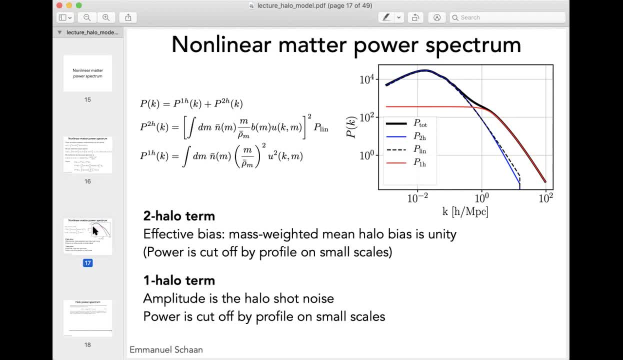 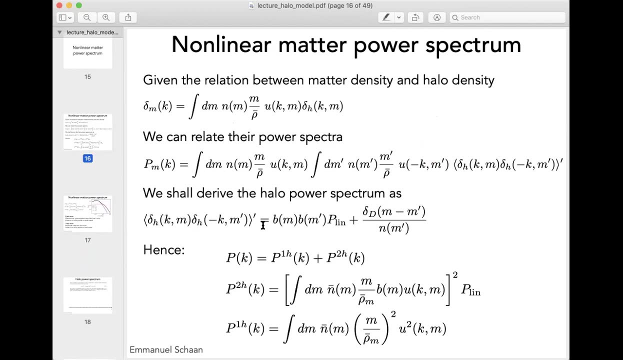 And so that's one of the key results of the halo model, And now I could go into more details about this one step in the derivation, this thing that I asked you to accept: the fact that the power spectrum of the halo number of a density- 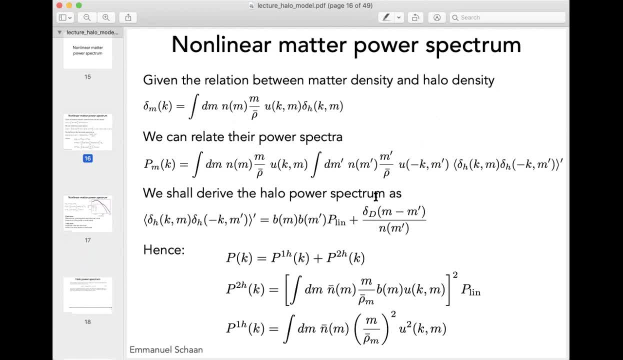 is related to linear matter power spectrum with linear bias plus this shot noise term, And I think what I'll do is keep this derivation in the slides that I'll give you guys afterwards so you can look in detail, And instead I'll give a simpler sort. 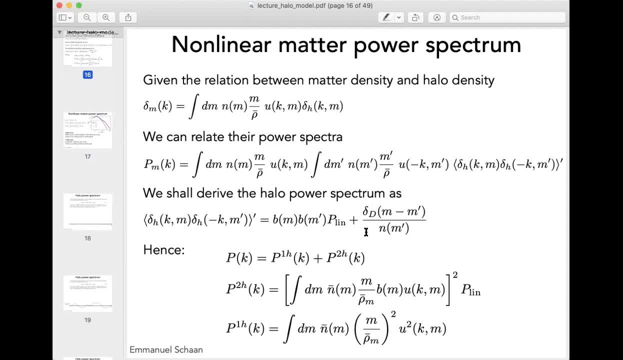 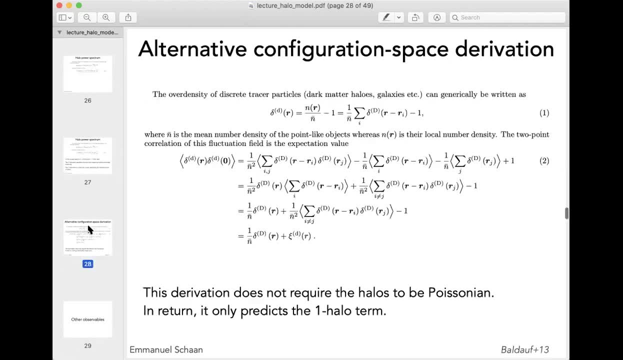 of schematic derivation for where this shot noise comes from, And so this is what I'll do now. OK, So the question was: when we look at the power spectrum of the halo number over density, why is there this additional shot noise term? 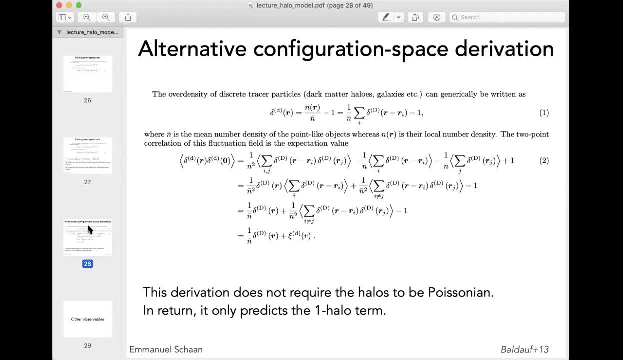 Where does it come from? And we called it a one halo term, meaning this is the clustering when two points are within the same halo. Where does that come from? So here is, I think, the shortest and simplest derivation of this. It comes from this paper by Tobias Baldov, which 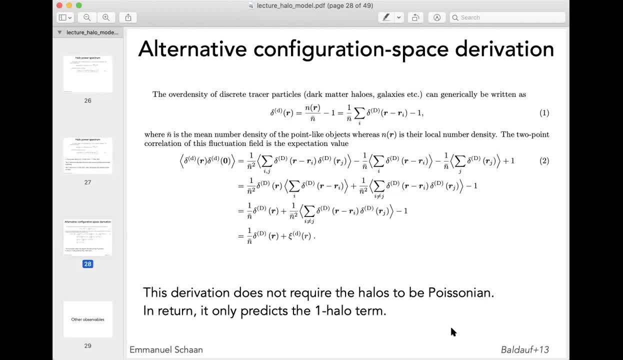 I really recommend. It's super pedagogical And here's how it goes. So here this delta D is basically our delta H. so the halo number over density, which is related to the local number, density of halos over the mean. 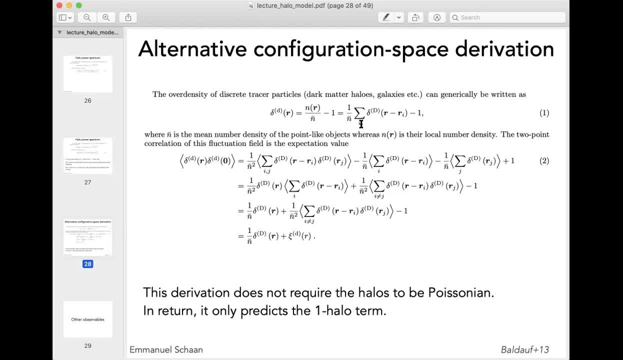 And you can express this quantity as a sum over all the individual halos, because the number density of halos is basically the sum of a Dirac delta at the position r i of halos. So the halo number density is the sum of Diracs. 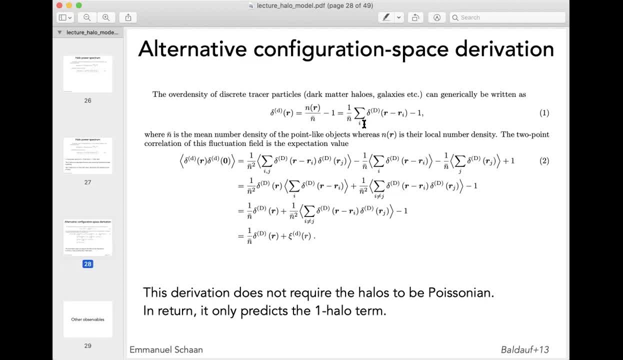 at the position of halos, And here the sum is over halos. OK, So given this halo over density, what is its correlation function in real space? You can obtain this quantity by just taking the mean of the halo over density at r times the halo over density at, say, the origin. 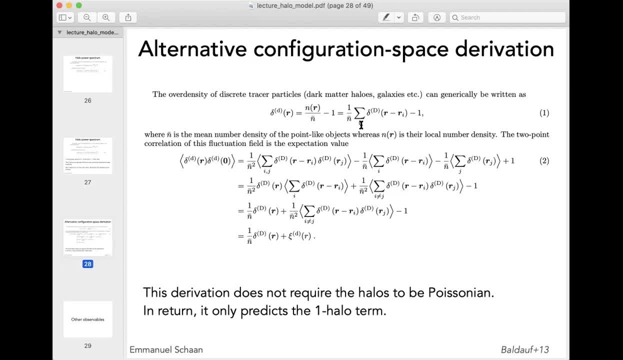 And this is now just algebra. So you have two sums: sum over i in the first term, sum over j in the second term. And this is what you get here, And because you have the minus 1s, you end up with the minus 1 squared. 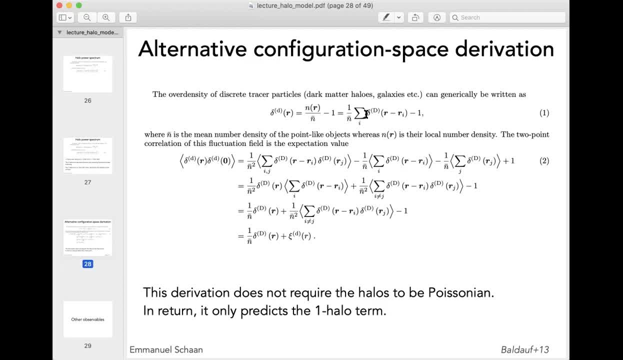 That's plus 1.. And the cross products minus 1 times the sum. And these are the sums. Something you'll notice is that once you put the expectation value, the sum, over these Diracs, the average of it is the mean. 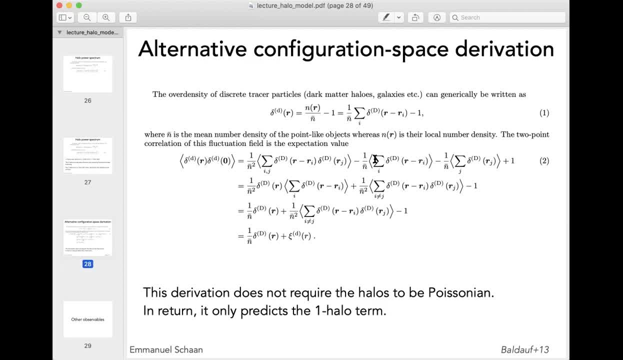 The number, density of halos, that's n bar. So this term gives me n bar over n bar, which is 1.. Similarly, this term gives me n bar over n bar, which is 1.. And so I have minus 1,, minus 1,, plus 1.. 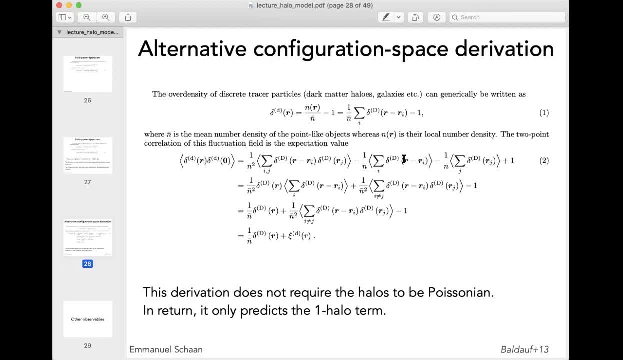 That gives me minus 1.. That's this minus 1.. Now let's deal with this term. We have this double sum, And here it's helpful to split the sum into the cases where i and j are different, meaning we're. 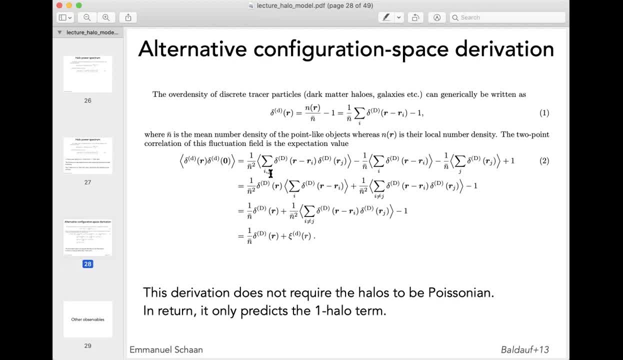 looking at two points in two different halos And the case where i equals j. So the two points ri and rj are in the same halo. So when you look at i equals j, what you get is the product of a function that's delta, Dirac at ri. 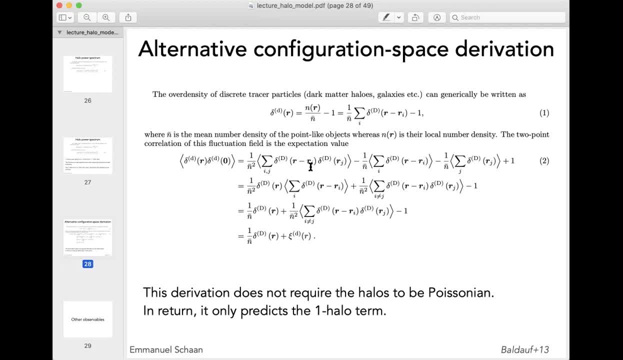 and this delta Dirac. So for this to be non-zero, when i equals j, you need r to be equal to ri. That's this delta function. And you need rj, rj, which is ri, since i equals j, to be 0.. 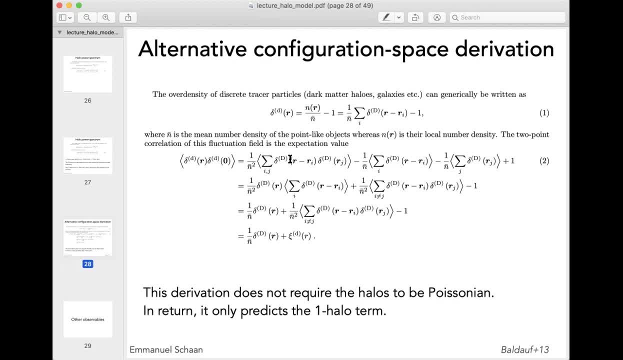 And so, because r is ri, you need r to be 0. So this term, when i equals j, gives you this. So you still have the 1 over n bar, You have a Dirac delta of r And you have this quantity, which again. 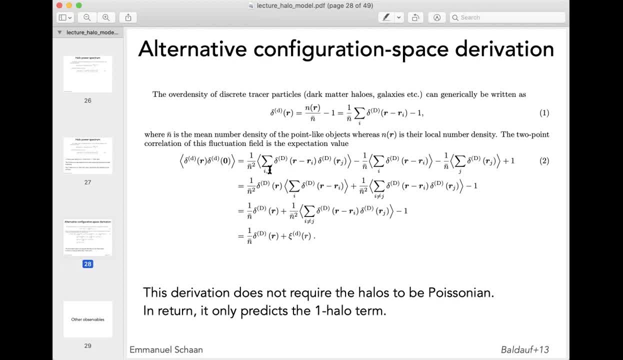 is the mean number. density of halos. OK, So that was the part where i equals j. Then in this sum you have the part where i is different from j, And here we just repeated it And you can see that it's not there. 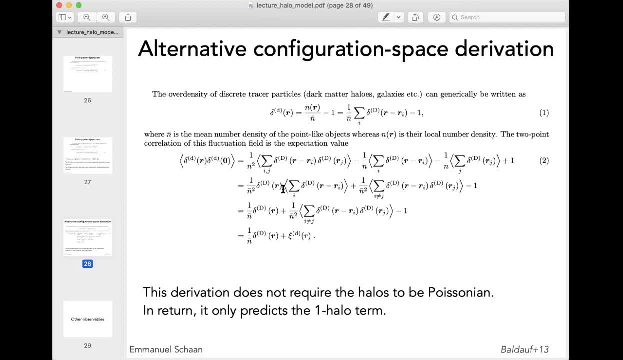 OK. So again, the expectation value of this sum is n bar, So I end up with n bar over n bar squared, So that's 1 over n bar. And what you see here in this derivation is that you end up with this extra term, this delta Dirac. 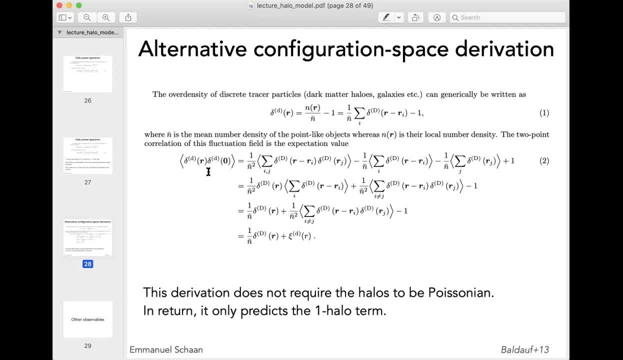 at the origin in the correlation function of the halo number, density, And this is a term that's non-zero, only basically in the same halo. So that's why it's called the one-halo term And that's why it scales as 1 over n bar. 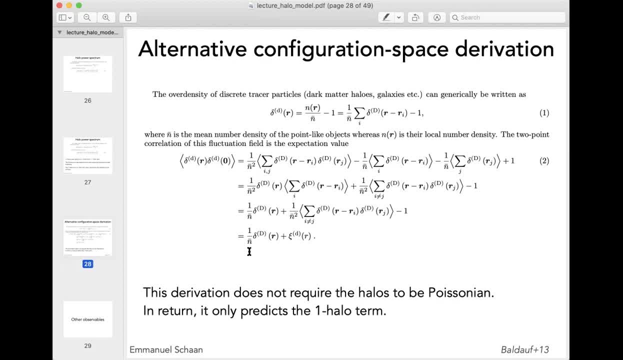 So that's the derivation for this one-halo term. Now, if you want more detail about this additional term that I haven't talked about, I'll invite you to look at the slides And I'll put them online for you to see after the lecture. 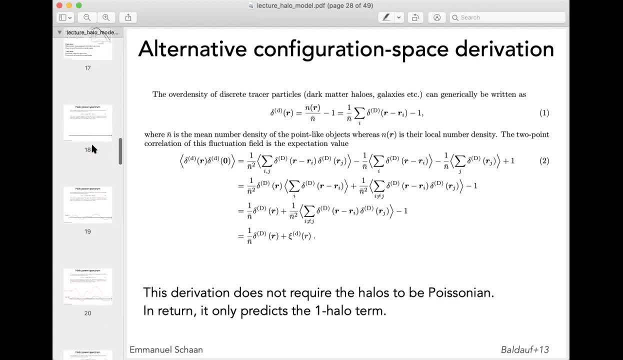 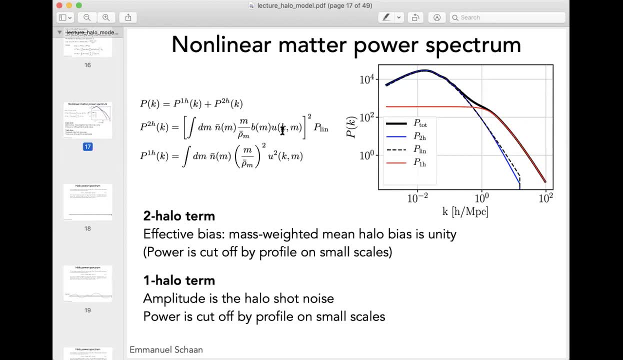 OK, So sorry, That was a lot to swallow, But really all I want you to do is to remember about this is that, given the halo mass function, the halo bias and the halo profile, the halo model lets you predict the nonlinear matter power spectrum. 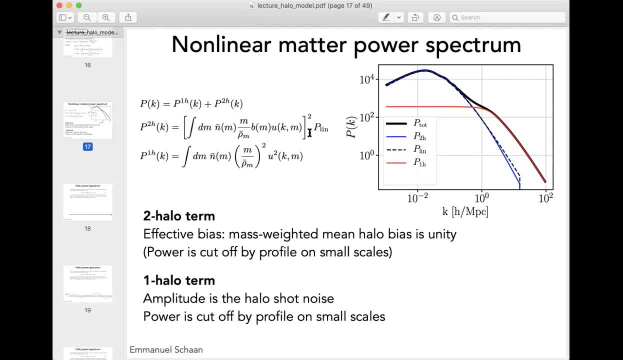 as a sum of two terms: the two-halo term, which is very similar to the linear power spectrum and has to do with the clustering of halos, and the one-halo term, which is a shot noise from the discreteness of individual halos. 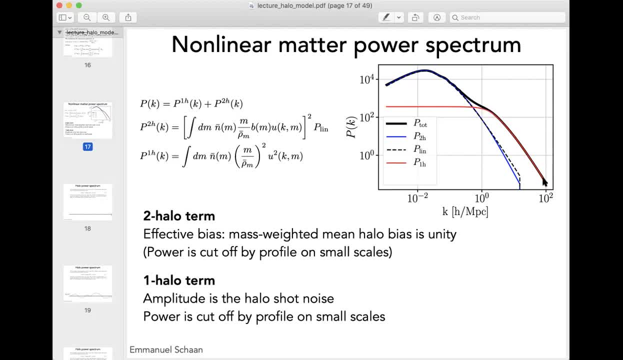 And it's flat on large scales and it goes down with the profile. So if you really just remember this, that would be a success, And I'm now going to move on to talk about other observables. So if there are questions on this, 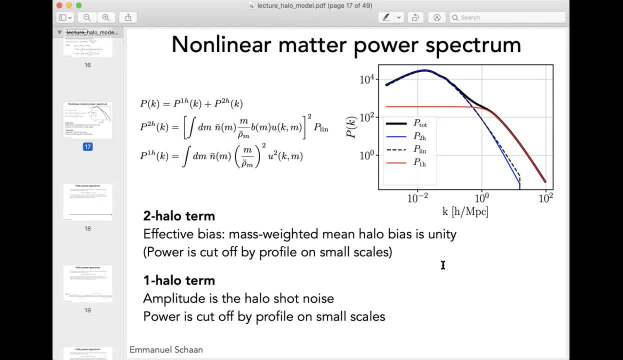 that would be a good time to ask: Sorry, It's nonlinear, because you're measuring the nonlinear halo power spectrum and then from that inferring the matter. Right, Sorry, Yeah. So the reason this predicts the nonlinear matter power spectrum is because the idea is that the number, density of halos 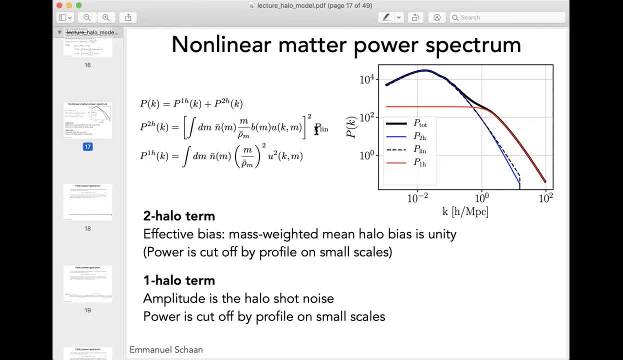 on large scale, traces, the large scale density field, which is the linear density field. But by capturing the fact that the matter has collapsed into those halos, you are capturing the nonlinearities of the evolution under gravity. So if, instead of putting your mass inside of halos, 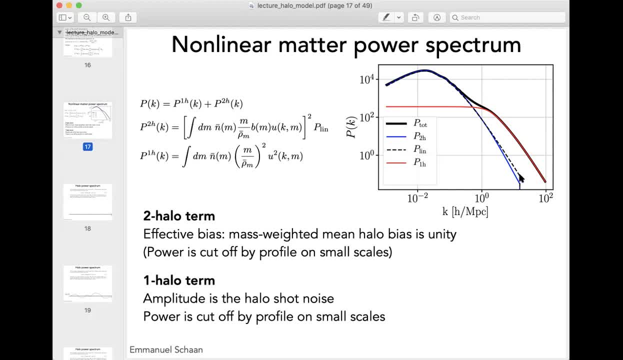 you kept them diffused, like the large scale matter density field, you would have this linear power spectrum. But once you put all the mass inside of those individual halos you get this additional term, And so this additional term here on small scales describe the nonlinearity of the evolution. 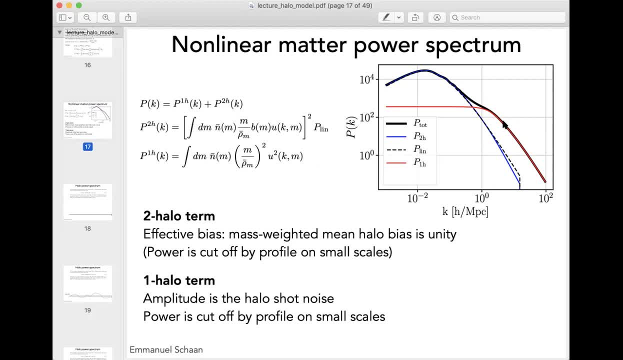 of the matter. density field under gravity: OK, And if you include the higher order bias terms, you still end up with just one and two of halo terms. But that's only because of our choice and our consistency condition, Right, So there is a bit of subtlety. 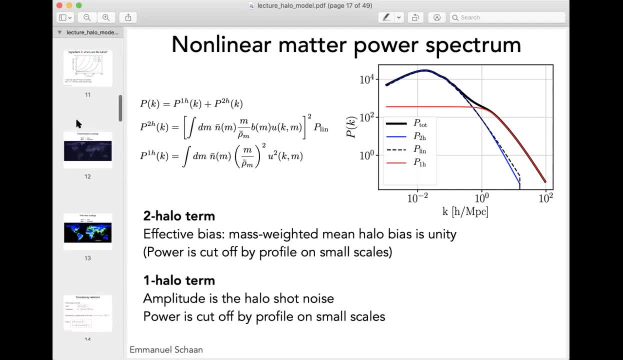 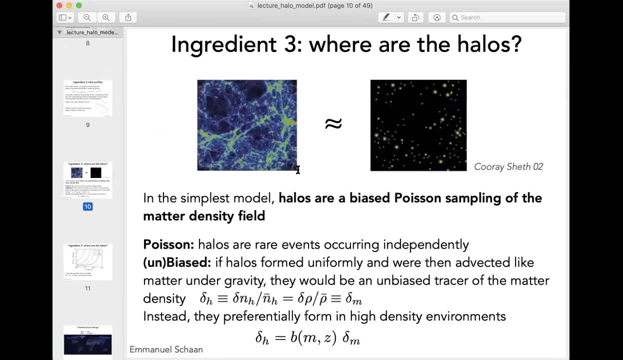 And I sort of swept this under the rug And the subtlety is in this question of linear bias. I related the halo number density field to the matter density field And here I was a bit schematic in not specifying whether this was the linear or nonlinear matter density field. 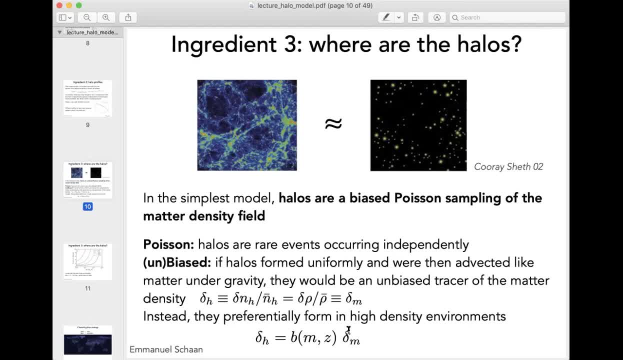 And different halo models differ in the implementation. So some people might put the linear or nonlinear matter density field And some people might include higher order terms And this makes the halo model a bit more complicated. In the simplest form it modifies the two halo term. 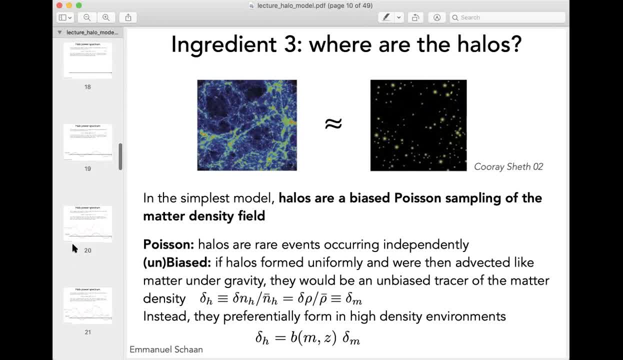 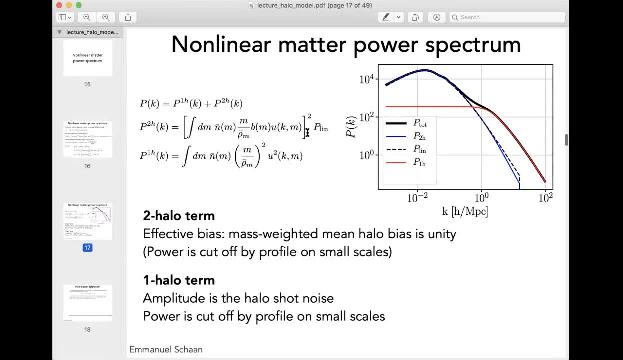 And so what you might often see is that, instead of having the two halo term look a lot like the linear power spectrum, you might have the two halo term look a lot like the perturbation theory power spectrum with your given bias: expansion, Yeah, Yeah. 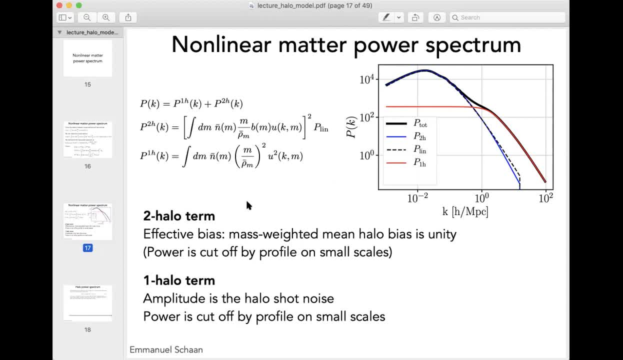 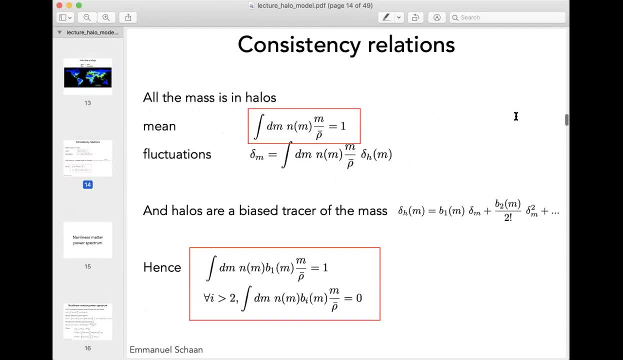 Thanks, Noah, That was a very good question. Sorry, The last question that I had was about the consistency conditions that we were writing down. Are these, I mean, are these unique? Do you mean, do they specify uniquely what the halo mass? 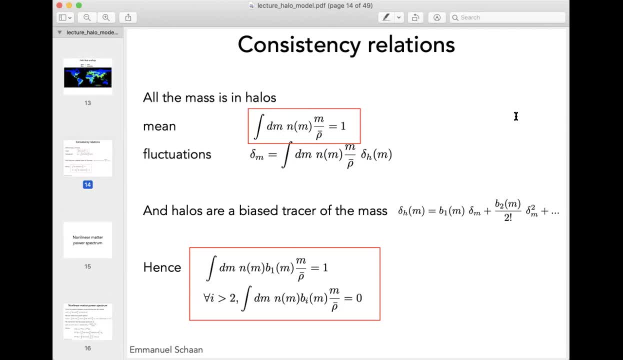 function bias should be or No. I mean you can't derive the consistency relations. They're kind of a choice. Is that true, Right? Yes, So here, those consistency relations are a consequence of the assumption that all of the mass in the universe is inside of halos. 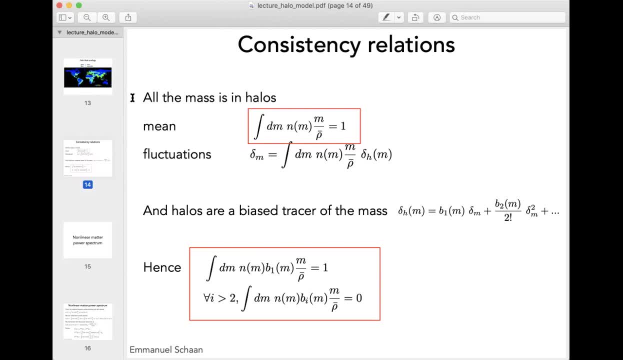 And this is something I'll talk about at the end, because this is an assumption you can question: Is all the mass in the universe really in halos or is there diffuse mass around them? And what you find when you look at simulations is that the halos you're able to measure. 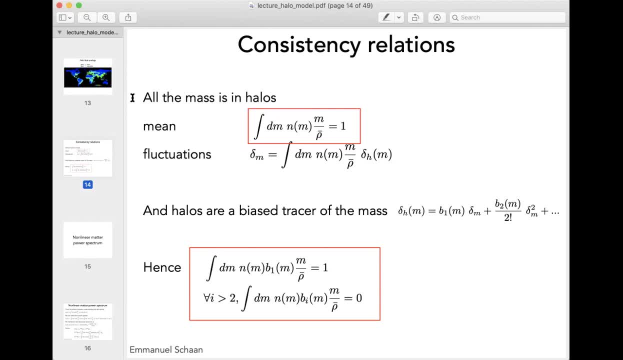 do not account for all of the mass, And so there are tricks to make those consistency relations valid, And so I'll say more about this. But basically, yeah, this is a very good question of whether or not you should trust those consistency. 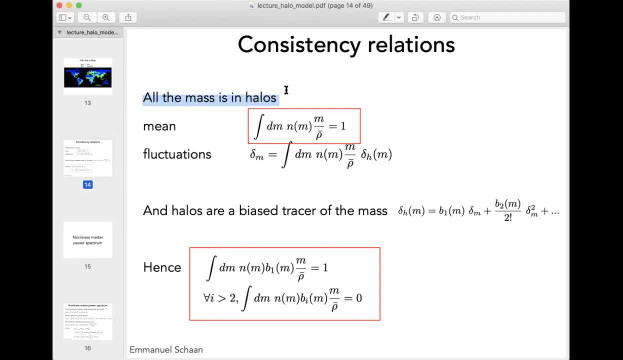 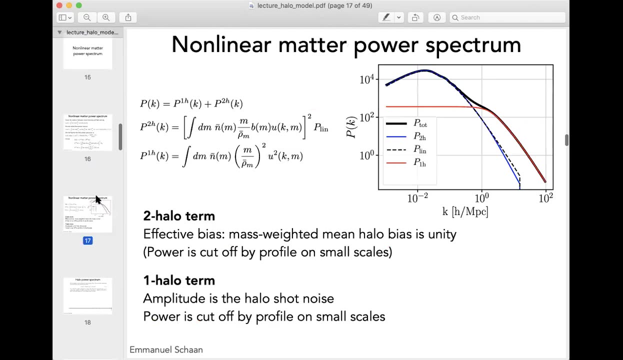 relations, given that they come from this assumption, And so I'll say a bit more about this And, if not, don't hesitate to ask again. OK, Cool, Thank you so much. Any other questions before we move on? All right, 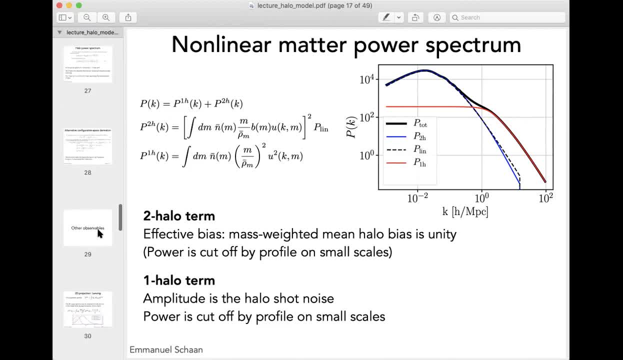 So in that case I'll move on to talk about other applications of the halo model, meaning applications to other observables than the matter power spectrum or the matter density field, And the reason for this is because there are a lot of models out there for the nonlinear matter power. 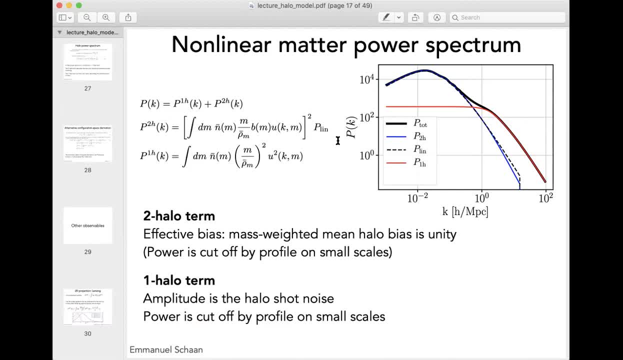 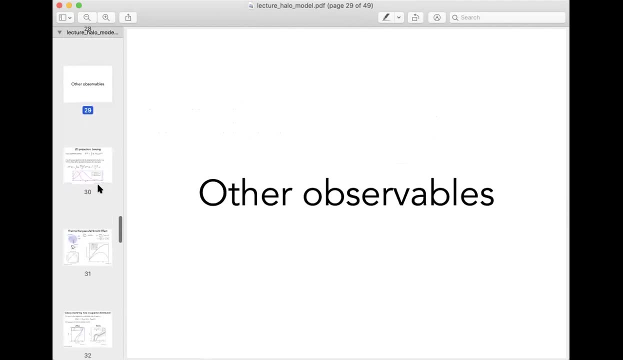 spectrum. This is something you can simply measure in simulations. There are a lot of perturbation theory models that do very well at this, And so if this was the only selling point of the halo model, maybe it wouldn't be very interesting, But it turns out there's a lot of other selling points. 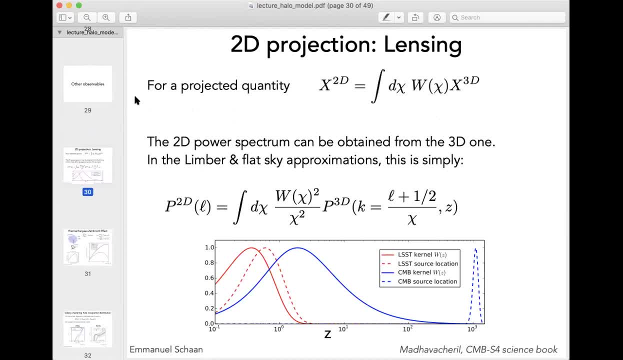 So first thing I wanted to say is, once you have the power spectrum of any 3D observable, which I called here x3D and that could be the 3D matter density field or that could be the 3D number density field of galaxies, 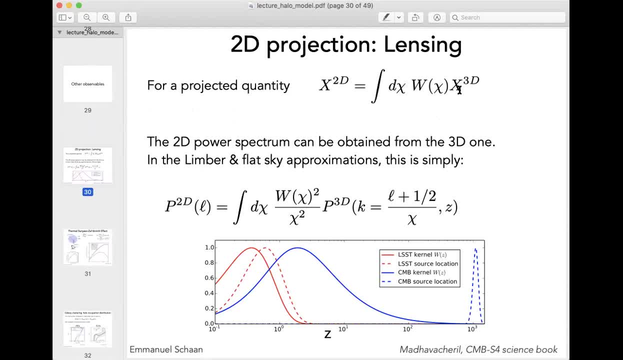 for example, It's easy to convert it into the power spectrum of 2D observables, like the 2D number density field of galaxies for a photometric survey, Or one useful application is that of gravitational lensing, And so a lot of people are working. 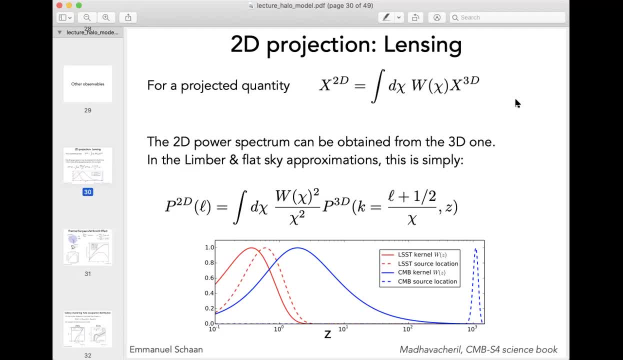 on measuring gravitational lensing of the cosmic microwave background or galaxies, But in all cases the lensing field is simply the projection along the line of sight. Here is the moving radial distance Of the matter. density field with some redshift kernel. And so here this plot shows you what a redshift kernel might. 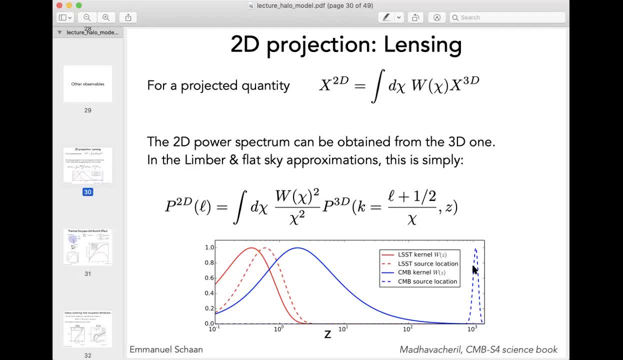 look like. So if you care about lensing of the CMB which comes from redshift 1000, the CMB lensing has this kernel picking at redshift about 2 and very broad meaning the lensing is caused by this integral. 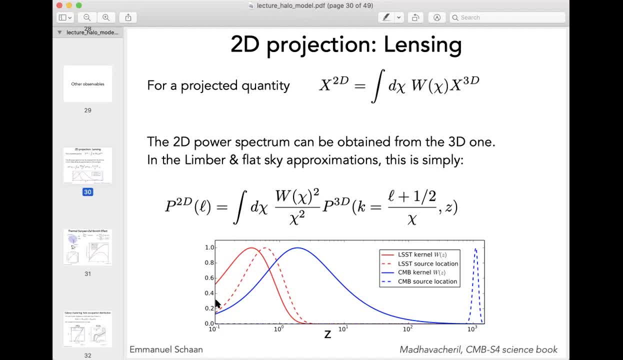 over the line of sight of the matter density field with this kernel, And here in red I'm just showing the equivalent for galaxy lensing. But the point is, once you have a model for the 3D nonlinear matter density field, you can then therefore, 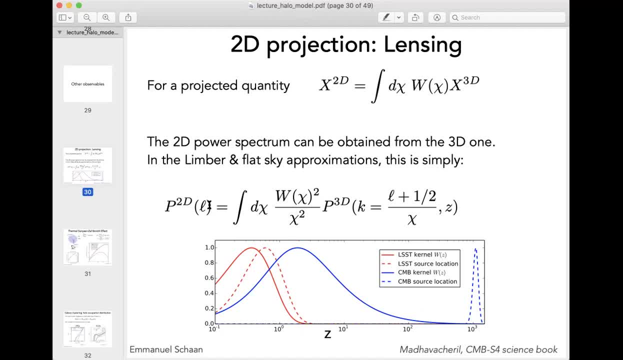 get a model for the 2D power spectrum of lensing by computing this integral. So this is the so-called Limber approximation and Flat-Sky approximation. You may have heard about this already in class, or you might at some point, So I won't say too much about this. 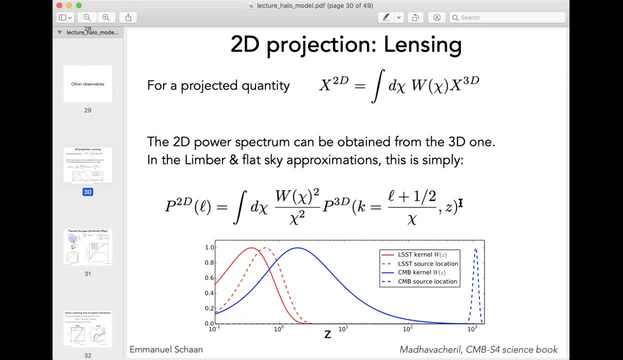 but I just wanted to advertise that once you have a model for the 3D matter density field from, for example, the HALO model, you can use this to predict CMB lensing or galaxy lensing. So that's already one application of the HALO model. 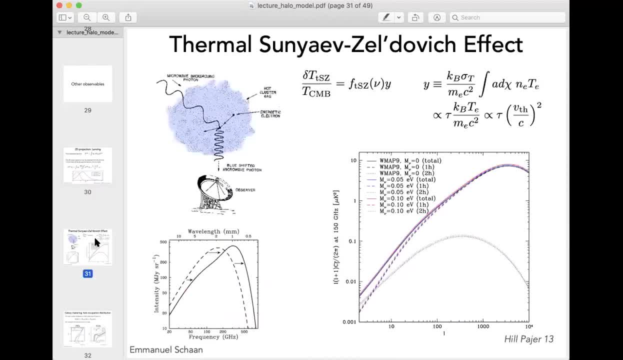 An other application is other observables. So instead of caring about the matter density field here, I'm pointing on another application, the so-called thermal Sunyev-Zeldovich effect. this is something you may or may not have heard about, And it's the fact that, as the cosmic microwave backgrounds 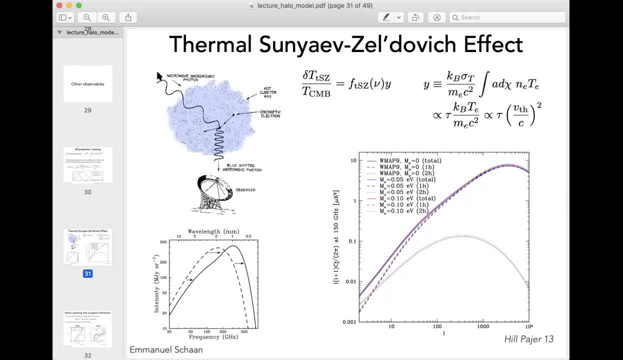 photons travel from the surface of glass scattering towards us, they may encounter clusters And these clusters have hot gas with pre-electrons And this hot gas around clusters imprints a shadow on the cosmic microwave background And this shadow is a change in the temperature. 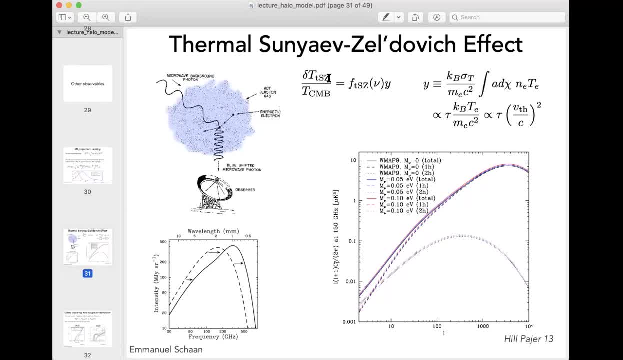 that you see, due to this thermal Sunyev-Zeldovich effect, It has a known frequency dependence and its amplitude is determined by an integral along the line of sight of the product of density times temperature of those electrons in the gas. And so here we're again in the case of a 2D quantity. 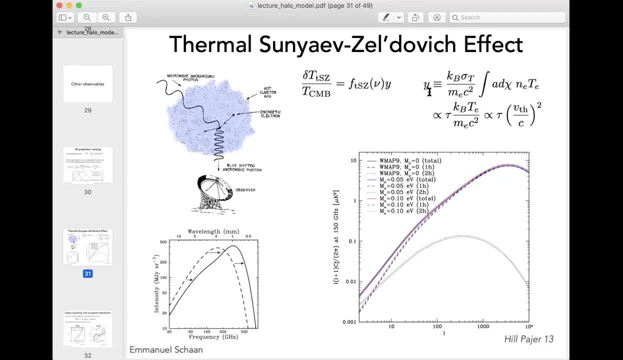 So you have a 2D map of the CMB And the effect here, the Sunyev-Zeldovich effect, is a projection along line of sight of 3D quantities, which is number, density times, temperature of electrons. 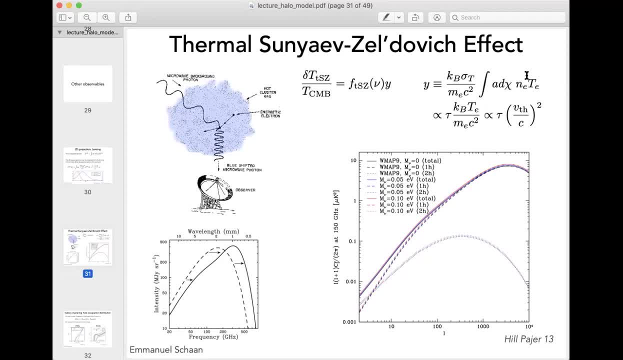 And so people have built HELLO models for the number, density, times, temperature of electrons. And once you know those profiles of HELLOs, since we know the HELLO mass function and the HELLO bias, we can predict the power spectrum. And so here's a prediction for this CLY. 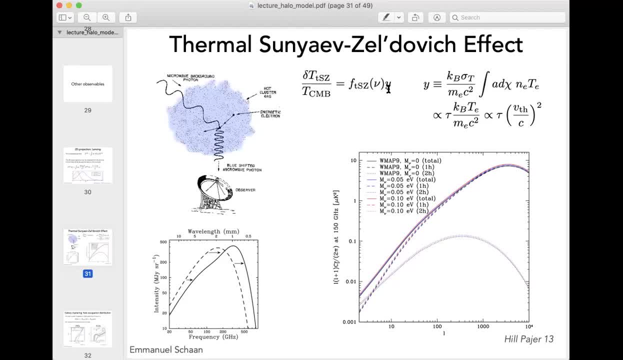 the power spectrum of this Compton Y parameter, which again determines the amplitude of the LZ effect. And so the HELLO model tells you what this power spectrum is as a function of angular scales- little L here- And the shape might look different from what we've seen before. 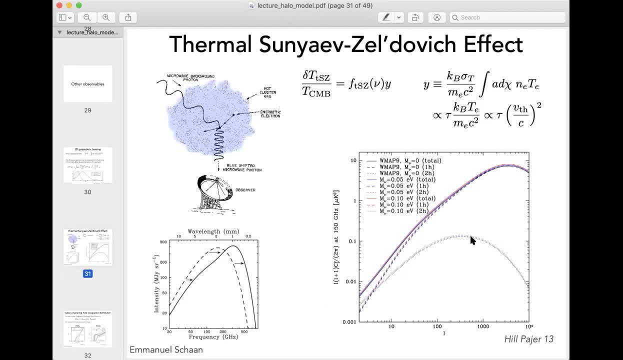 but again you have sort of two terms: One which is negligible on small scales but large on large scales, is this two HELLO term, And the other term here is the one HELLO term which dominates on small scales at high L. 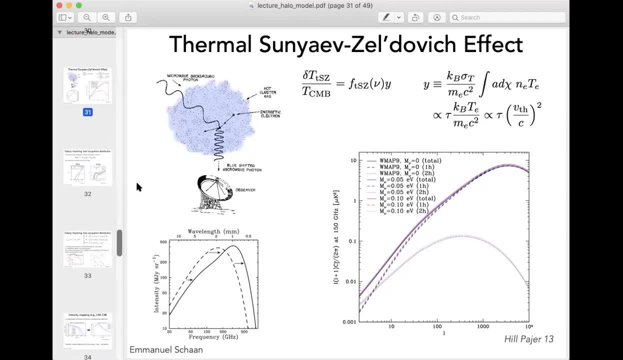 So you can already see that the HELLO model is pretty versatile, because these ingredients of HELLO mass function and HELLO bias are still useful here. Just the same, The only change is that the HELLO profile, instead of being an NFW profile, for the matter, density profile. 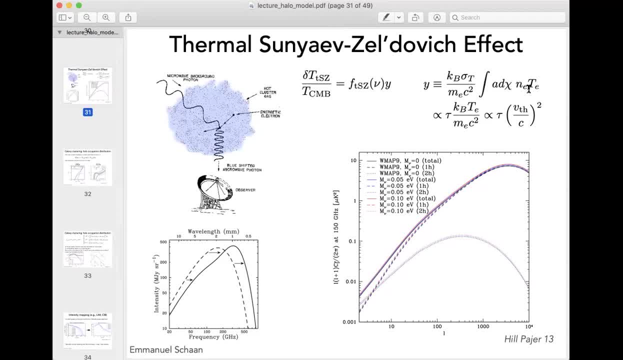 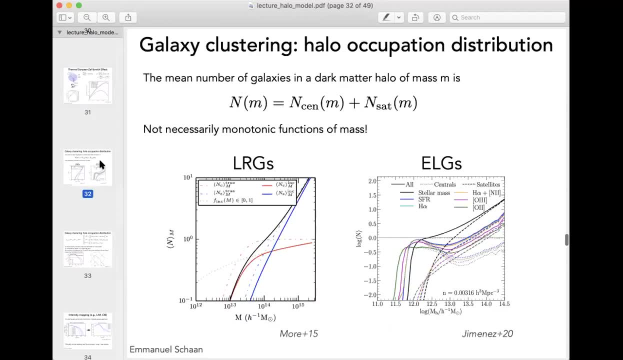 is just an electron profile of density times, temperature, And once you have that ingredient, you can predict the power spectrum of this observable. Another very important observable that the HELLO model is often used to predict is galaxy clustering, And so you'd like to know, for example, 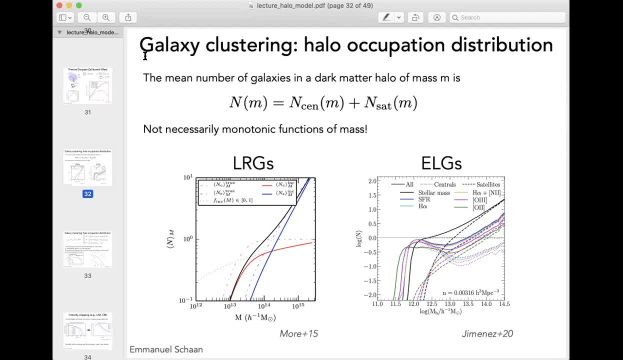 what is the power spectrum of the dynamic, the number, density of galaxies? And to do this again, you use the same HELLO mass function, the same HELLO bias, And you'd like to know what's then the HELLO profile in terms of galaxies. 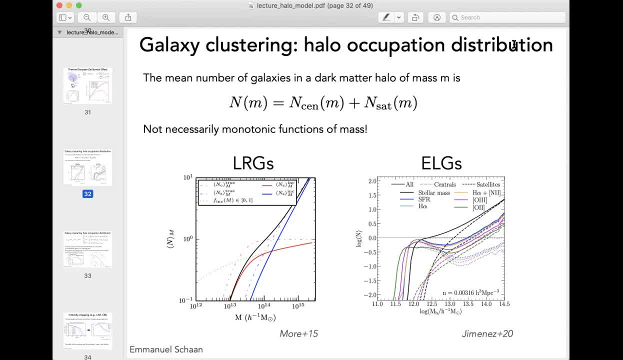 And this is typically parameterized by something we call a HELLO, occupation distribution or HOD, And it says that for a HELLO of mass m, you have a certain number of central galaxies, typically zero or one, that sit in the center of your HELLO. 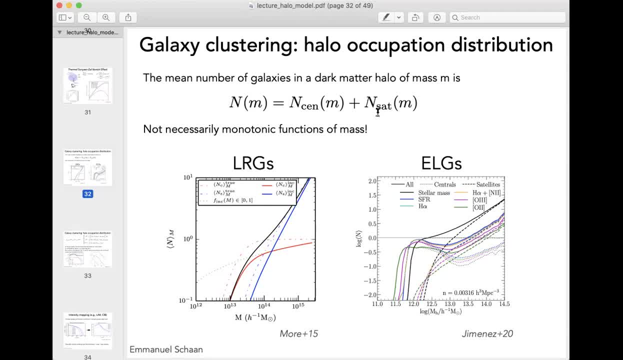 And a certain number of satellite galaxies, of which you can have many that follow often the NFW profile of the galaxy. So that's a typical prescription, a typical HOD, HELLO, occupation, distribution, And here there's many curves, but I'm showing examples of such HODs. 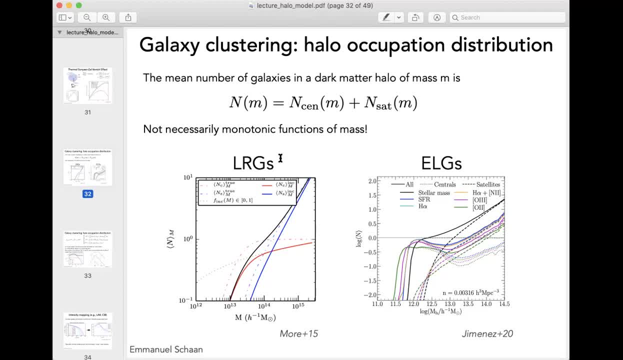 In the case of galaxies like luminous red galaxies that are selected based on their brightness, And what you can see here is the min number as a function of mass. In red is the number of centrals, And so at low mass you have basically 10 to minus one or less. 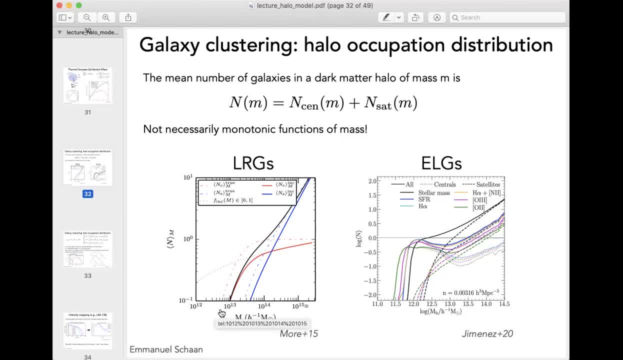 So basically no central galaxies in those low mass HELLOs And at high mass this gets to close to one, meaning all high mass HELLOs will have one central galaxy. Then in blue this quantity is the number of satellite galaxies. 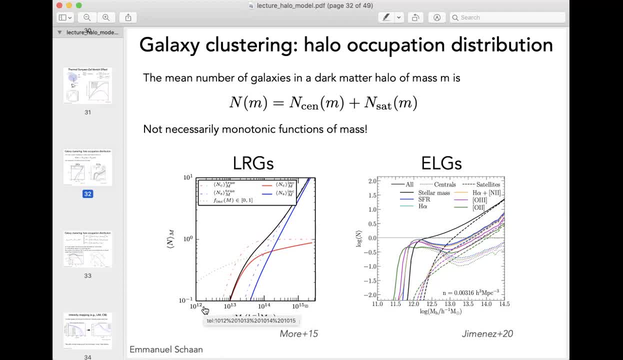 And this says: as the mass goes down you have fewer and fewer satellite galaxies, But as the mass increases you can have arbitrarily large number of galaxies, something like 10 in this example. So that's a HELLO occupation distribution Here, for I just wanted to show in this plot. 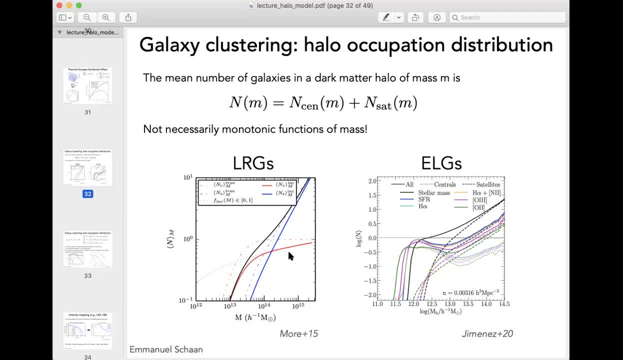 for emission line galaxies that those quantities are not necessarily growing monotonically with mass. And this is often the case where you look at galaxies that are not selected based on their the fact that they're bright and red, but based on their star formation rate. 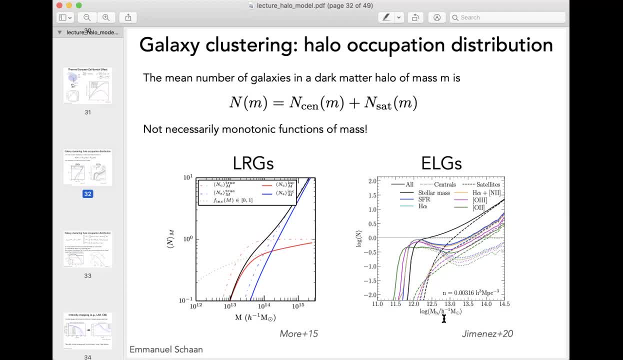 And the reason for this is that when you go to high masses there's a number of quenching processes that kill star formation and will therefore reduce the number of central galaxies you might be able to find. So this is sort of a slight digression. 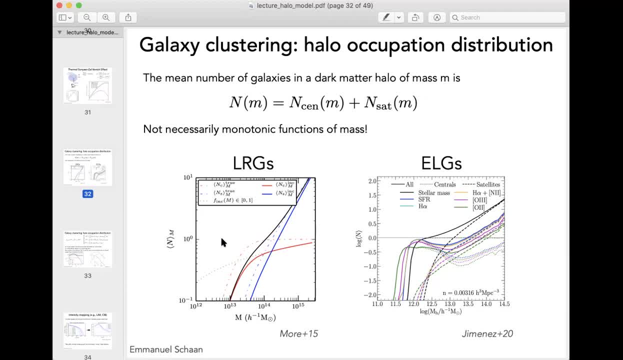 but I just wanted to show you what an HOD is and two examples you might encounter of this HELLO occupation distribution Once you plug this into your HELLO model. so again, the same HELLO mass function, the same HELLO bias. 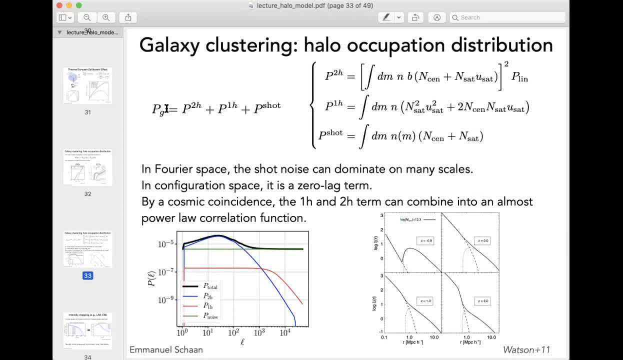 and now this HOD, you get the power spectrum of galaxies, And so you still have this two HELLO term that we talked about. You still have this one HELLO term, which is the shot noise of individual HELLOs, But now you have an additional term. 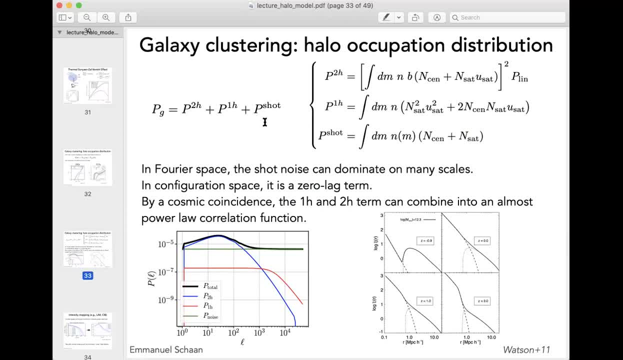 which is the shot noise of individual galaxies. So, as we've seen in the quick derivation, as soon as you have discrete objects- and before it was HELLOs- you end up with a HELLO shot noise. But now, not only do you have discrete HELLOs, 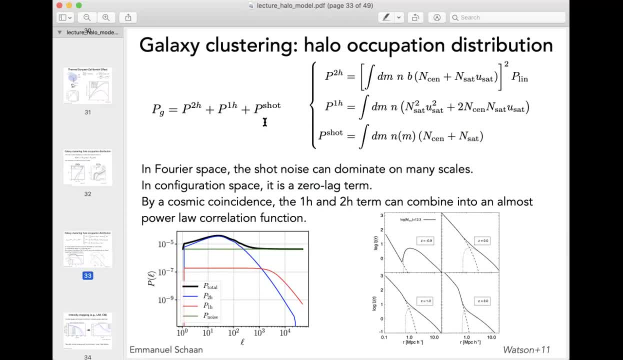 you have discrete galaxies that have those HELLOs And, as a result, you end up with a shot noise of galaxies. The expression for the two HELLO term looks very similar to what we had before, but now the profile is replaced by this: HOD. 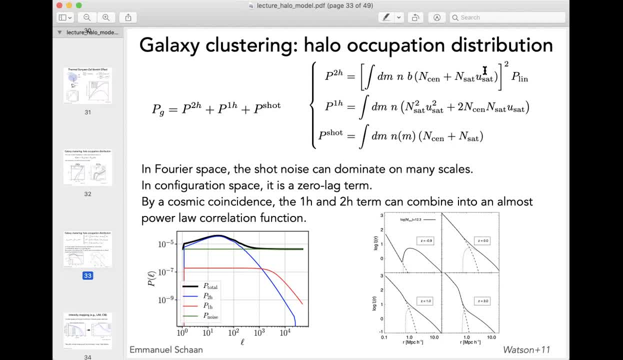 where USAT is a distribution of satellites, typically an FW. And again the one HELLO term looks similar in that it's only a single integral over mass. And finally you get this shot noise term And again you end up with a shot noise term. 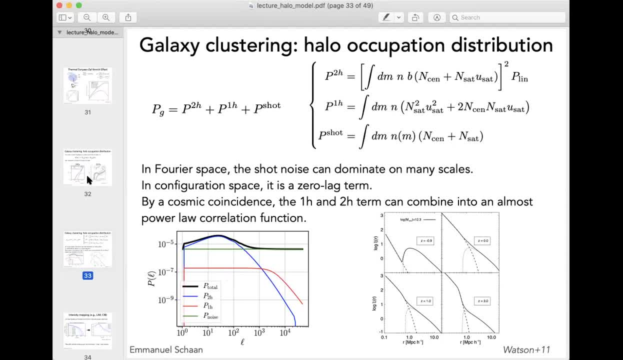 due to the discreteness of galaxies. To give you an idea of what that might look like for the HOD I showed you here, for luminous red galaxies, the power spectrum you might find is something like this: where again two HELLO here in blue. 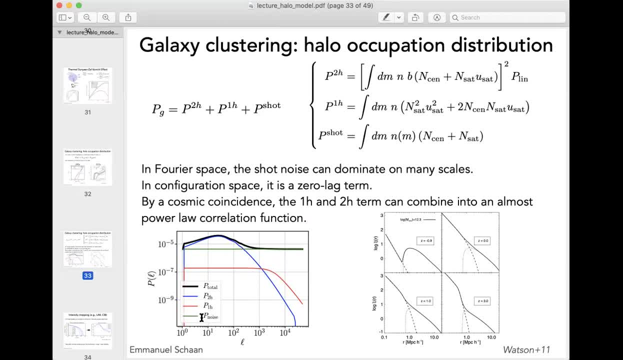 describes the clustering One: HELLO in red, the shot noise of HELLOs, And here this new shot noise term in green, is the number of galaxies that are in charge on a number of scales. And finally, I wanted to point out something 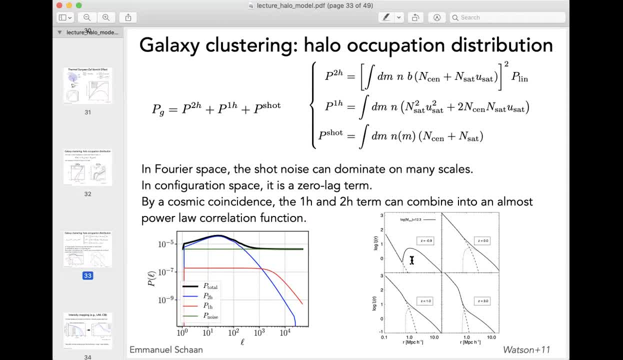 that's kind of interesting. You might find that a lot of times, when people measure the correlation function of galaxies, those galaxies are found to follow a parallel clustering, And the HELLO model helps to explain why that is. And so here, what you have is this correlation function. 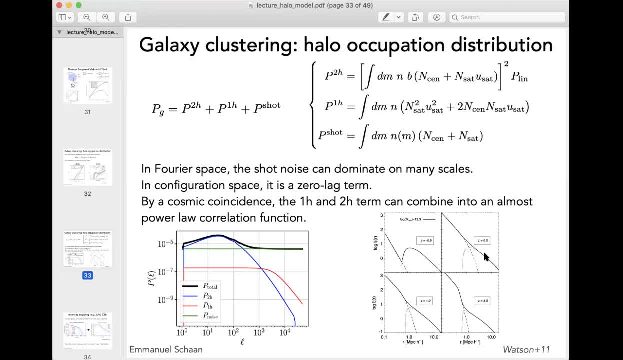 of galaxies as a function of separation, And in this panel, at redshift zero, you find that a conspiracy occurs between the one HELLO term on small scales and the two HELLO term on large scales, such that their sum looks almost like a parallel. 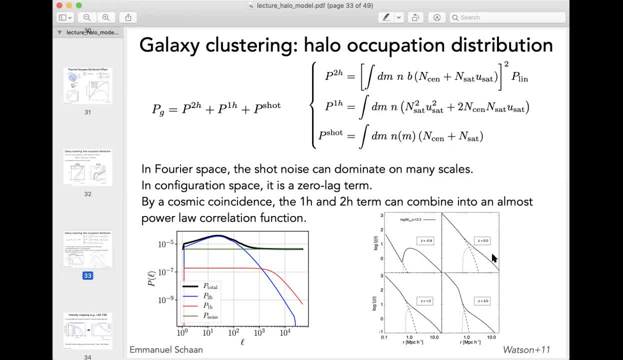 So this is an interesting fact that the HELLO model allows to explain, And because the one HELLO term and two HELLO terms scale differently with redshifts as you move to different redshifts, that coincidence is broken. Okay, So we've used the HELLO model. 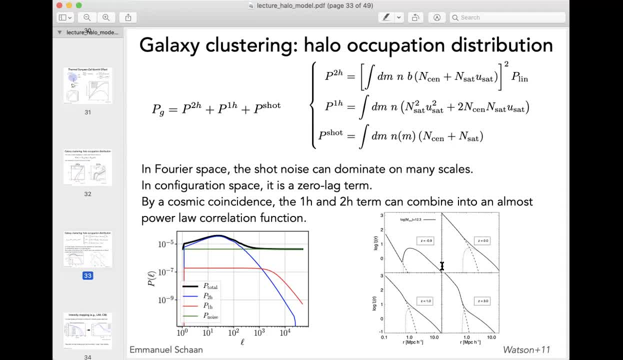 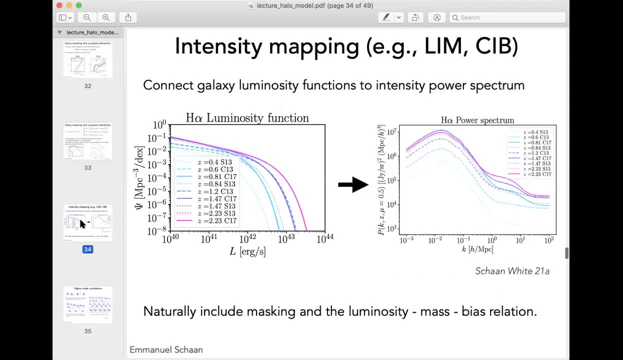 to predict the clustering of matter, lensing the Sunyev-Zeldovich effect: galaxy clustering. You can also use it for other observables, like intensity mapping, And intensity mapping is this way of looking at the large scale structure where, instead of identifying individual galaxies, 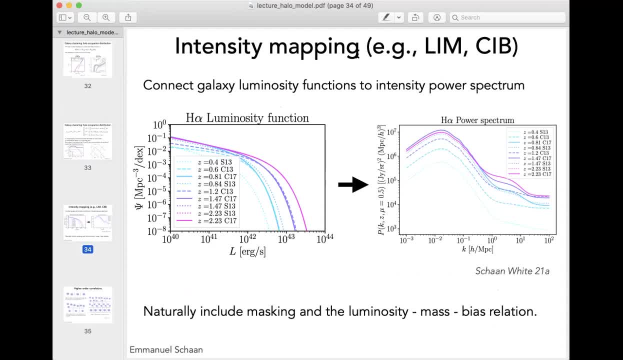 what you do is you measure the integrated emission from all the galaxies within your pixels, And so you do not require that you resolve individual galaxies. You're just measuring the blended total emission, And here too, the HELLO model is very useful. It lets you relate the galaxy luminosity functions. 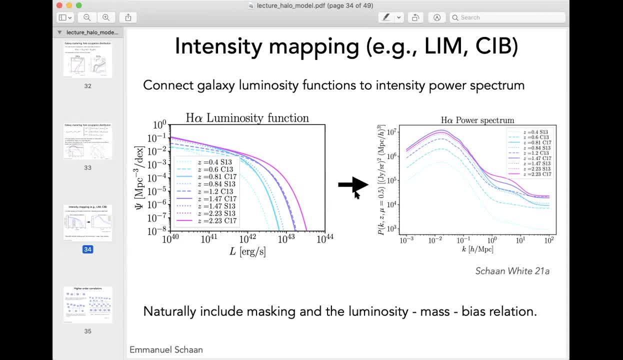 So how many galaxies are there of a given luminosity to their power spectrum? And so I won't enter into more details on this. I just wanted you to know that this is one very valid application of the HELLO model. Okay, So we've talked about power spectrum. 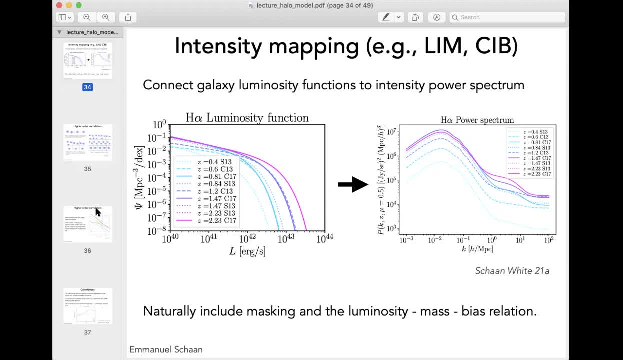 of many different observables. I'm going to talk about other things that the HELLO model allows you to predict, And so if there are any questions now, feel free to ask. So if not, I'll keep going and talk about higher order correlators. 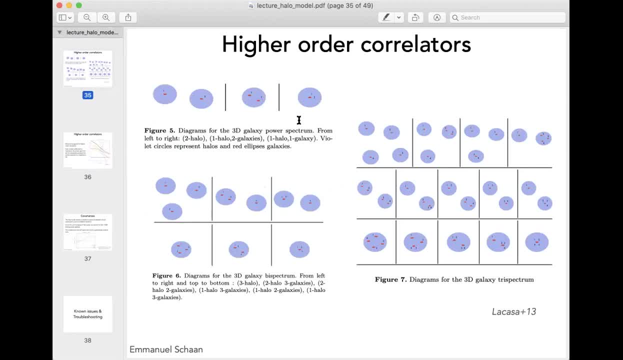 And I do not expect you to understand all of these cryptic schematics, But what I wanted to show is that the HELLO model lets you predict correlators of higher point than just two points, not just the power spectrum, but it also lets you predict the bispectrum. 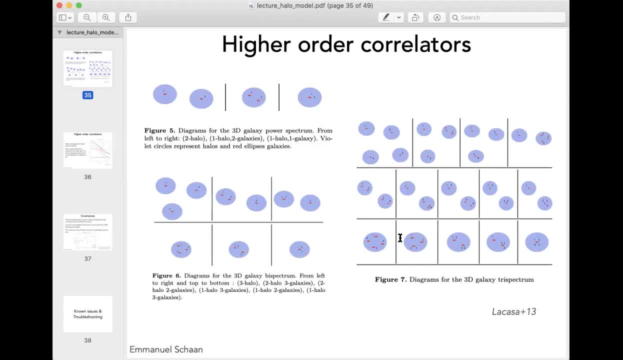 which is the three-point function, and the trispectrum, which is the four-point function, And the schematics here describe the various terms. we talked about The one HELLO term where the two points of interest, one and two, lie in two different HELLOs. 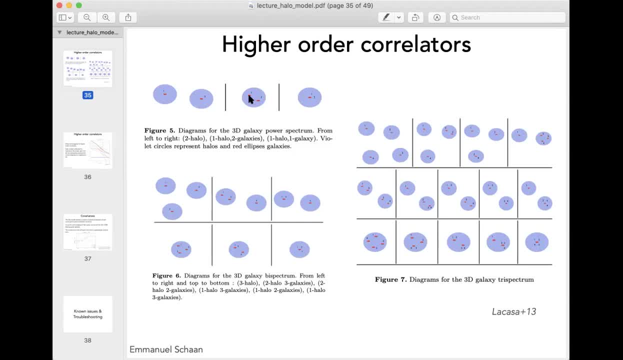 The one HELLO term where the two points or the two galaxies of interest are in the same HELLO, And the galaxy shot noise term where we're looking twice at the same galaxy And the same kind of combinatorics occurs in higher point functions. 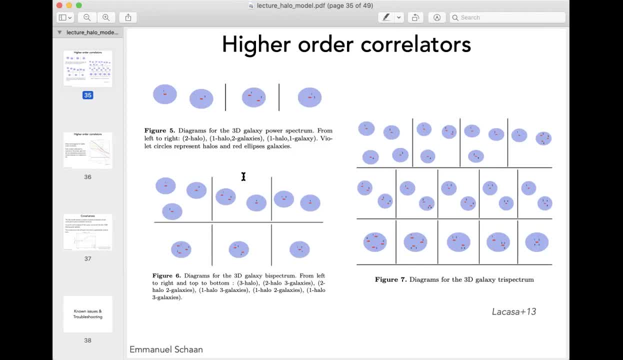 where now, instead of having a two HELLO, one HELLO term and a shot noise, you might have a three HELLO, various two HELLO terms, various one HELLO terms and one shot noise, And so the HELLO model. 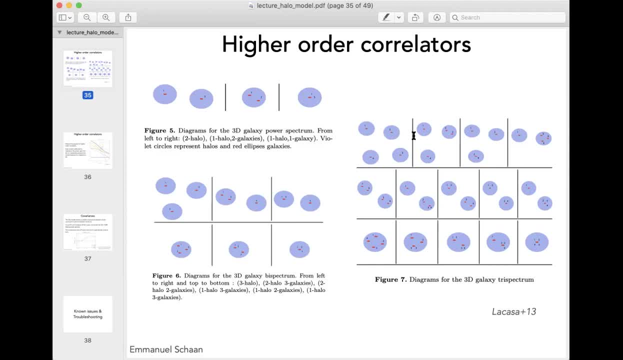 lets you go to higher order and split the high point function, for example the trispectrum, as a sum of many four HELLO, three HELLO, two HELLO, et cetera terms, And so that's sort of a nice property. 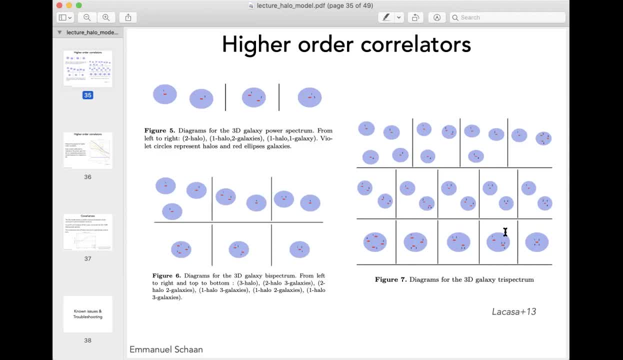 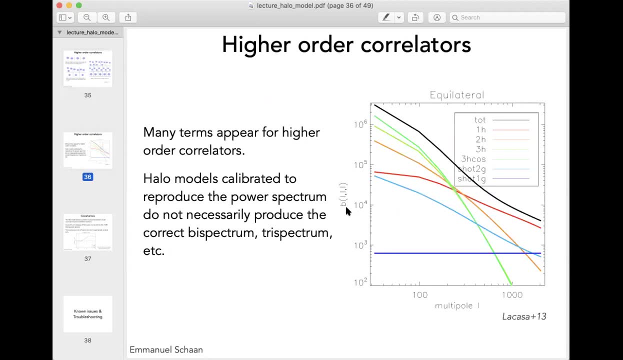 of the HELLO model is that it lets you go to higher point function than you would otherwise be able to do, And, to give you an example, this is some of the various terms that go into the bispectrum of galaxy as a function of scale. 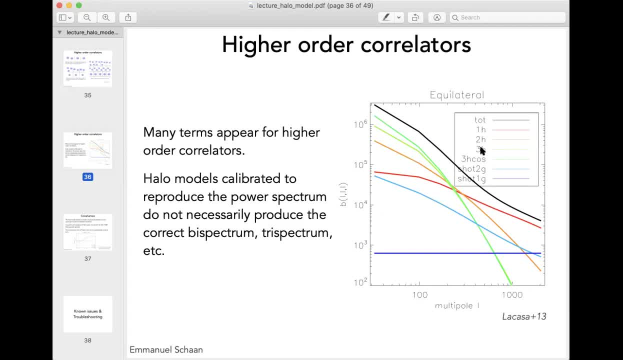 in a specific configuration, And so what you should see is it gets complicated and that there are many, many terms that appear more and more as you go to higher and higher order. And also, I would encourage you to always be cautious when looking at higher order correlators. 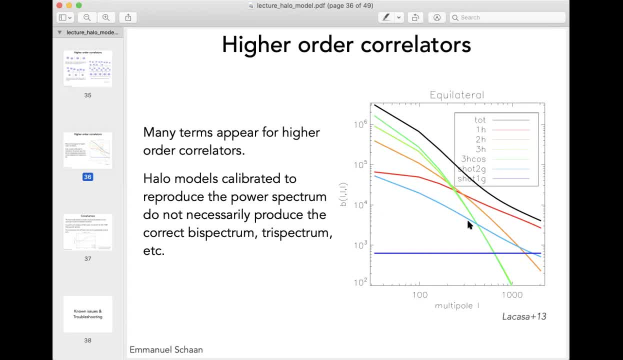 from the HELLO model, because most HELLO models have been calibrated to produce the right power spectrum, but not necessarily to produce the right higher point function. So this is always something to keep in mind, but it's still a nice property of the HELLO model. 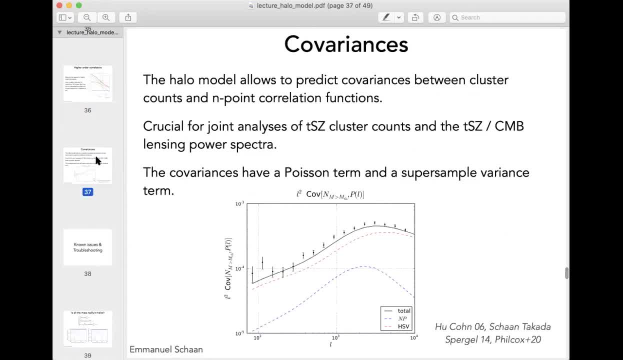 And finally, and related to being able to predict higher point function, another thing that the HELLO model predicts is covariances, For example, covariance between power spectrum at one scale and the power spectrum at another scale, or covariance between the power spectrum. 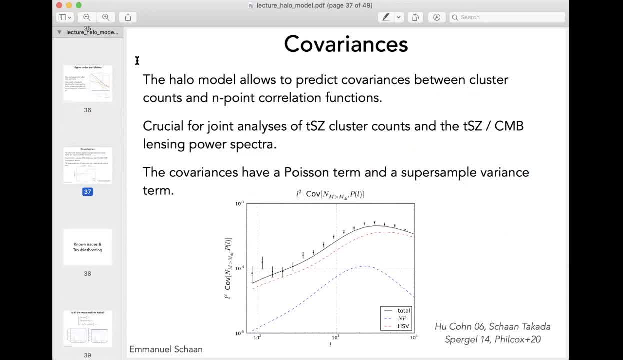 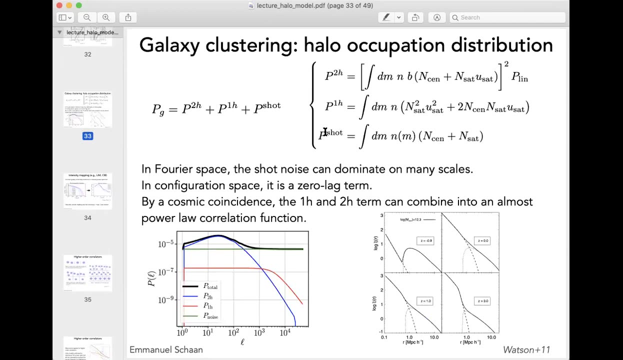 and the bispectrum or, importantly, the correlation between your endpoint function and cluster counts. And to give you an idea of how this works intuitively, it's fairly simple. Your power spectrum, or your endpoint function in the HELLO model, is a sum over the number of HELLOs. 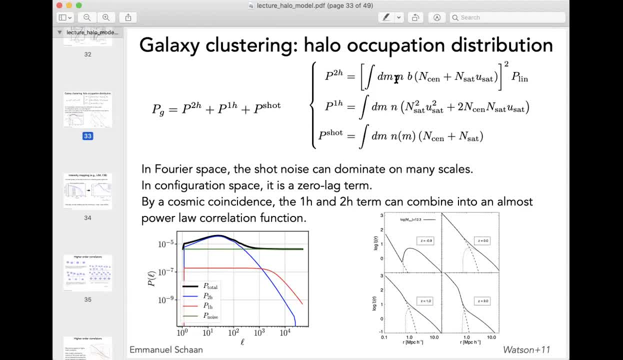 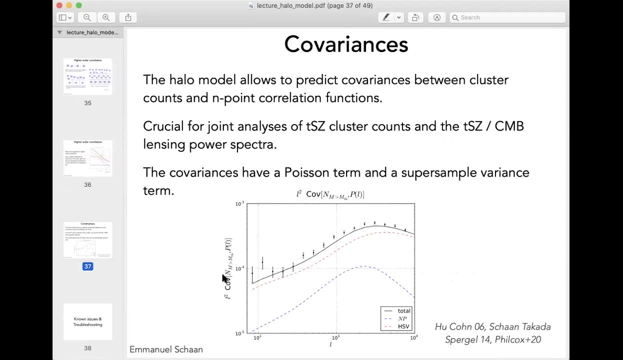 So if you now know which HELLOs hosts clusters, you can clearly see what the correlation is between those clusters and your power spectrum or your endpoint function. And so this plot here is just an example of a covariance between the number of clusters and the lensing power spectrum. 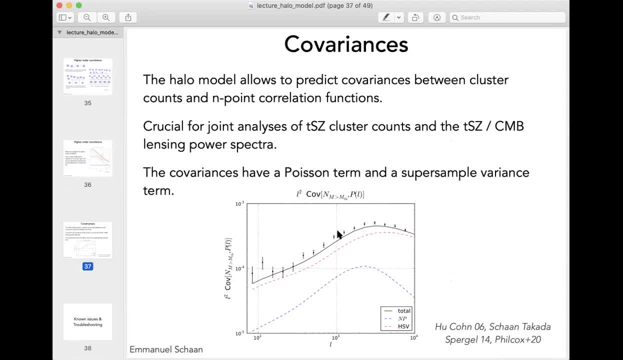 And you can do these calculations in the HELLO model for any number of observables, And so that's in my mind. one of the key values of the HELLO model is this covariance with the number of clusters. That's otherwise quite hard to predict. 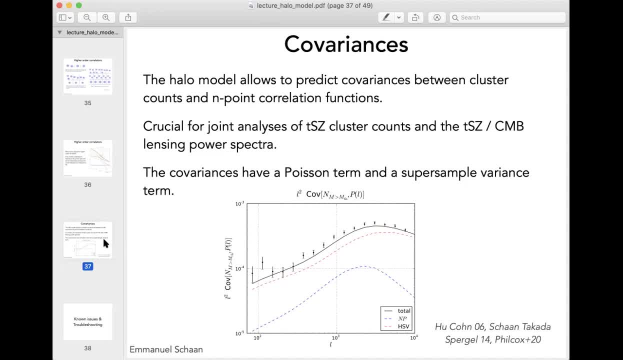 So I think I'll stop there for the various applications of the HELLO model. So we've talked about power spectrum of very many quantities. We've talked about bispectrum, trispectrum, covariances of power spectrum and number counts. So if you ever need to compute, 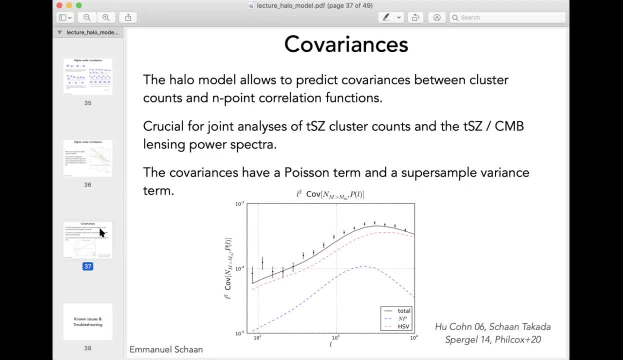 any such thing, you might want to think about the HELLO model as a good way to estimate it. And now in the last few minutes, I'll briefly go over some of the known issues and limitations of the HELLO model And, depending 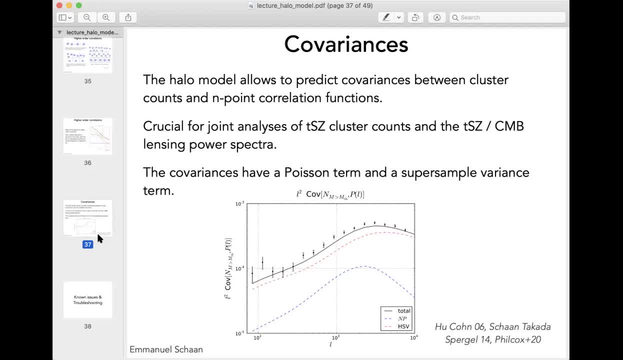 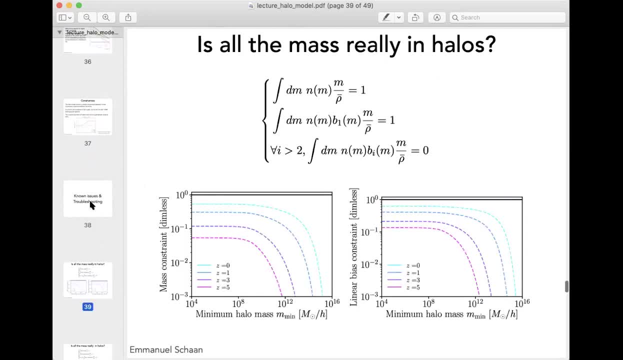 on your application. these may or may not be a showstopper, But regardless, it's good for you to be aware of them. So the first known issue that I want to talk about is the one that Noah raised earlier in relation with those. 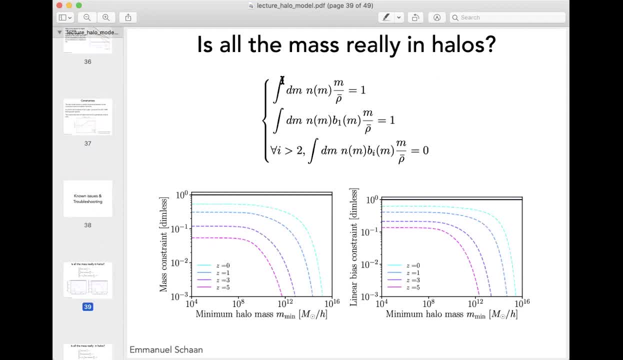 consistency relations. So the first one, if you remember, was this idea that all of the mass is in HELLOs, And so if I sum all of the HELLOs in the universe, weighted by their mass, I should get the total matter. density field. 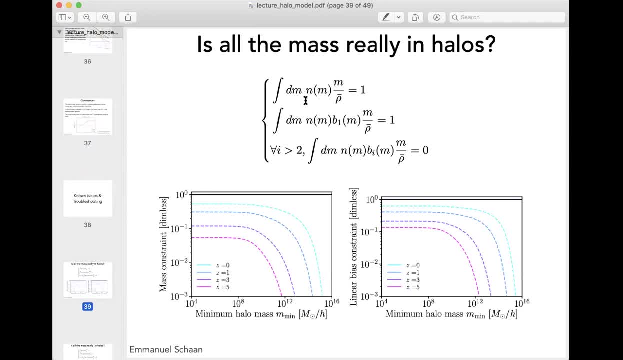 in the universe. Now, in practice, the HELLO mass function is only measured from simulations down to a certain minimum mass under which you don't resolve HELLOs. And so when you compute this integral as a function of the minimum mass, so when you compute, 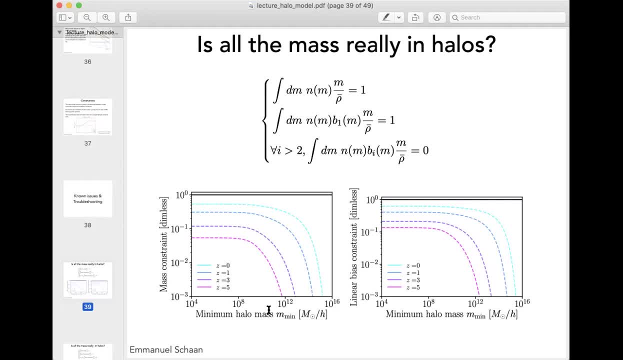 this integral here as a function of the minimum mass. as the minimum mass goes down and down and down, you get closer and closer to unity And you would hope, for example at redshift zero, that at some point you would reach unity. 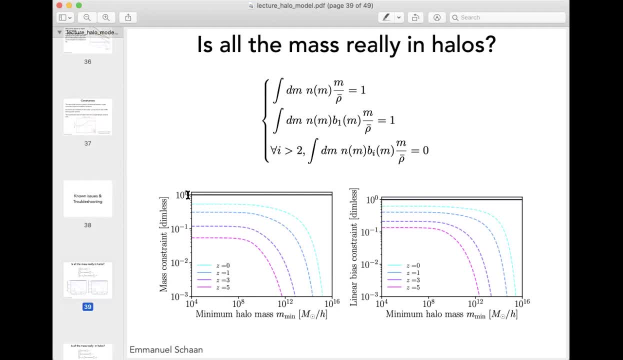 But with a lot of HELLO mass function fitting functions, you find that that's not the case. So, for example, at redshift zero, even when you go to incredibly small HELLO masses, you find that only about 0.5. 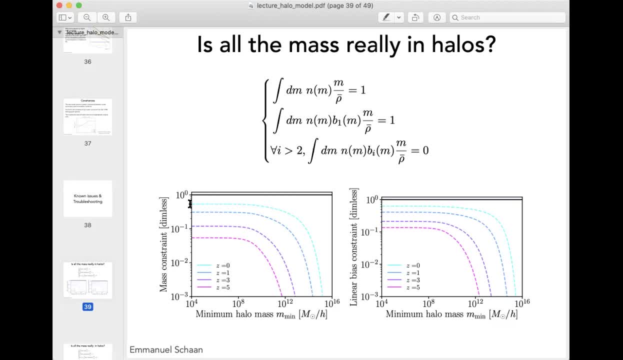 or 50% of the mass is actually inside of your HELLOs. The same issue occurs for the second consistency relation that involves the bias, where when you compute that integral and you hope to get unity, when you go down and down in the minimum mass. 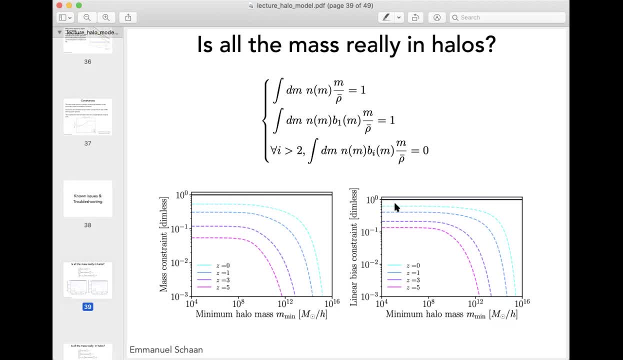 for example, at redshift zero, you find that you don't quite reach unity. So, depending on the observable you care about, this may or may not be a problem. If you care about the matter- power spectrum- this is a problem. 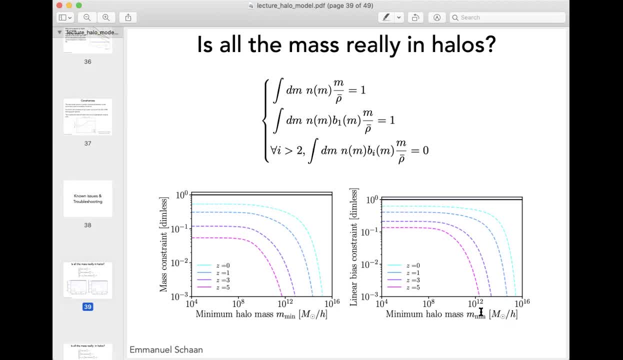 If you care about observables where only the highest mass contributes, for example, if your galaxies only live in massive HELLOs or, for example, the thermal IZ, which only cares about massive clusters, then it's not an issue. 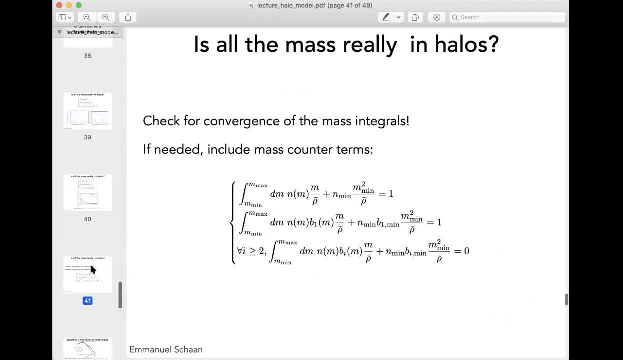 But in all cases, if you use a HELLO model, you should always check for the convergence of your mass integrals And if those integrals do not converge because not all the masses in your HELLOs- a typical fix that people use. 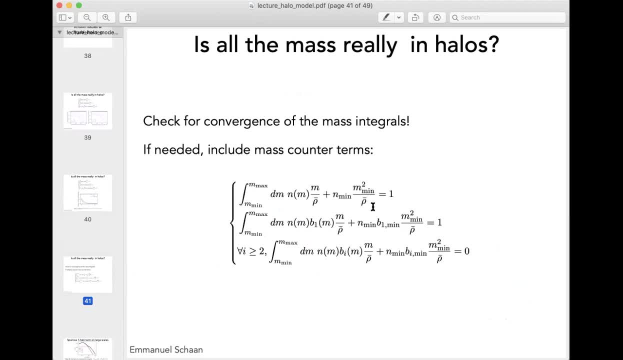 is to add these counter terms for the low masses, And so I won't say too much more about this, but this is a very simple fix that allows you to satisfy the consistency relations. So that's one of the key issues that we need. 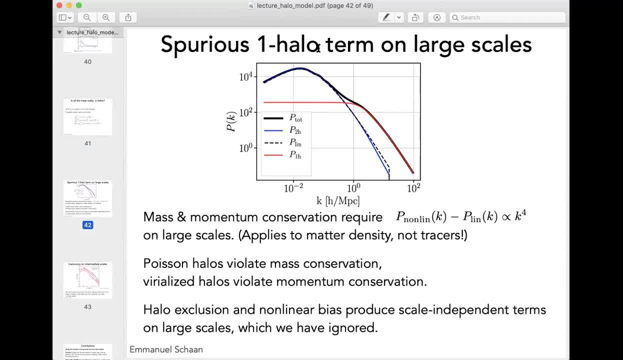 to consider. The second one is this question of the one HELLO term on large scales. So, if you remember, this is the matter: power spectrum as a function of scale. And, as I explained, this one HELLO term is what makes the power spectrum. 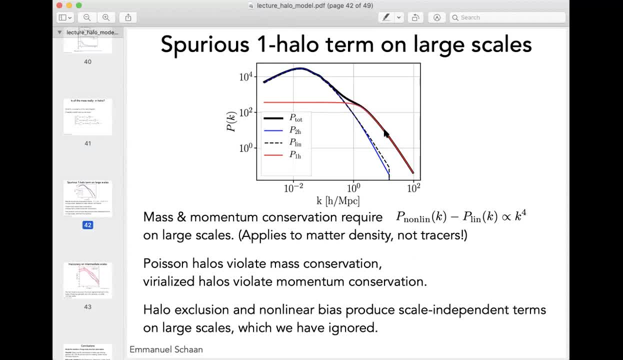 differ from the linear power spectrum mostly, And it's a correction that matters on small scales. But what's not shown on this plot is that this one HELLO term is constant with k, So it stays flat forever As k goes to zero. 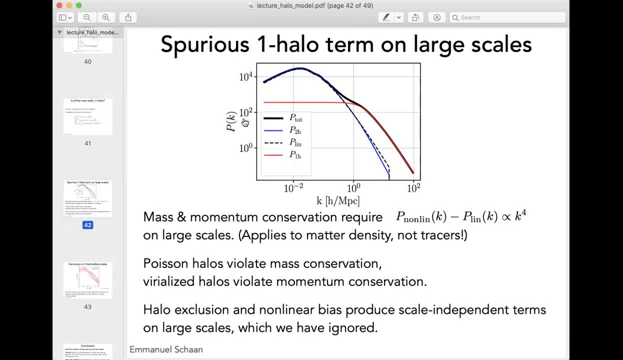 And so if you go on large enough scales, your HELLO model power spectrum is dominated by the one HELLO term, And this is an unphysical effect. The reason we know this is unphysical is mass and momentum conservation. you can show. 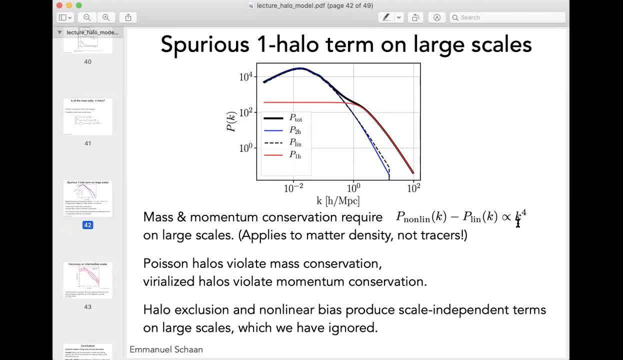 that they require any deviation from the linear power spectrum to go down at loci, And so this one HELLO term is forbidden by mass and momentum conservation. The reason it appears here is because the HELLO model, the way we phrased, 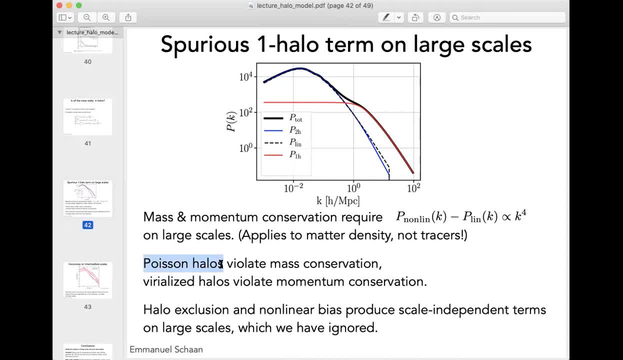 it violates those conservations. One, if you remember, we assume that the number density of HELLO is poisson, meaning rare, independent events, And this violates mass conservation, because if you want to conserve mass and you form one more HELLO here. 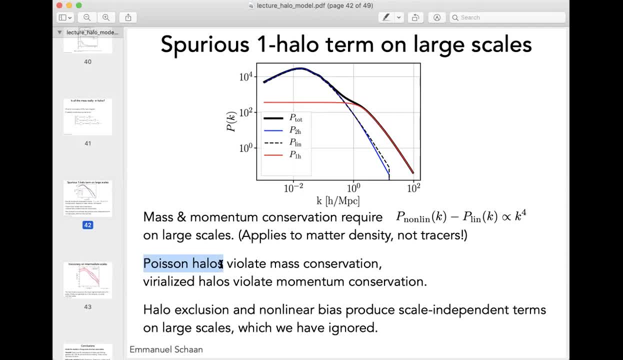 the number density of HELLO left and the number density of HELLO right. you assume things are independent. poisson approximation: you will violate mass conservation And second our HELLO profiles. the NFW profiles assume basically that the matter is virulized. 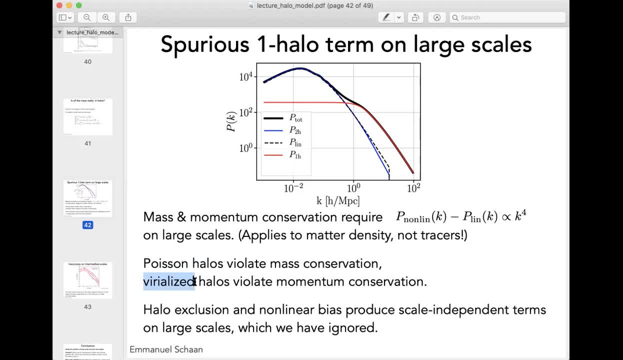 instead of HELLOs. I won't say too much about this, but basically this says that there's no memory of the initial velocities of those particles, And so this violates momentum conservation. So you do not care about any of these issues. 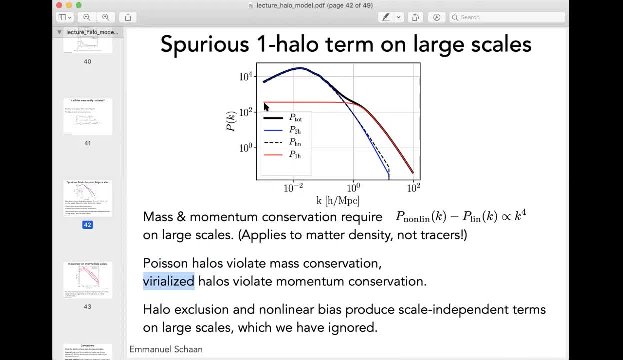 But if you care about the very larger scales, for example, if you care about non-Gaussianity, then you may want to truncate your one HELLO term to avoid this pervious contribution. So that's the second biggest issue with the HELLO model. 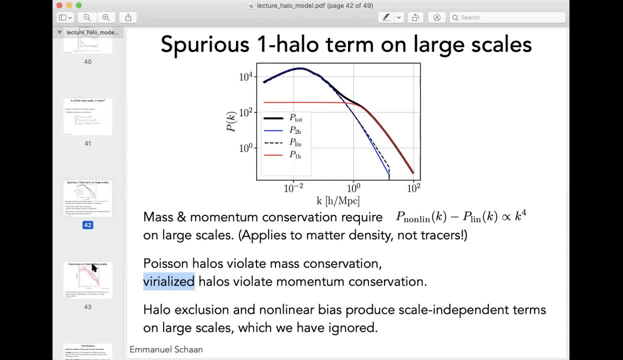 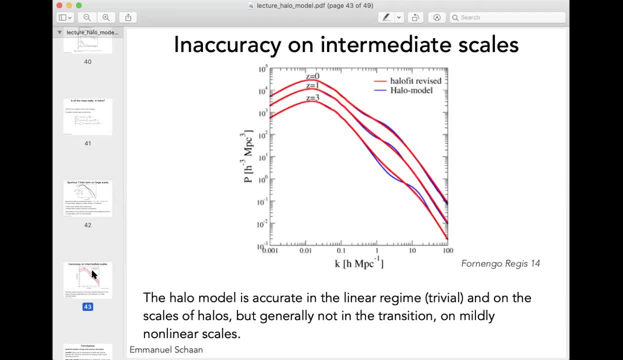 And again, for most applications where you care about small scales, it's not a big deal, but it's something that you should always be aware of. And finally, before we finish, the last HELLO model is its accuracy on intermediate scales. 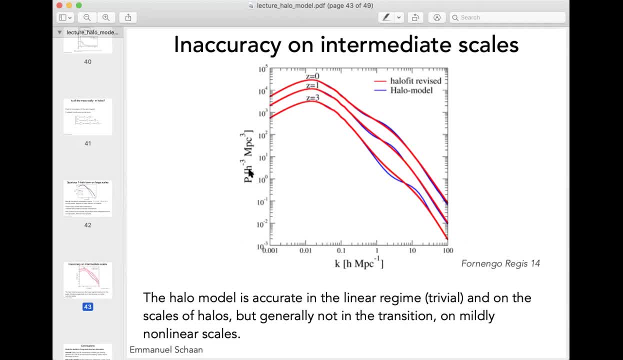 So what you see here is again the matter-power spectrum as a function of scale. Blue is the HELLO model prediction And red is HELLO fit, which is a fitting function to simulations, And what you might see is that the fit is very 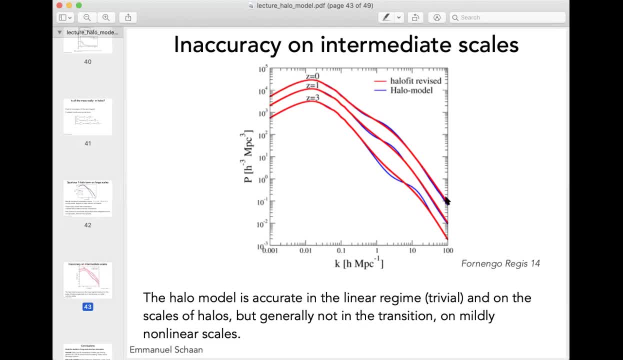 the two curves match very well on large scales where linear theory is valid, And they match quite well on very small scales where you are indeed in the middle. but the match is not excellent on those intermediate, mildly nonlinear scales. And again this has to do. 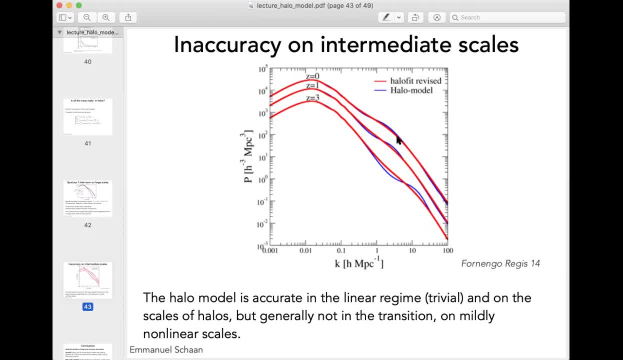 with our assumptions of Poisson HELLOs and of linear bias. And so if you care about high precision on mildly nonlinear scales for matter, the HELLO model may not be the tool for you, But if instead, you care about the very small scales, 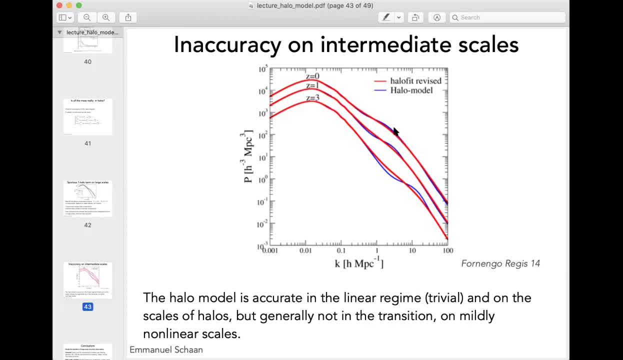 the highly nonlinear regime and, for example, that's often the case for other observables, like the HELLO model. the HELLO model is a good choice. Okay, So these were the three known issues of the HELLO model that I wanted. 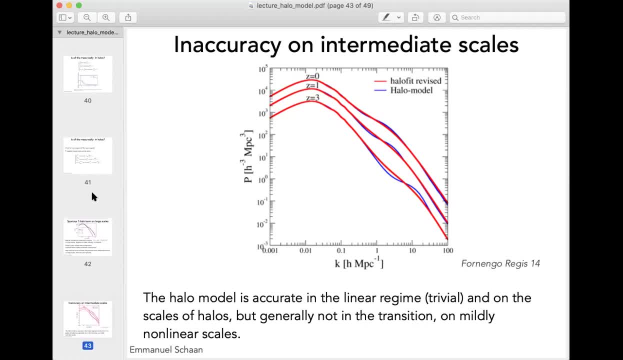 to point out So: one, that all the mass is not always found inside of your HELLOs. Two, the spurious one HELLO term on large scales. And three, there's not great accuracy on intermediate scales, And so. 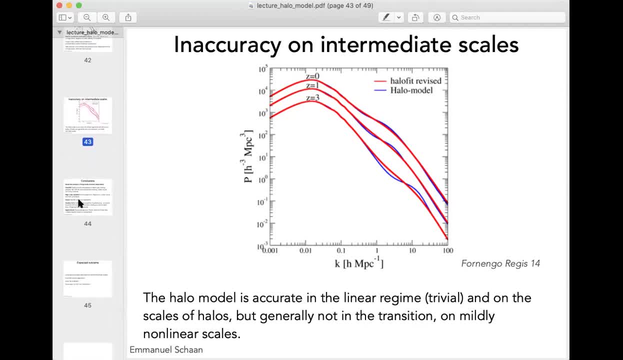 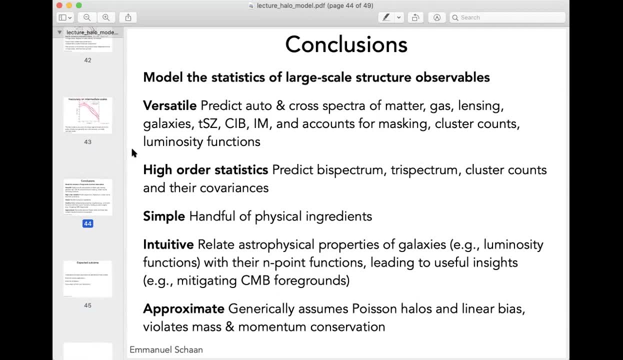 I'll just conclude with the things that I think are important to consider. I started with so one. hopefully you have some understanding now of what the HELLO model is and how it lets you model the statistics of various large-scale structure observables. 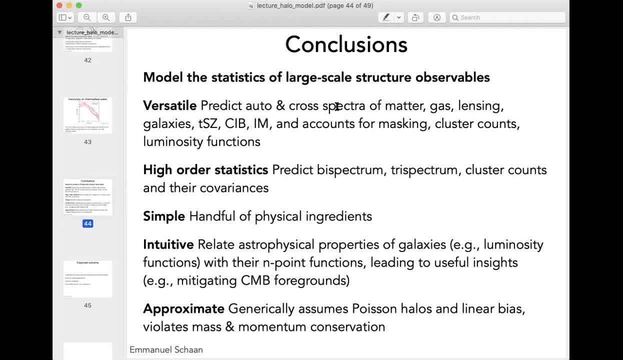 I've tried to show you how it's very versatile in predicting power spectra of many different observables, but also quantities like number counts of clusters, number counts of galaxy, galaxy luminosity functions, The fact that the HELLO model is very simple. 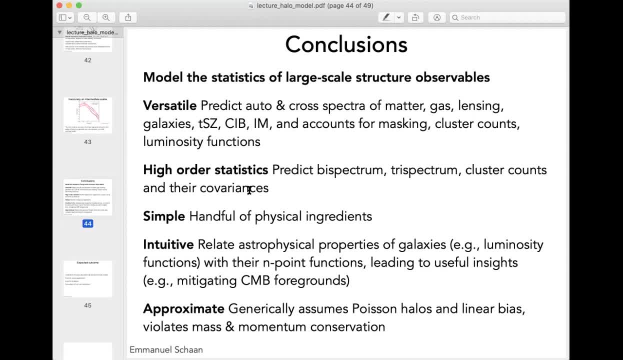 only a handful of physical ingredients, if you remember HELLO mass function, HELLO bias, HELLO profile, and that's it. And the fact that it can give you some intuition as to why the power spectrum looks the way it is, by relating 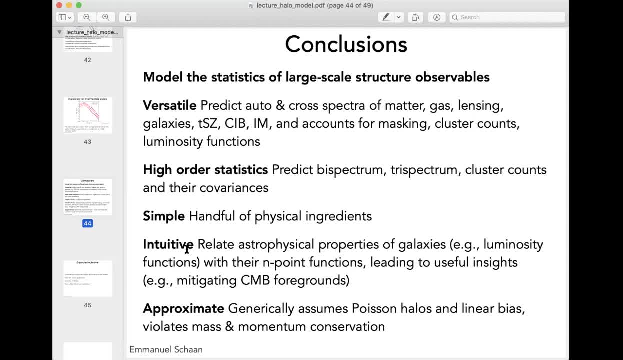 properties of galaxies, for example, luminosity function with their endpoint correlators, And the other thing that I would like to highlight is that the HELLO model can be used in many different ways. And finally, we talked about the various approximations that go. 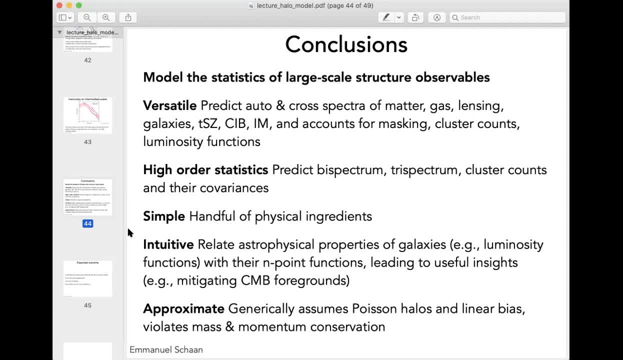 in the HELLO model and their limitations. So things like assuming Poisson HELLOs and linear bias which violates mass and momentum conservation, And so that's the end, which would be a really good starting point if you want to learn more about any. 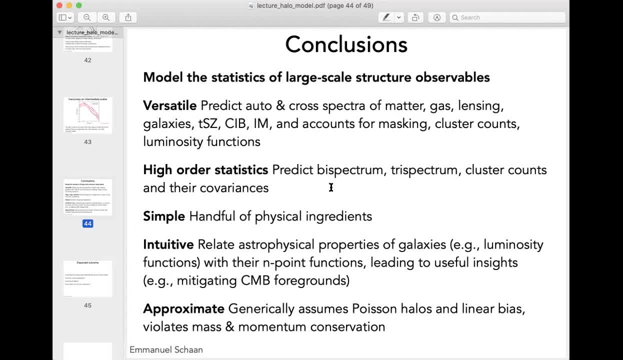 of this. So this is the end, And if there's any questions, please feel free to ask now. Are there modifications to the HELLO model that you know of that? try and change the statistics of how HELLOs matter in a way that conserves. 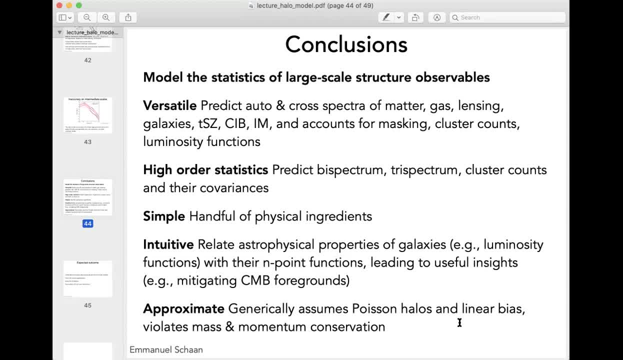 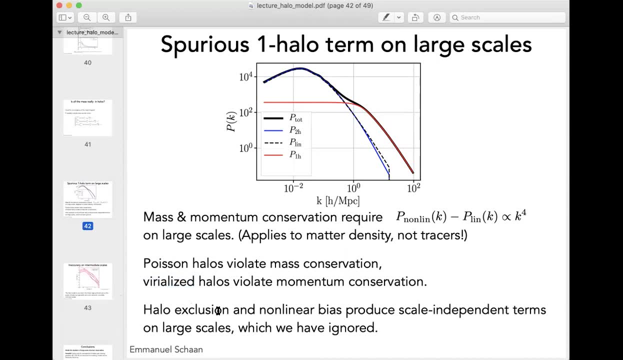 mass Right. Yes, So it turns out there are, And so right. So the two main limitations that cause this spurious one HELLO term on large scales here are this Poisson assumption and this assumption of linear bias. And it turns. 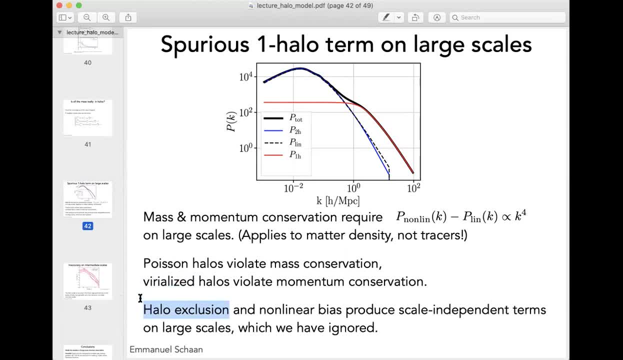 out something called HELLO exclusion. the fact that the space is inside of a HELLO cannot be inside of an other HELLO because HELLOs are defined to be non-overlapping. This HELLO exclusion effect kind of like hard sphere model in StatMech. 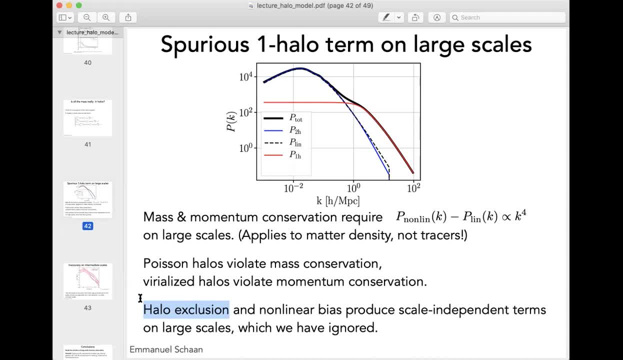 means that it breaks this Poisson assumption and it kills part of this. one HELLO term on large scales And non-linear bias. so, for example, terms like the b2 squared also causes a scale independent term in the power spectrum, And so 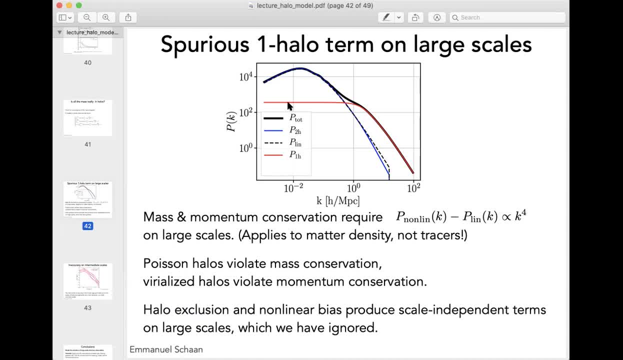 if you can self-consistently include all these effects, you would find that this one HELLO term go to zero. And so some of these, some of the papers I listed here, do some of this, And so, if you're interested, 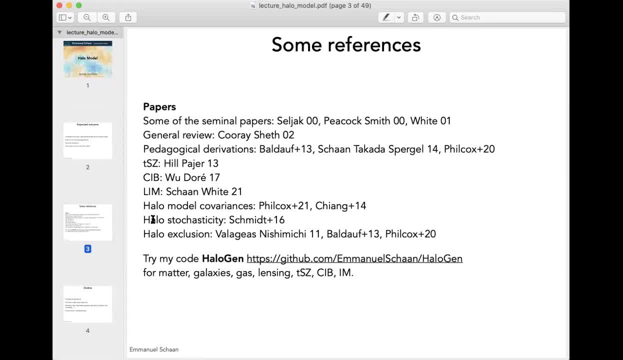 in issues of HELLO exclusion and HELLO stochasticity or deviations from Poisson statistics. this is also a very good reference. And are these just with antibody simulations or are these analytical Here? most of these papers here are analytical modeling that basically try to include.